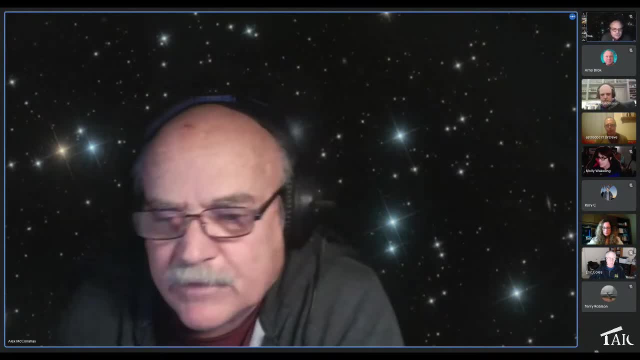 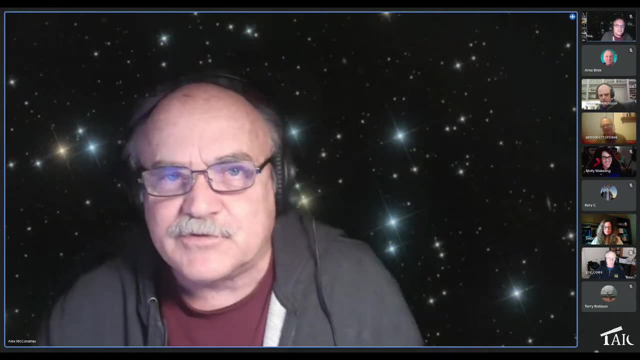 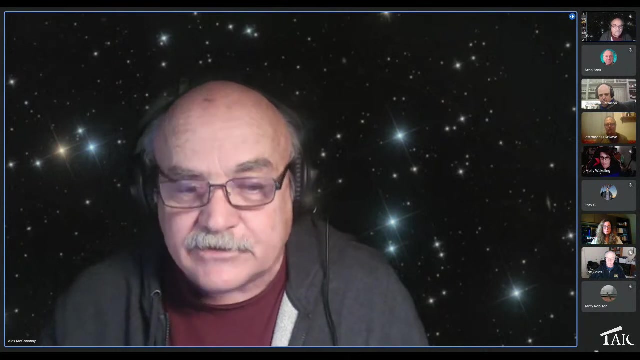 And we ask questions and we find out what's happening in astroimaging, And tonight in particular, Dr Dave Doctor will be joining us from Las Cruces, New Mexico. He's here to tell us about high-res spectroscopy And we're looking forward to that show. find out some things we can do as astroimagers- besides take pretty pictures. 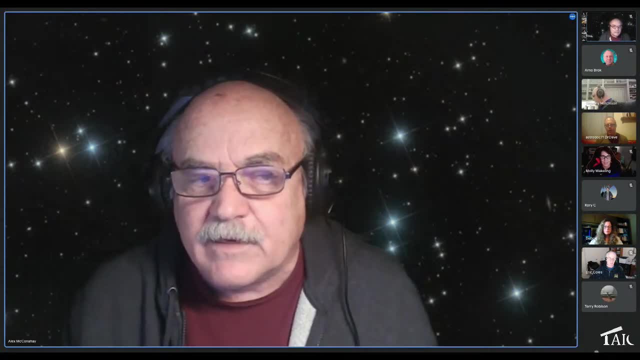 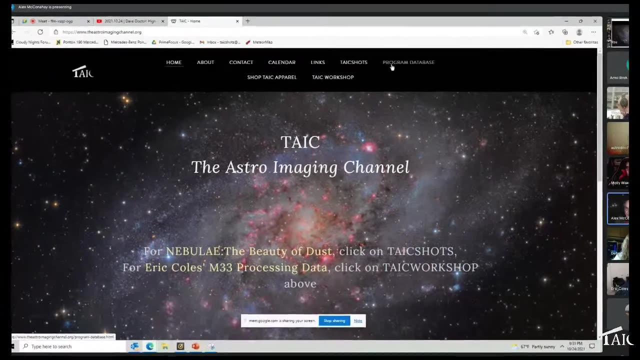 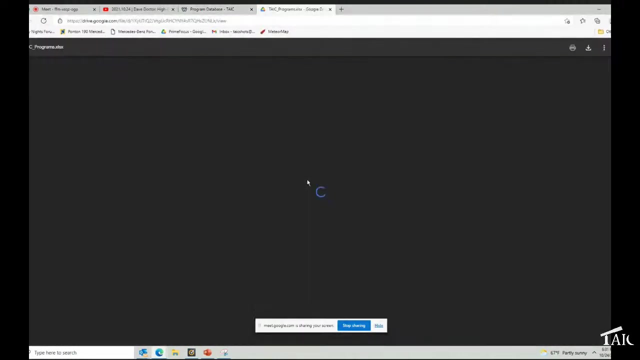 where we kind of focus a lot on that kind of stuff. So let me take you over to the website for a minute, because I got to. I want to remind you of some things. The first place: I want to remind you that we've got a big spreadsheet out there with all our programs in it. 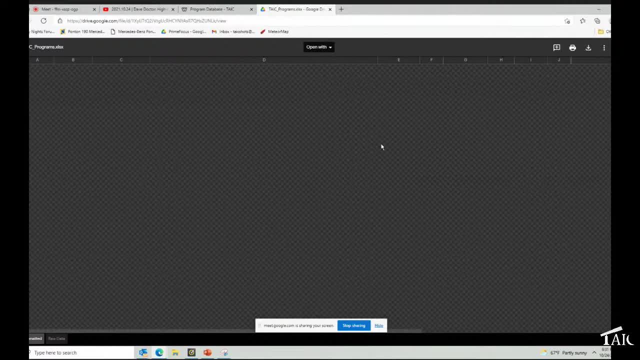 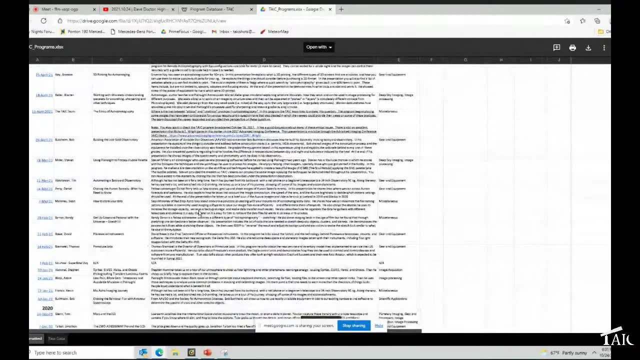 And we've got a couple of people working really hard to put information into this spreadsheet. You can search any time you want and find whatever it is you like And it's a description of programs and all that we've had And we've gotten like a couple of years worth done now. 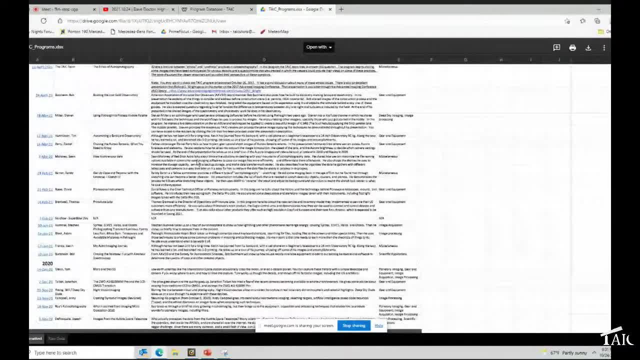 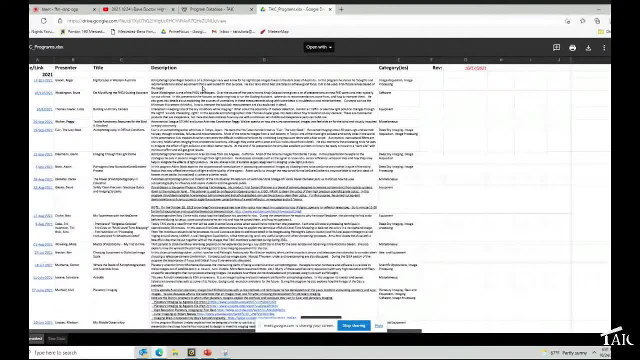 And we're coming up on what? eight years or seven years, Seven to four years- And it's been hard to get it all caught up. But Wanda has gotten us caught up and she's starting to get some other people to help. 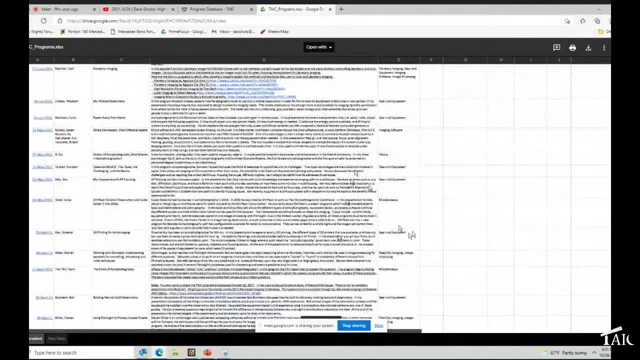 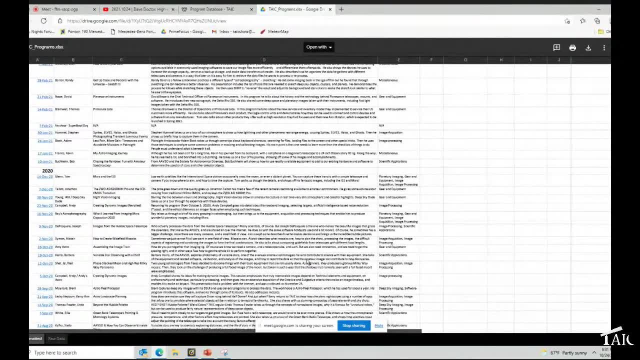 If you'd like to help on this project, you can see that down towards the end. we've got lots of them down towards the end that aren't done yet. I'd also like to congratulate Wanda, who didn't join us in the room tonight because she's moving around the country. 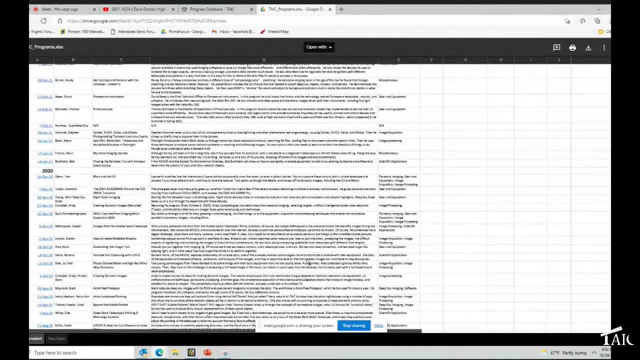 But she's with us. I think, Wanda, you got a letter to the editor in Sky Intel Magazine, if I'm not mistaken, So congratulations on that. Now, where were we? Oh yeah, We were going to go. told you about that. 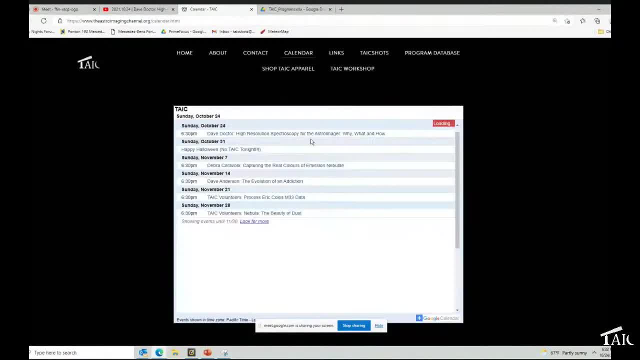 And I want to tell you about the calendar, because tonight's Dave, and then next week we won't see you because we have to be jumping up And I would be. it's my time. you know, 630 at night here in California. 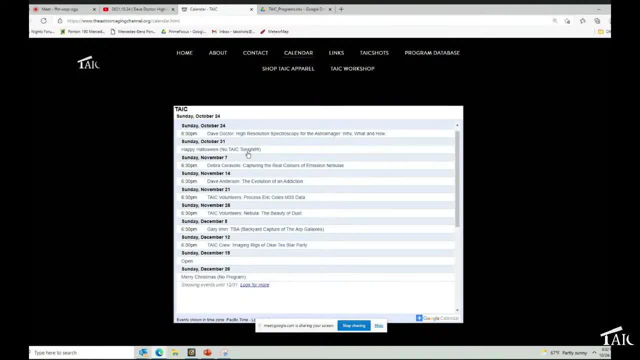 I'd be out there feeding the ghouls and the skeletons and stuff like that. So I'm not going to be jumping up, So I'm not going to be able to be here. So there's not going to be a TAIC show next week. 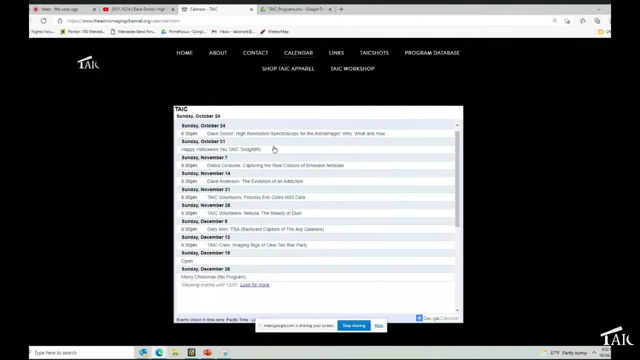 So you'll all be on Sugar Rush anyway and you probably wouldn't be contributing to the program. So we're just going to skip next week. But Deborah Cerebolo is joining us And Deborah's always a pleasure to have around. 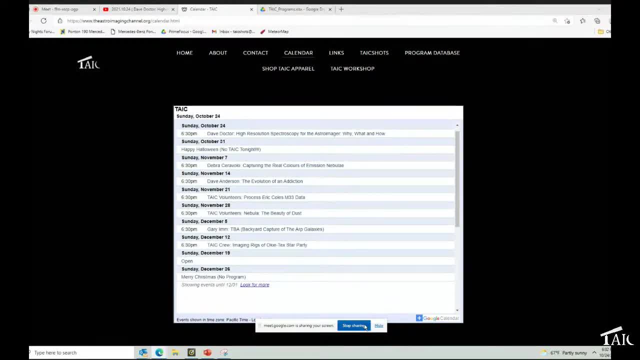 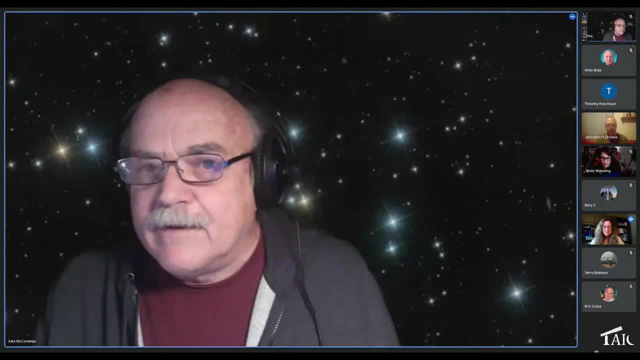 I'm going to stop sharing because Deborah's here and she wanted to tell you just a little bit about what's happening with that program. Stop sharing, Deborah. come on in Sure, Can you hear me okay? Yep, All fine. 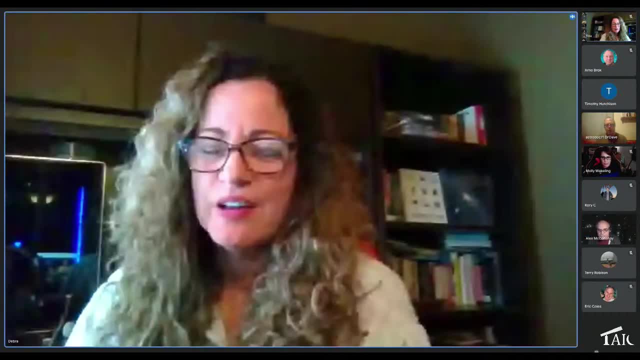 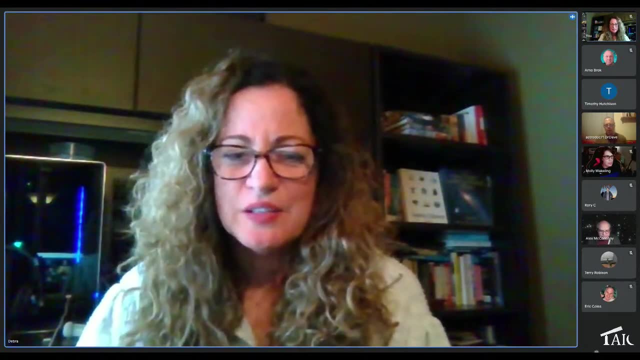 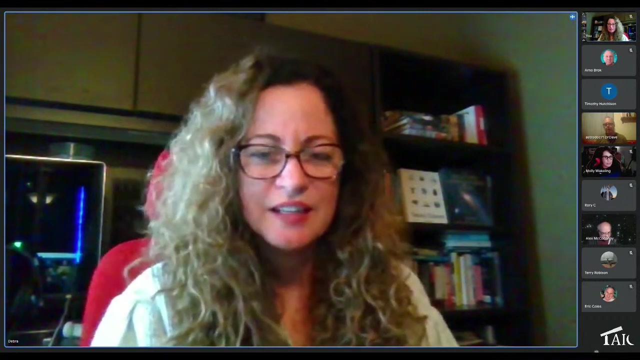 Okay, Yeah, I'm going to be talking about how I acquire my narrowband images for emission nebulae and how I process them And basically the bottom line that you know, the results I got from all the testing that I did with different filters- is actually quite surprising even to me. 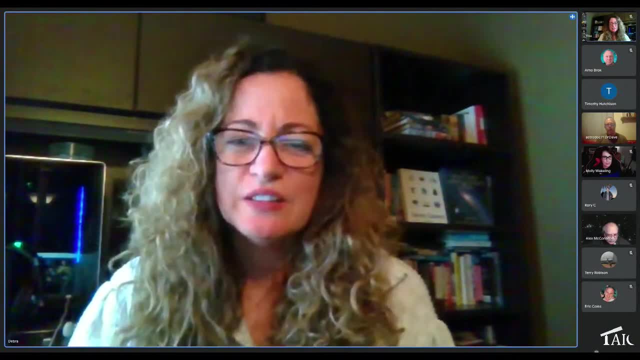 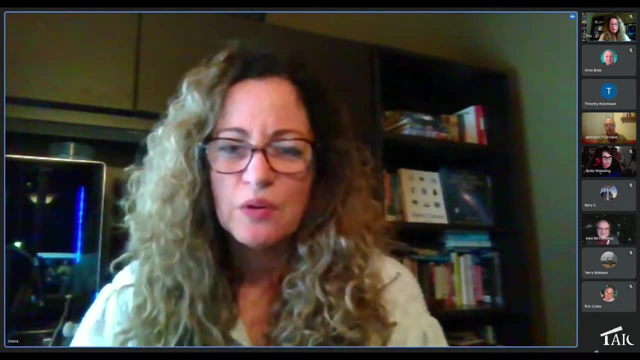 But the result is that basically forget RGB, Use only narrowband, But I use other filters like hydrogen beta. that makes all the difference in the world, So tune in to find out more about that. Okay, Thank you very much, Deborah. 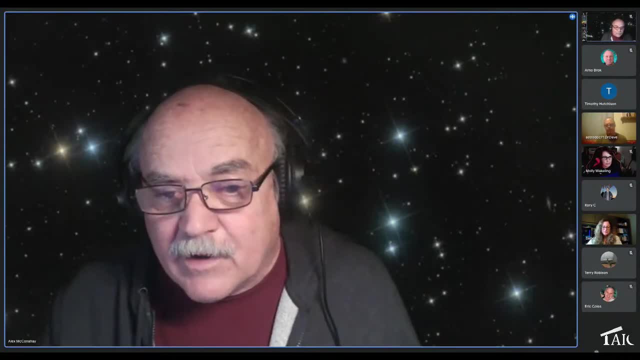 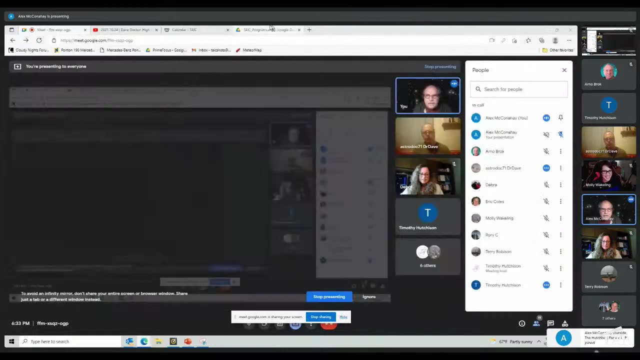 We'll be seeing you Now- that's in a couple of weeks, remember, because we're going to be gobbling next week, Not gobbling Thanksgiving, That's in a different time- coming up, And then where were we? Then we've got some other programs. 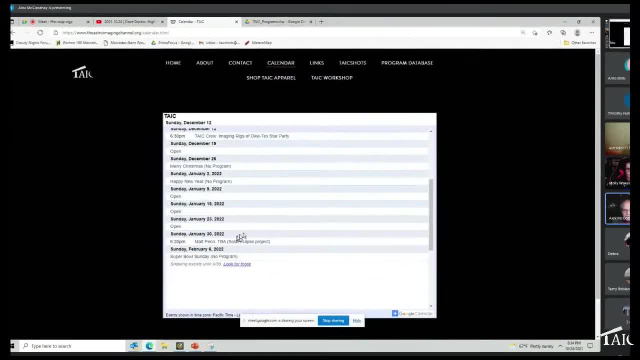 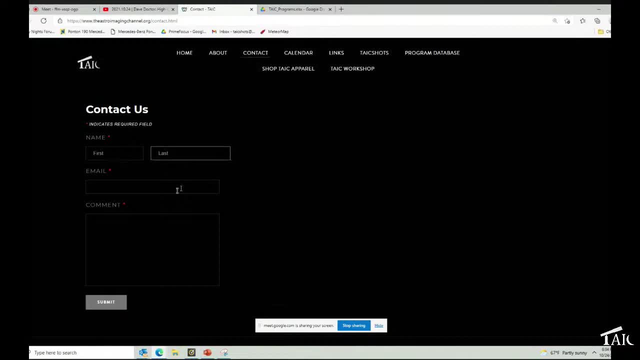 And then we start having emptinesses And we've got to fill those empties And we need your help doing that. So please hit the contact button. Okay, Tell us who you are, what you want to talk about And join the fun. 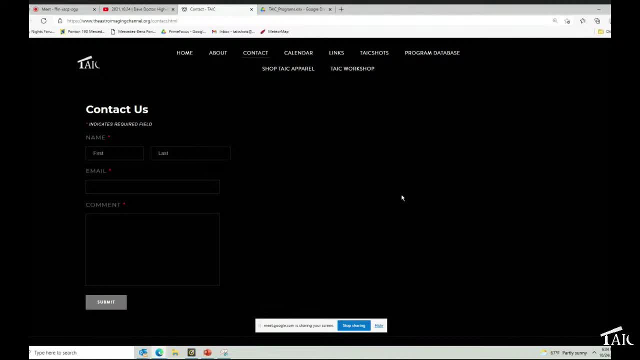 You know, I mean, it's good to have people that are really, really, really, you know, really professional, high class, But mostly we want people that are enthusiastic about astroimaging and are willing to join us. Okay, So please come along with that. 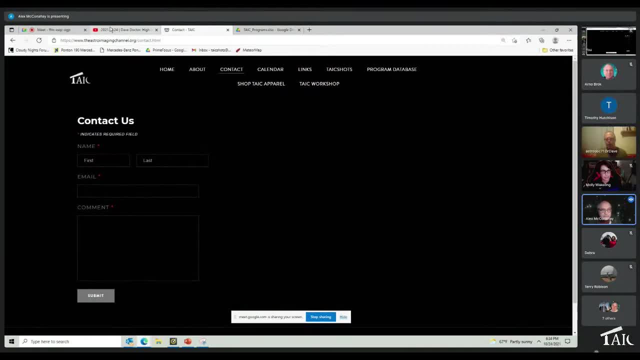 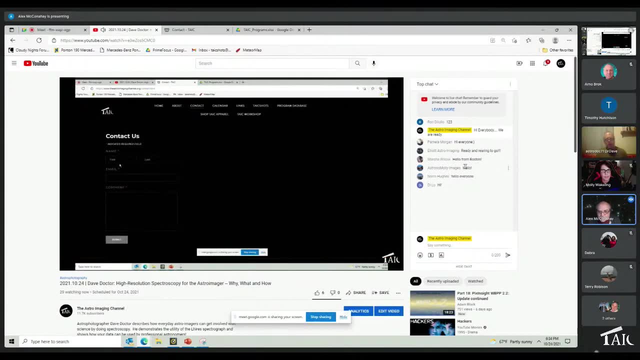 And, if I'm not mistaken, let's see Where is There it is. Oh, I have to turn myself off. There we go. You've got notice over here. You've got an area to ask questions about spectroscopy tonight, if you've got anything that you want to know. 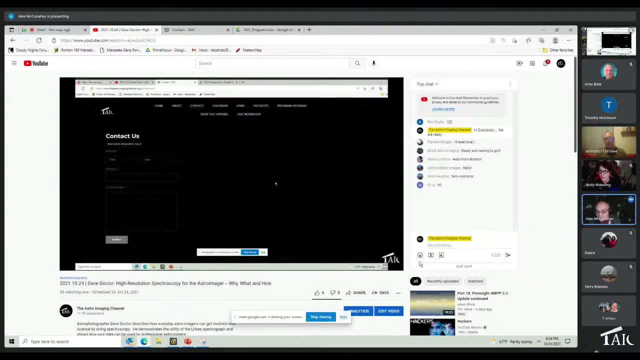 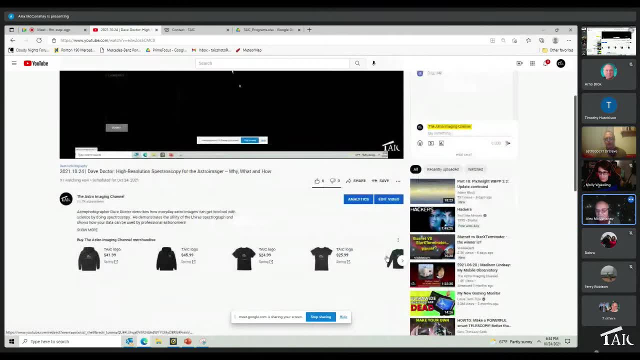 You've got some buttons You can donate And you can, you know, put in some emoticons. You can do all that kind of stuff. You can buy swag for Christmas presents, really cool Christmas presents. So there's a lot. 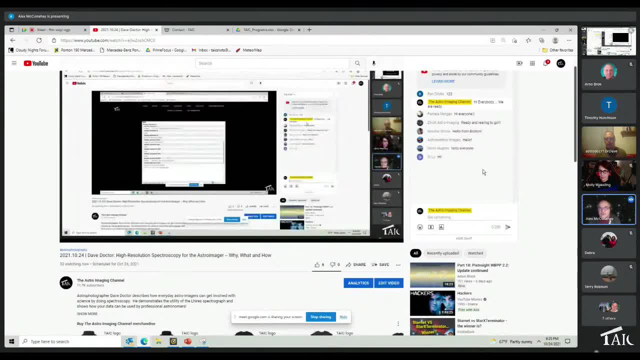 There's all sorts of stuff here, But mostly join in the conversation over here. It's part of what we do. We're a little different than the other programs. We've got one fellow that keeps asking us: why do we keep interrupting the presenters? 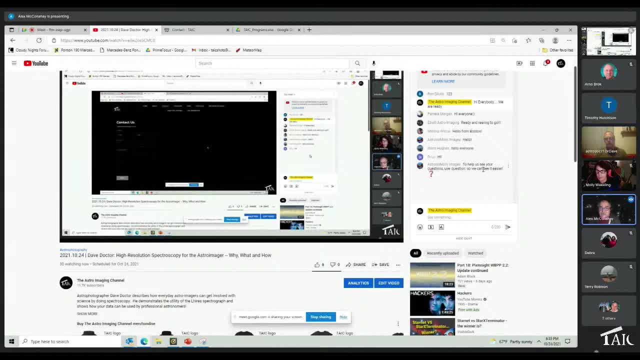 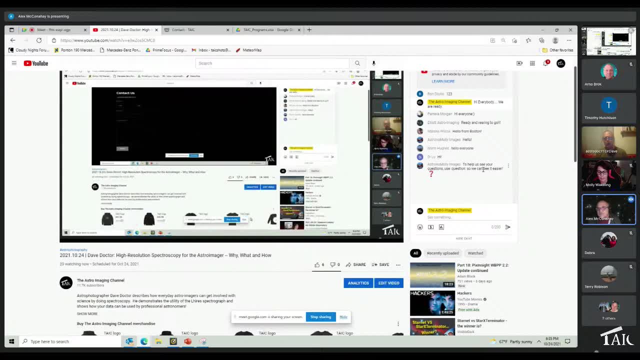 Well, we should tell you. we ask the presenters before each show about whether they prefer to be interrupted or everything held, And almost invariably they say no. when a question comes up, if it's appropriate, bring it up. We do wait until there's a logical break to bring it up. 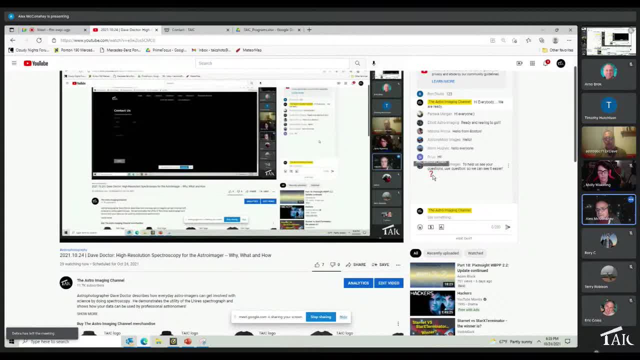 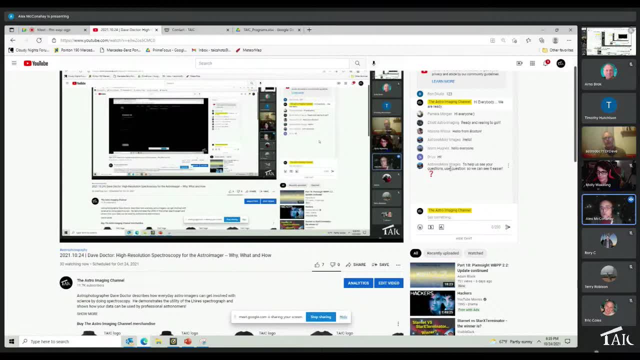 But if you've got a question like see what Astro Molly says, put that big red question mark in there and put it in Now. tonight's one of the nights where the presenter has asked us to hold off until the end. So get your questions in, but don't expect us to be interrupting like that. 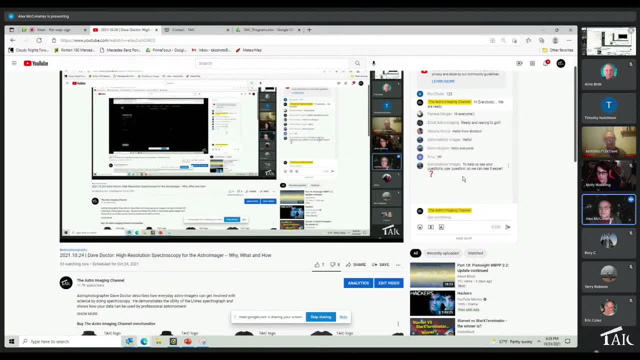 But anyway, that's why we feel it's necessary to interrupt. We're not like some programs where we've just got somebody that's going to get up there and talk the whole way through. It's somewhat interactive. That's why we rely on this information over and over. 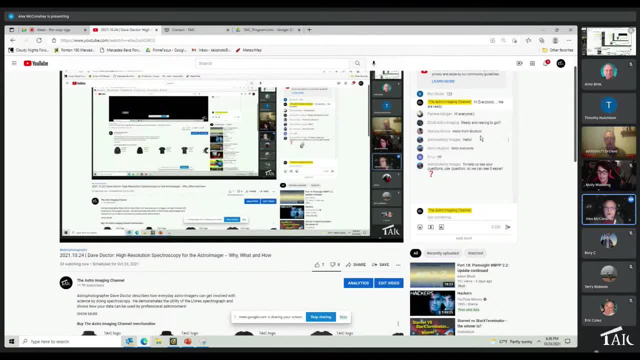 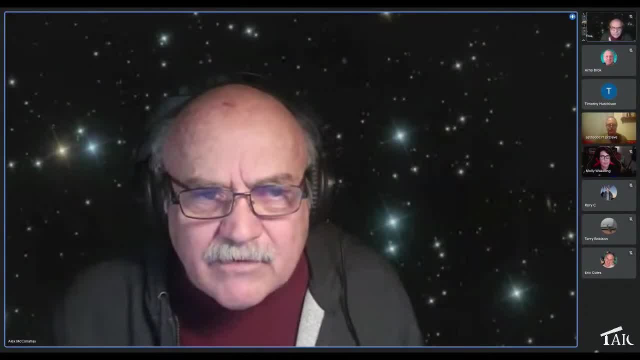 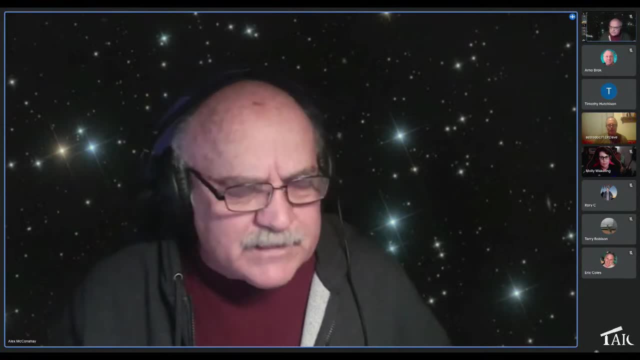 Okay, but enough about how we run the Astro Imaging Channel. Let me stop sharing my screen. And, Dave, are you about ready to come on back in with us? Yes, sir, Okay, Dave, you go take it over. Tell us who you are, what you're about and why we should be doing spectroscopy. 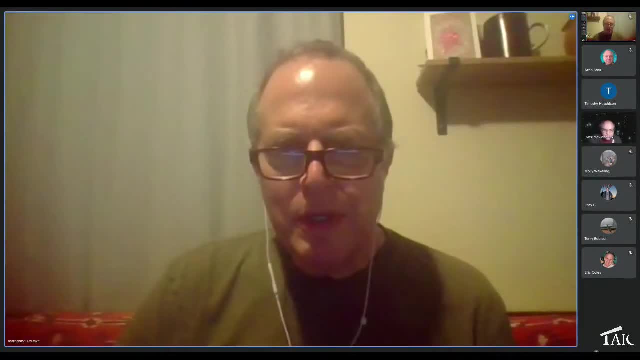 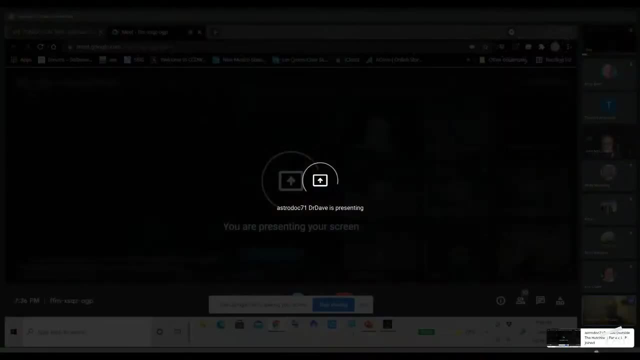 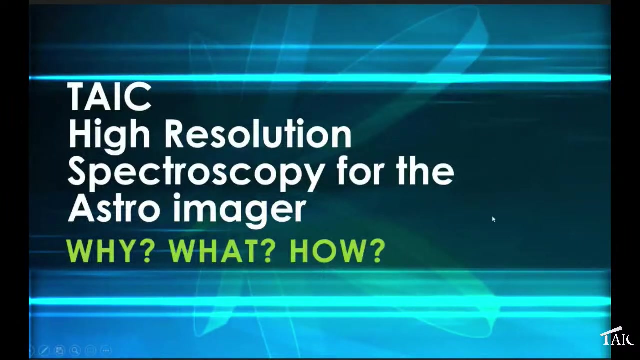 All right, Thanks very much. Let's see if we're good here. You're looking good, Okay And yep, there you go. You're pulling on, Cool, All right? Well, greetings from Las Cruces, New Mexico. 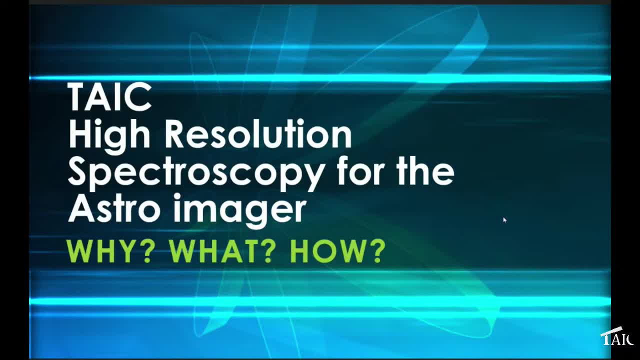 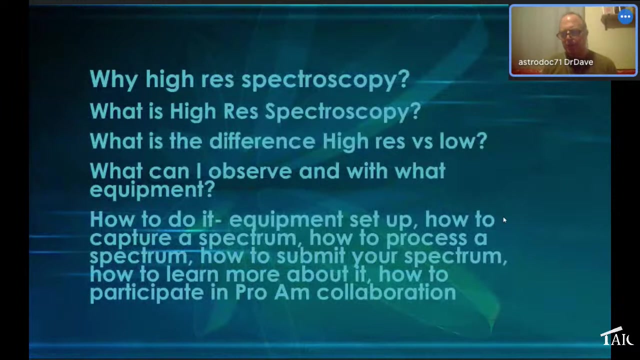 And that is actually located about three hours south of Albuquerque and four hours east of Tucson, And I just want to thank you guys for the opportunity to share something that's a little different than what you may be used to here on this channel. We are going to boldly go where few astro-integers have gone before, and that's into the realm of spectroscopy, and specifically high-resolution spectroscopy, which is growing in popularity. 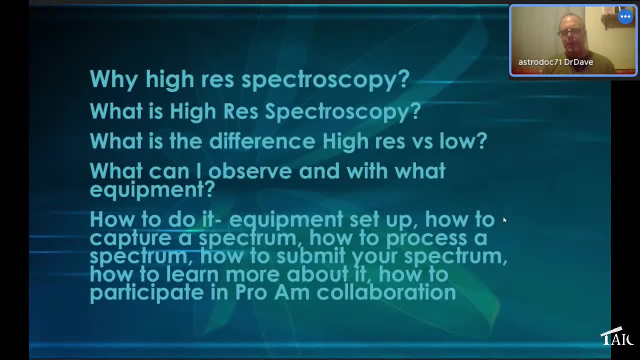 I would say it's hugely popular in Europe. not as much in North America, but I think it is gaining some traction here as well, And so what I wanted to do is just kind of give you a soup to nuts General overview of you know what it is, why you might want to do it and, if you did decide to do it, how you would go about doing that. 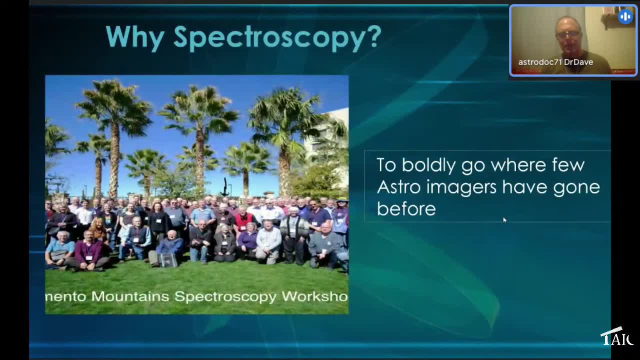 So just a little background on why I decided to be here. I apologize for the truncated caption on the bottom of the image here. This was the Sacramento Mountains Spectroscopy Workshop, which was held in Las Cruces. So think about it. This was about two to three years ago. 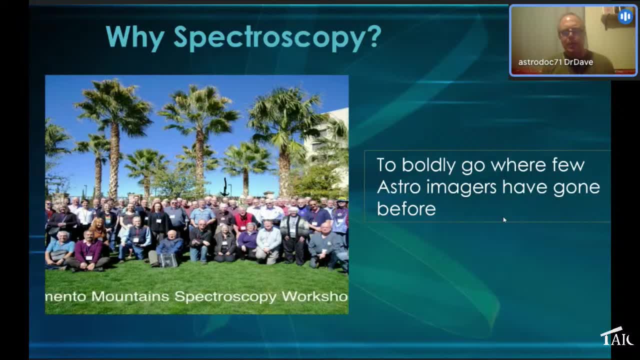 You can see me under the black arrow in the back there, But I am mostly an astro-imager. like many of you, I do remote imaging And about, I would say, 10 years ago I started playing around with the Star Analyzer, which is a low-resolution grading some of you may be familiar with. 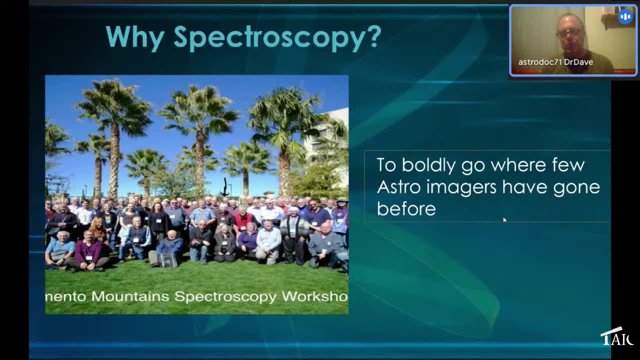 And I was frankly amazed at the stuff that you could see with such a simple setup. But I really wondered What the heck is this high-resolution thing about? And so I got a spectrograph And a couple of friends of mine who were avid spectroscopists and they were responsible for putting on this conference. they approached me and they said: hey, do you know anybody who has equipment? 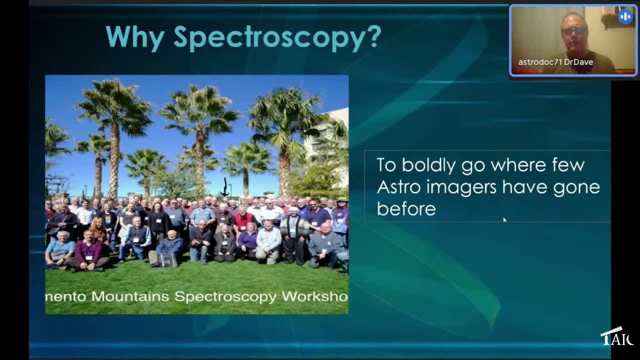 Because we really need somebody to do a demo for this conference. And I said, yeah, I got equipment. I haven't used it yet, But you know, but I have it. So I volunteered and realized just after that, gee, I only had a couple of months and I was going to have about 150 people at my house. 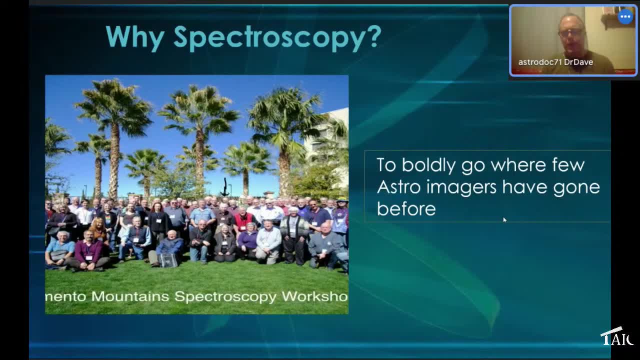 So I better figure this out pretty quick. And I was able to do that and learned a ton. And you know, after that I thought to myself: gee, you know that really that's really not that hard. In fact I was surprised and felt that doing like high-resolution regular imaging- 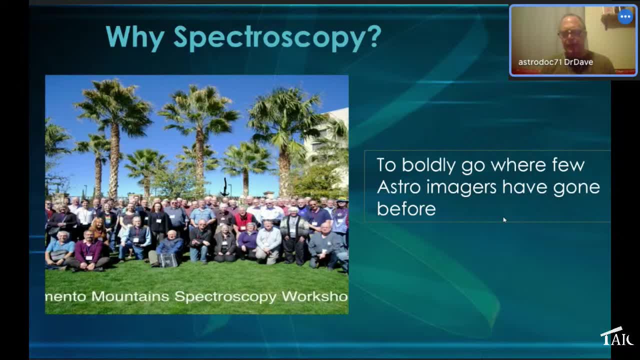 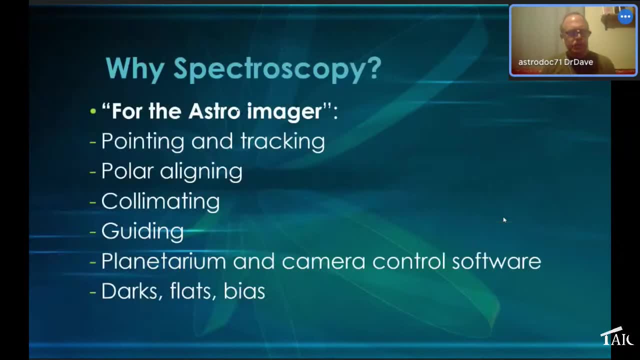 It really is a lot less forgiving, And so I decided to, you know, share some of the stuff I learned, And hopefully, at the end of this, at least one or two of you might get the same impression and they want to try it out. 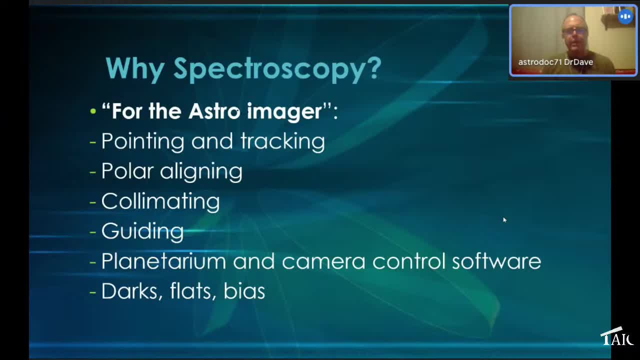 So I thought this was a great audience because you guys already know how to do pointing and tracking, You know about polar aligning, collimating, You know how to use a guide camera, You know how to use, you know, planar imaging. 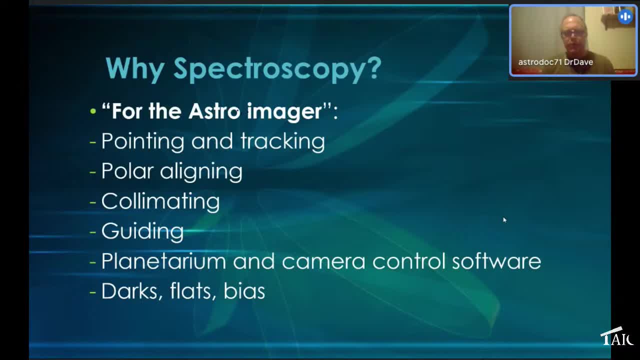 You know how to do that. You know planetarium and camera software And you understand the basics of image calibration. You're already 95% of the way there, So that's certainly one reason why you might want to think about it. 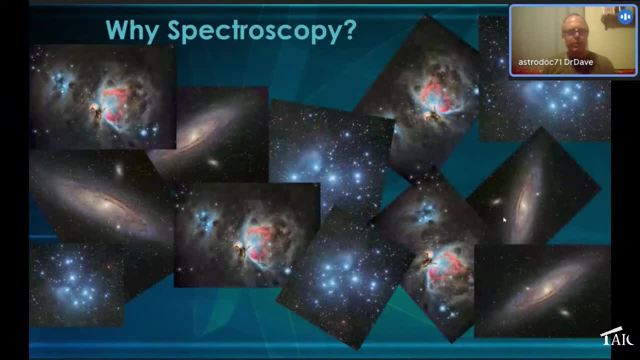 You know I'm an imaging fanatic, like a lot of you, And it never gets old. I get that. But look after your 800th Pleiades and your 700th M31 and your 600th Orion Nebula. you know, maybe you might. 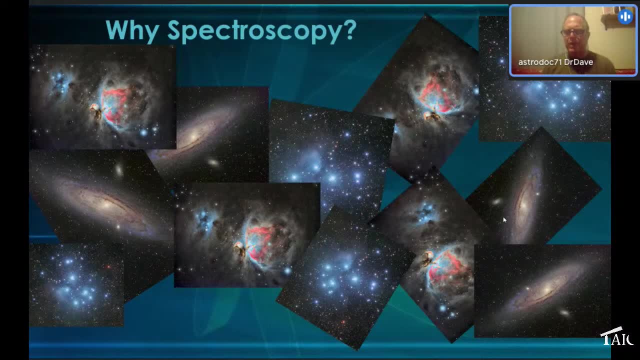 ask yourself: gee, you know, is there something else I could do that won't necessarily take away from my imaging schedule completely, But something that's interesting and fun, that you know I could do on the side. And yeah, there definitely is something you can do. 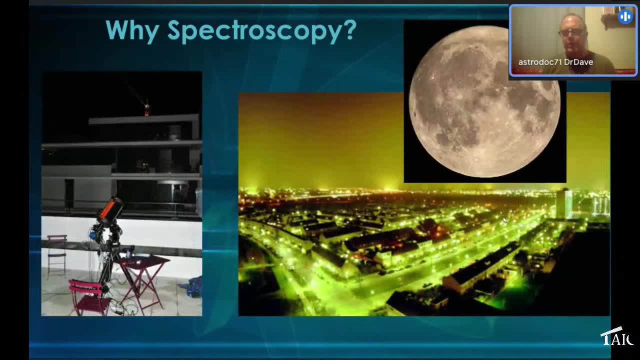 You might be in a situation where you're in a Bordeaux 50 sky and there's no way you're going to get to a dark sky side anytime soon. You know the moon is not our friend for two weeks And you may be getting tired of you know, the Hubble palette, for example. 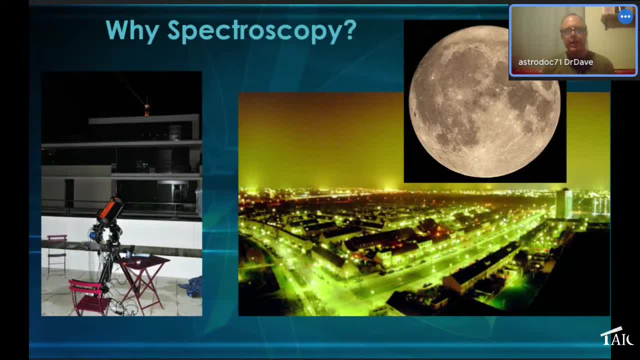 But the great news is that spectroscopy doesn't really care about ambient light. surprisingly, In fact, this setup on the left here is an amateur spectroscopist who is in Paris and has her setup about a block away from the Eiffel Tower. 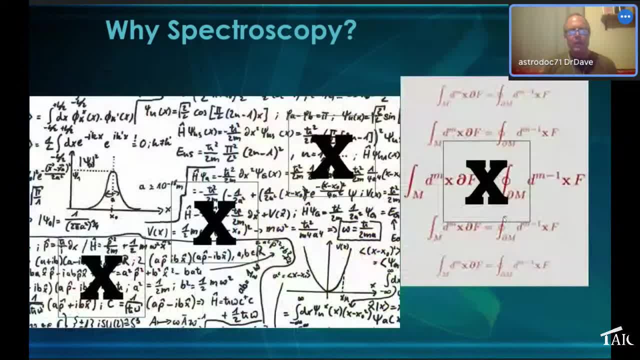 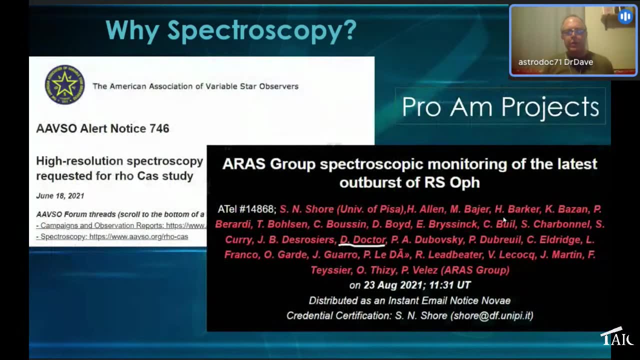 So you can imagine what that's like. Do you have to understand vector calculus and quantum mechanics? No, you don't have to understand any of that, And I've been doing this for a few years and I still don't understand it. One of the most compelling reasons for doing it is that you are virtually guaranteed to participate in a direct, meaningful way to astronomy research. 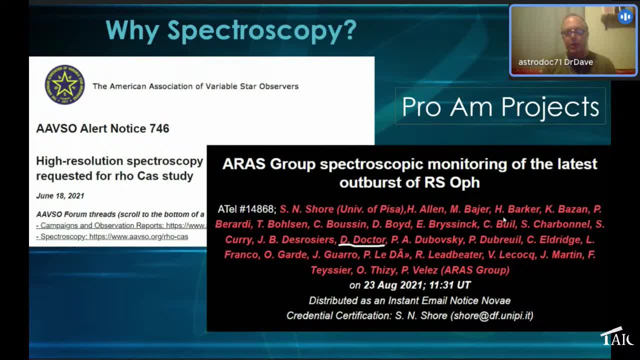 And discovery And it's one of the few areas in our hobby that's still a possibility. This was a project I did on the relatively recent nova outburst. I know some of you were imaging And I got kind of late. I was a little late to the party about maybe a week and a half after the peak. 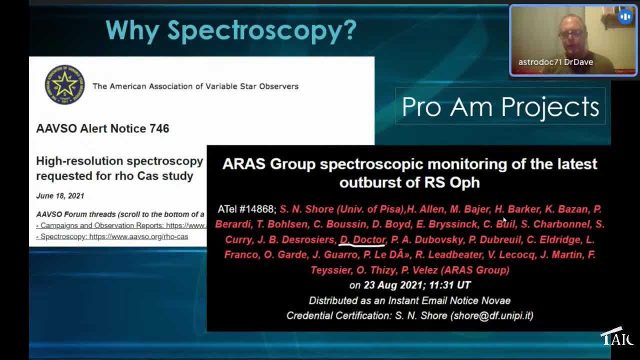 But I was excited because you know a lot of novae are pretty dim and you really can't do much with them, But this one was bright. This one was bright enough where I was able to take a couple of spectra and you know I submitted it. 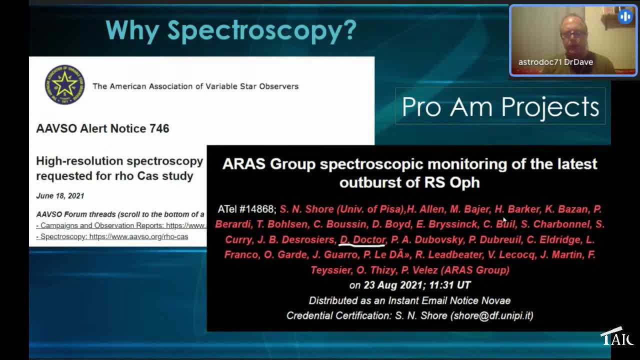 And a couple of days later it was part of the astronomical telegram, So this is a definite. this is something that you will be able to do on a regular basis pretty easily If you become a member of the American Association of Variable Star Observers. 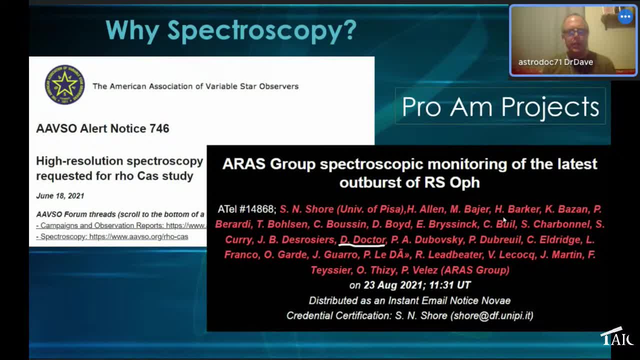 you will get bulletins from them every couple of weeks And there will be plenty of projects. Believe me, the professionals need your data. They're going to bug you for it once you get involved with this, So there's not going to be any shortage of work. 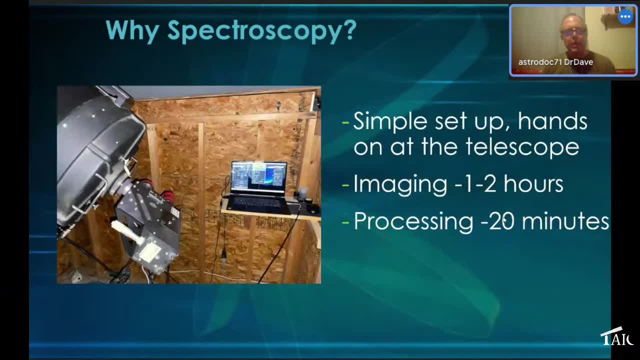 One of the reasons I like it is it's kind of it's relaxing for me, Because for those of you who do remote imaging, I'm sure you can relate to being anxious about things like you know: software crashing and cameras timing out. 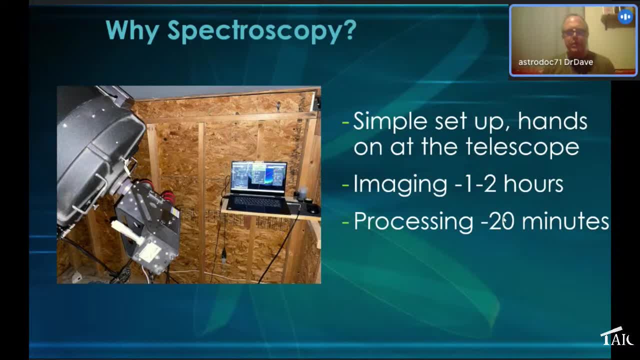 and your roof doesn't close and the internet drops And it can be really stressful. This is really great because it's all hands-on. It's a very simple setup. I have a home-built roll-off in my backyard in Las Cruces. 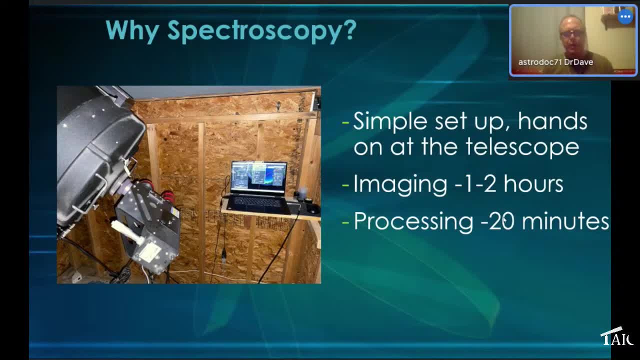 I just set my laptop up on the shelf. I've got my spectrograph here on the left I use a C14. The projects are super short. They're like maybe an hour or two And the processing literally is like about 20 minutes as opposed to. 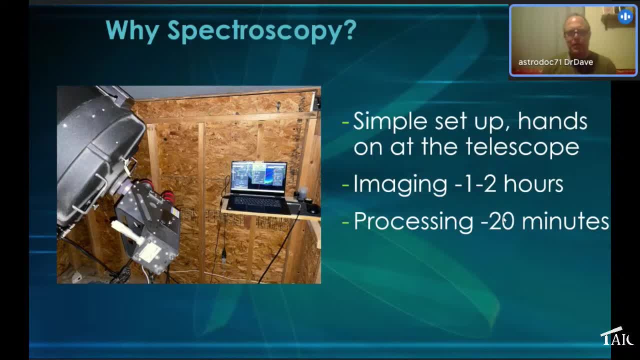 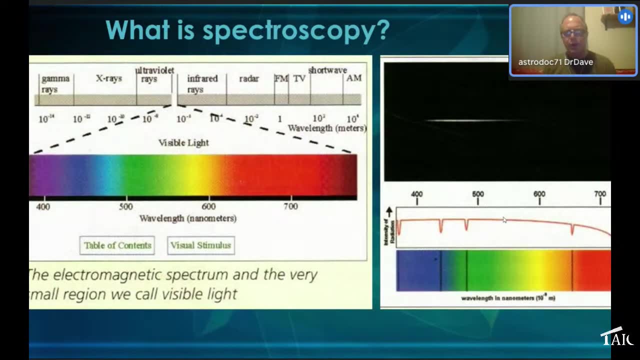 you know a minimum of 20 hours with PixInsight and Photoshop. So what is spectroscopy? Well, you know a lot of what we know about how the universe works comes from spectroscopic observations: The simple diffraction of light into its component. 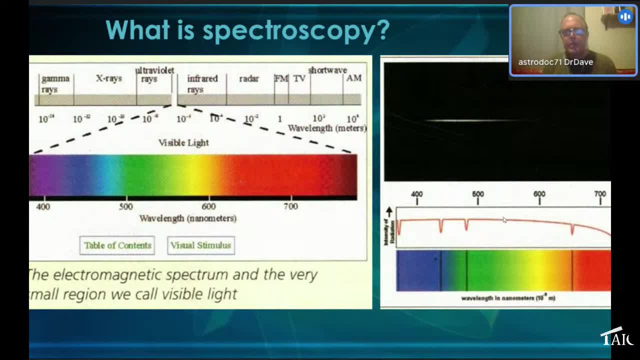 colors or wavelengths, gives astronomers the ability to figure out a host of physical properties of whatever they're looking at, And this can be anything from velocity, temperature, mass and a host of dynamic processes that are occurring in the object. For us, as amateurs, we're focused on the visible light. 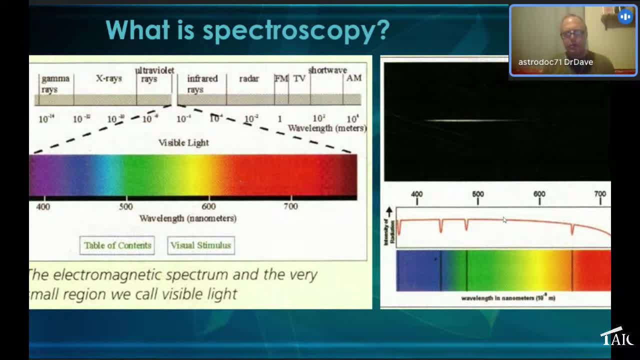 which is from about 4,000 or so angstroms to around 7,000.. On the right here you see, this is a low-resolution spectrum I took of I think it was Vega or it was a spectral type A star. 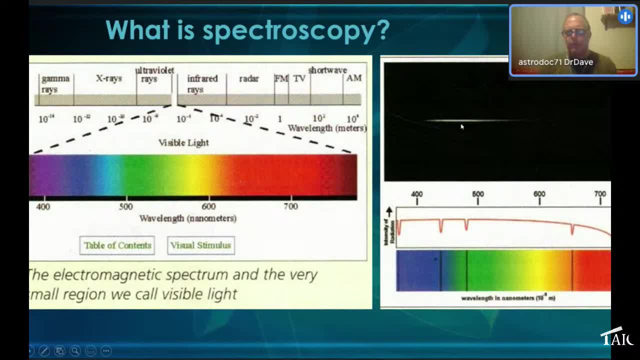 And I don't know if you can see this- There are these little vertical black lines. These are absorption lines, And on the bottom here this is a typical spectral plot where you have intensity in the y-axis and the wavelength is in the x-axis. 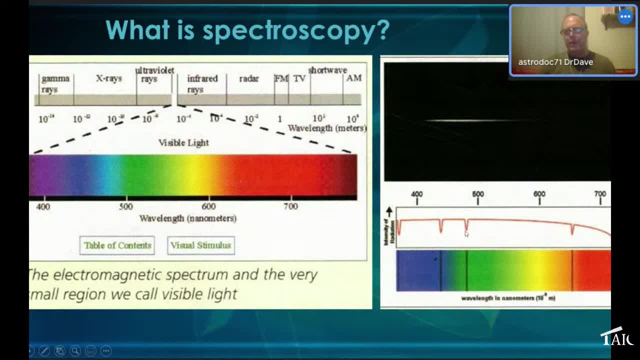 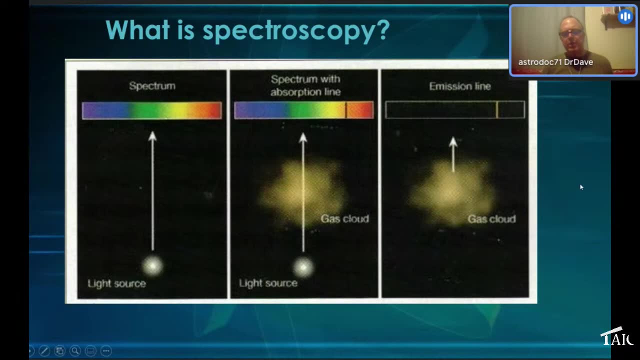 And you get these little dips here. these are the absorption lines that occur at the discrete wavelengths, And if these were emission lines, they would be flipped and the intensity would be increased at the same locations. There, basically, are three different types of spectra. 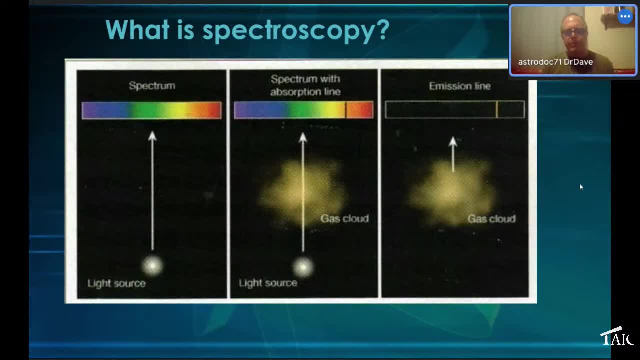 On the left is what's known as a continuous spectrum. That's produced by a very hot opaque body like the inner photosphere of a star, And you get a spectrum without any lines in it. If you have an intervening layer of gas, that's cooler. 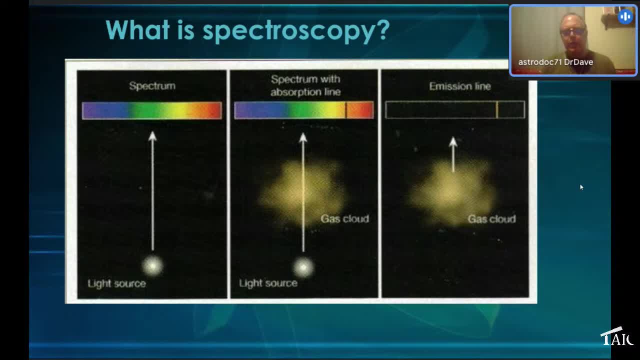 that's going to absorb the light or the energy from the inner photosphere and that's going to cause a superimposition of the absorption line on the continuous spectrum And, in the case of an emission spectrum, you're going to have a hot, low-density gas, kind of by itself. 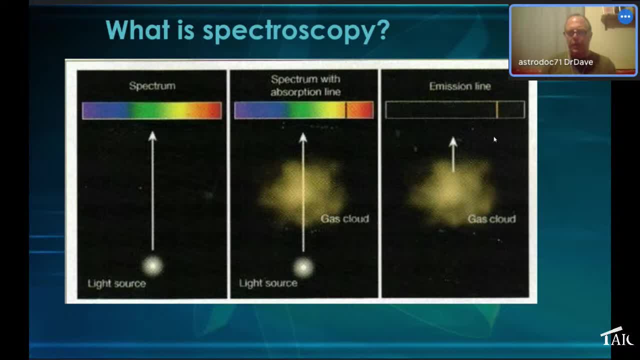 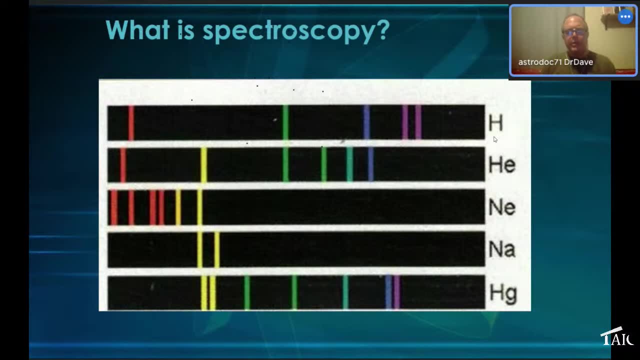 With nothing between it and you, and that's going to give you an emission line. All the elements that we know have this sort of barcode of potential spectral lines based on their atomic structure, and those potentially could give you absorption or emission lines, depending on what's happening. 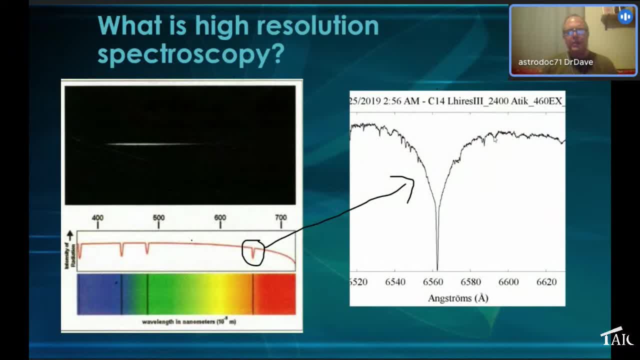 So what is high-resolution spectroscopy? Well, that's similar to, in a way to regular imaging where, for example, you have your 500-millimeter focal length wide field set up, where you're taking the beautiful Milky Way shots. 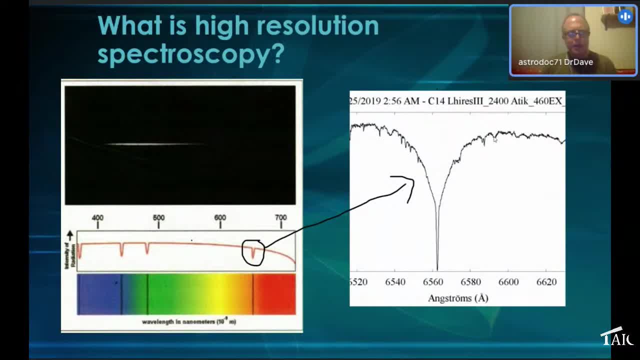 and nebula shots and then you got your 0.5 arc second per pixel galaxy images. So here, what we see on the left is a low-resolution spectrum, what I showed before. And if you take this hydrogen alpha absorption line here and you blow it up using high-resolution equipment, 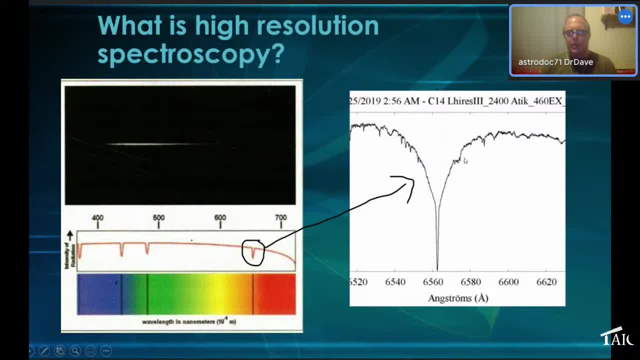 you can see all these little lines here in the line profile. This is about a 100-angstrom field as opposed to, you know, a 3,000-angstrom, the whole spectrum that you see with the low-density setup. So you can imagine that subtle changes in this line profile. 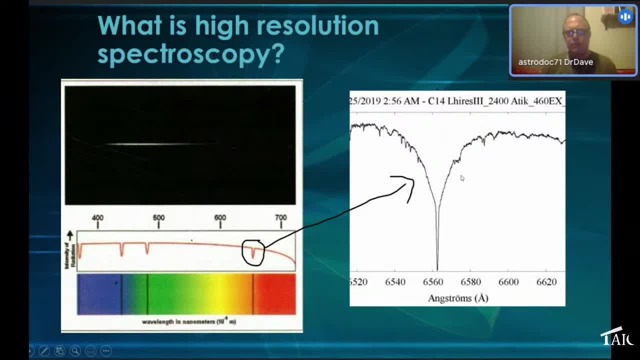 could indicate a host of events, anything from mass ejection in the start and maybe interaction with the binary. A lot of these, a lot of processes that occur on these objects, are figured out just by these small alterations. or sometimes they're huge, like in the case of ANOVA. 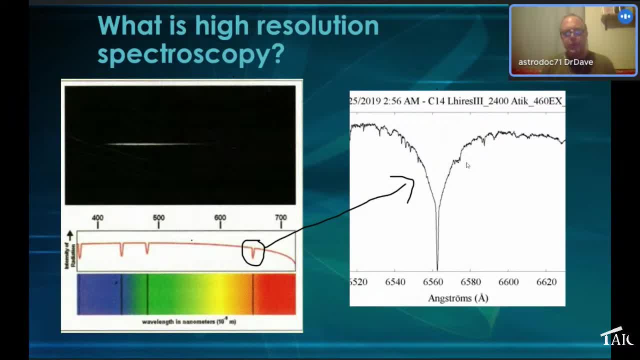 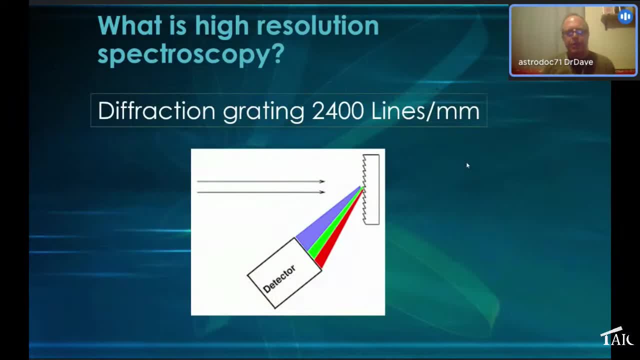 But more information that can be gathered from these single absorption lines than you might think In a spectrograph, which is the instrument we use. the resolution is determined by the number of lines in your diffraction grating, which is basically a block of glass. 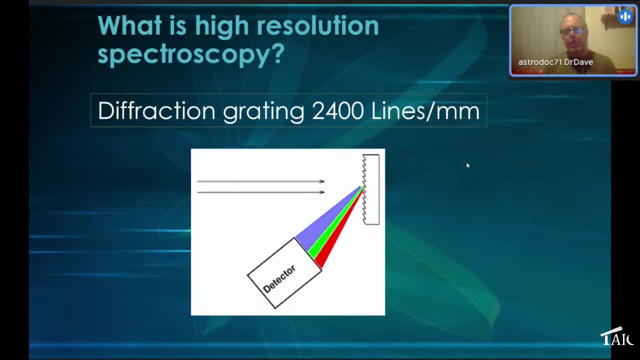 with a bunch of etched lines in it. So in a high-resolution setup you have maybe 2,400 lines per millimeter and low-resolution might be like 100.. In the spectroscopy world the R value is the resolution. 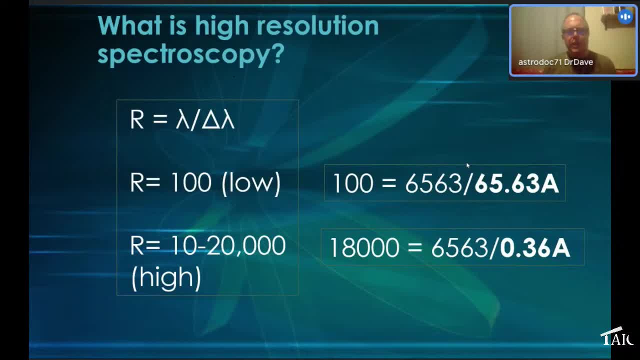 and that's defined as the wavelength you're looking at divided by the smallest wavelength increment that you can resolve. So for a low-resolution setup, you're going to be able to see maybe 66 angstroms as your smallest detail, but in a high-resolution it goes up to or down to. 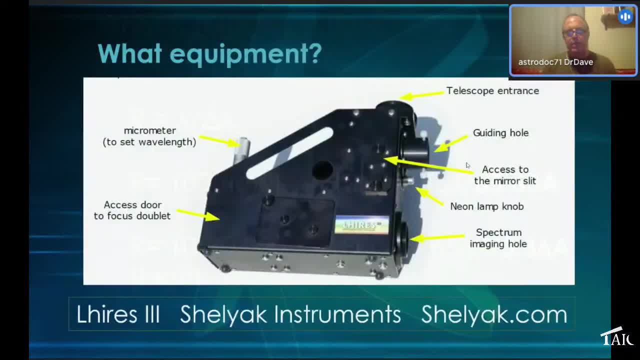 like 0.4 angstroms, which is that's a pretty big difference. So what equipment do you need? So for myself, look, I'm not a mechanical engineer, I'm not an electrical engineer, I'm just an old country doctor Jim. 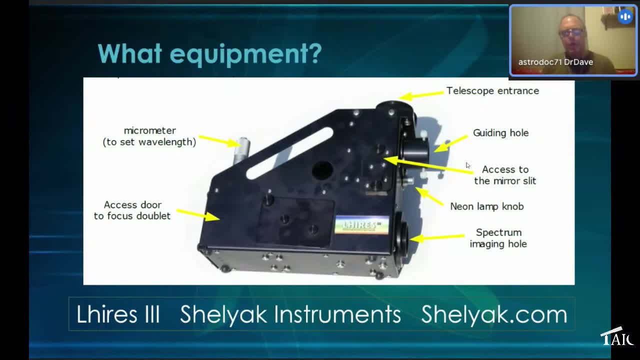 So I kept it simple. I didn't want to reinvent the wheel. This is the L-Hi-Res III, which is manufactured by Cheliac Instruments in France, and the L stands for LITRO, which is the type of spectrograph design that it has. 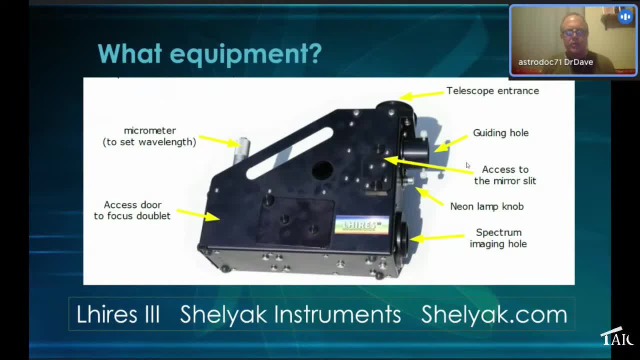 Don't have enough time to go into the different ones, but needless to say that for this unit everything is there. You've got your guide port, so you don't need an extra guide module. You have your both your calibration lamp and your flat lamp. 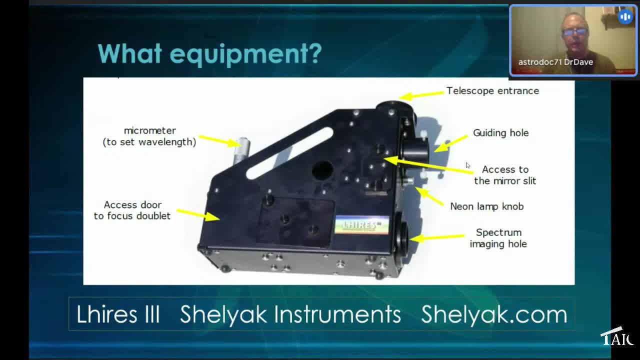 are already in there. You've got your micrometer that you can scroll to different parts of the spectrum, And it's pretty much ready to go right out of the box. Now there are other options If you are, if you are, mechanically inclined. 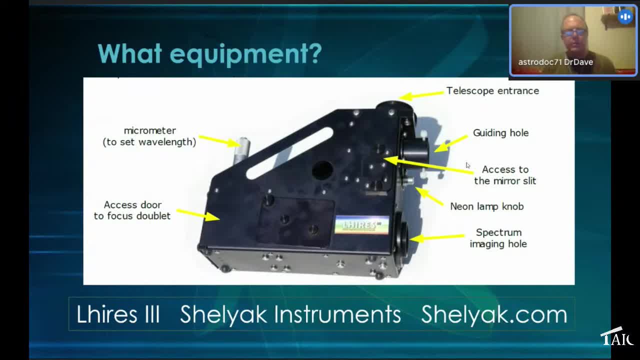 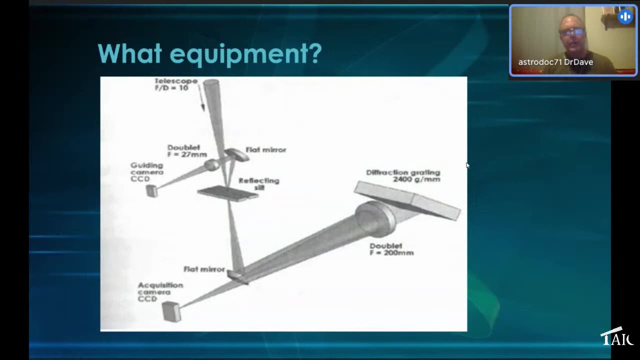 there are spectroscopy groups that actually are 3D printing their own spectrographs, and there are kits available, So there are plenty of options for just about any type of background. It's a very interesting setup. You can kind of think of it in a way as like a mini folded refractor. 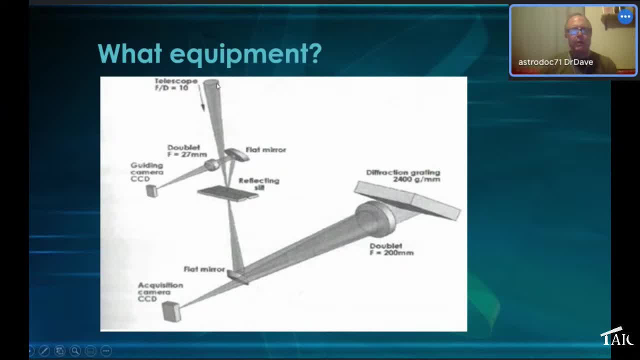 So you have your light that comes in from the telescope. It goes down to this reflecting slit here, That's what it's called. There's a 23 micron slit, that's in the that bisects this thing, And so you have a light that reflects off of that onto this mirror. 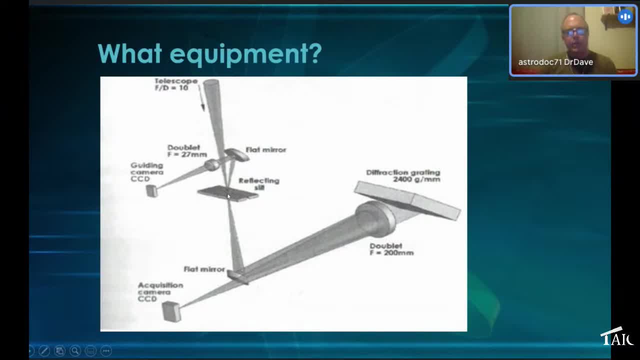 and into your guide camera and the rest of it, or the portion of it, the small portion of it, going through the 23 micron slit, goes to your acquisition camera And it bounces off of of the diffraction the reflection grading back through this 30 millimeter doublet lens onto. 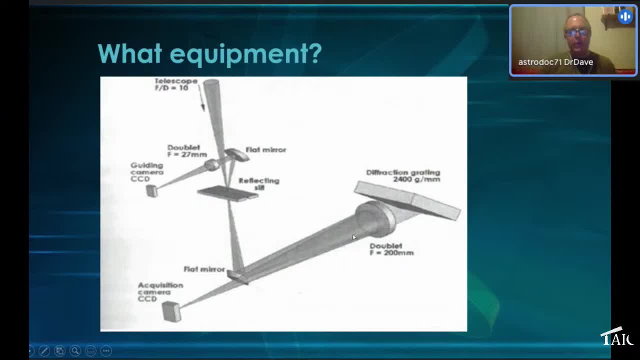 your CCD. Now there is a tilt here about 10 degrees, Otherwise the, the, the slit image would just go back out to the sky, And that really wouldn't help us too much. But the one thing you really want to get from this diagram is that the 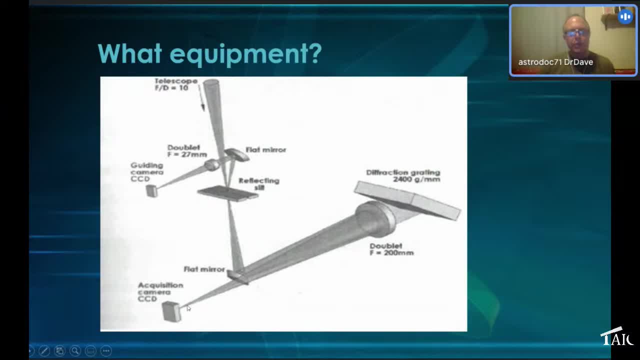 your camera, your acquisition camera. here your where you're going to see, you're going to record your spectrum. It doesn't know anything about what's happening outside of the spectrograph. It doesn't know where your, your telescope is, where you're what. 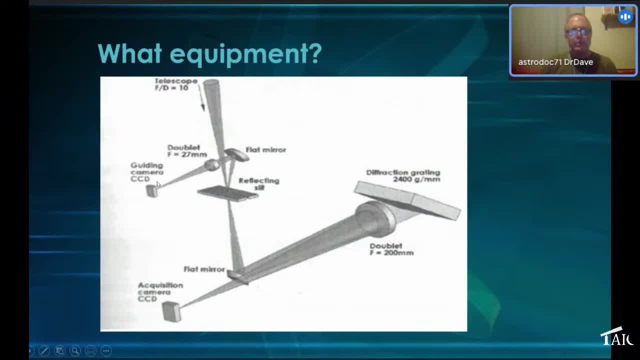 what you're looking at. So your guide camera has to be your eyes as well as your guider, And it has a little more importance in in this, in the setup here. This is just to illustrate some of the features of the Elhira, as you have a. 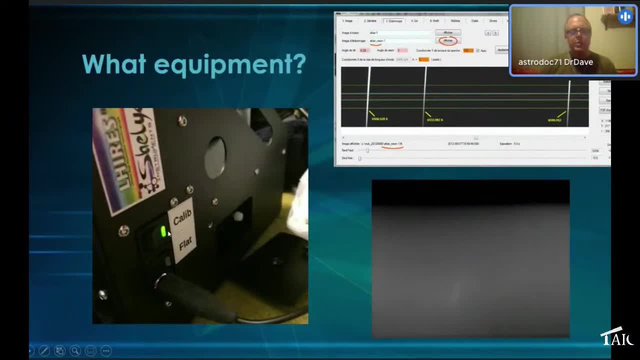 calibration lamp and a flat lamp. It's just a simple switch. It's a requires a 12 volt power source. You can hook up an adapter to plug it into a regular outlet. This is what your calibration lamp produces here. If you took 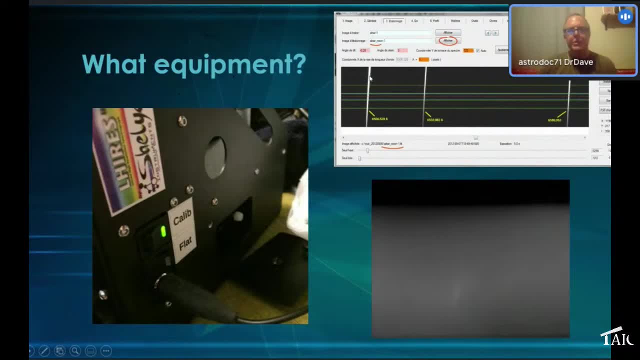 take an image of it. it's a neon lamp, So it produces a bunch of emission lines in the red end of the spectrum. So your hydrogen alpha is going to be in here somewhere And the the neon lines you can see here. 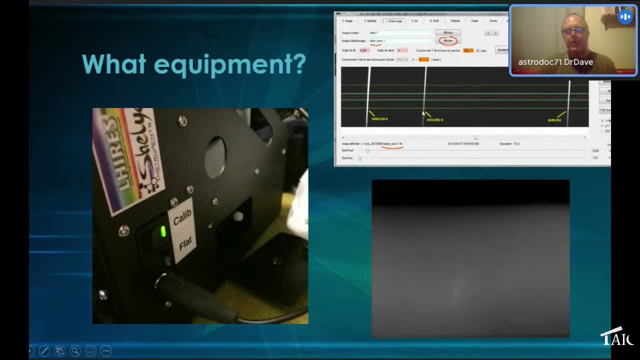 and they have specific wavelengths And those are used to calibrate your spectrum. So you got to tell your your software which wavelength goes with which pixel. That's basically what this does. On the bottom here is a is a flat image. 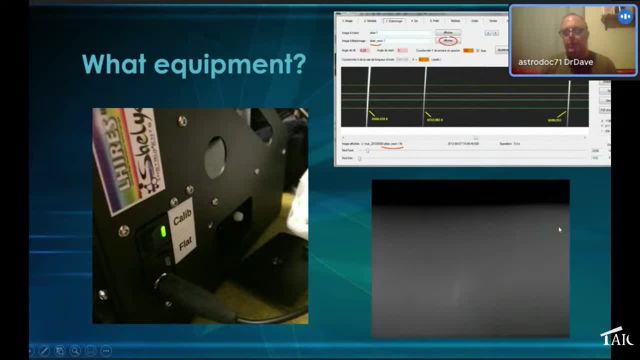 which kind of, in a way, looks a little bit like what we're used to seeing. This is a tungsten lamp and it's just a. you take your flats at the end of the night. They're just about eight second exposures. What cameras. 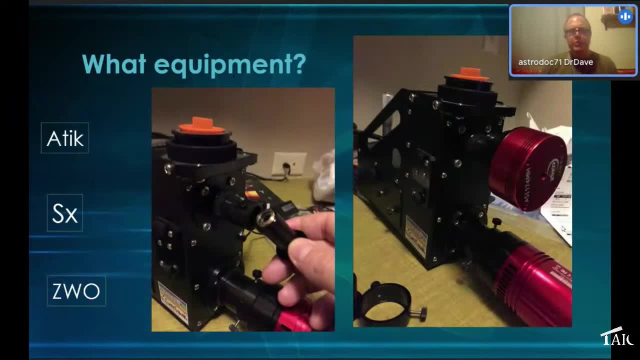 The, the attic cameras are very popular And I think the reason is because the sensor has a, has a QE. that's a little bit skewed to the, to the red, And since you're imaging an H alpha most of the time, it does help you. 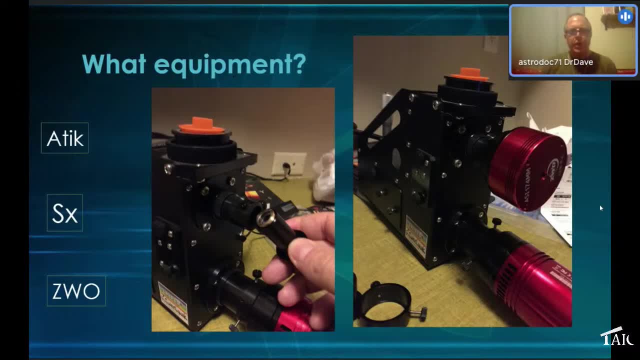 But a bunch of different cameras can work. Starlight express, ZWO, ASI cameras are great, but you have to look when you look at this. okay, this is my guide camera And this is your, your imaging cameras. 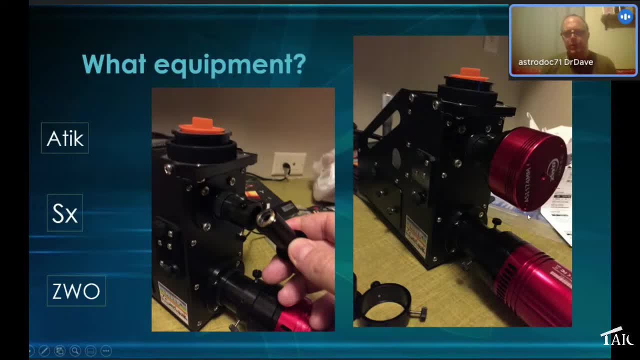 not really a lot of space in here for a lot of bulk, So you have to be careful with, you know, things like S big and maybe some other ones that may be a little bit tighter, And and also the, the unit. 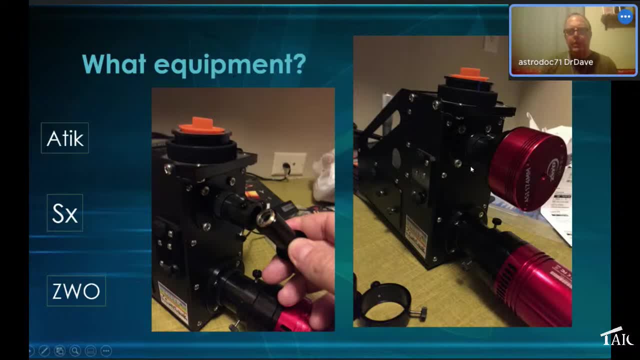 only weighs about two to three pounds, So it's not really. it's not really that heavy. And these, these ports are not really super. you know well, they're not really built to accommodate a lot of camera weight, So you just need to be aware of that. 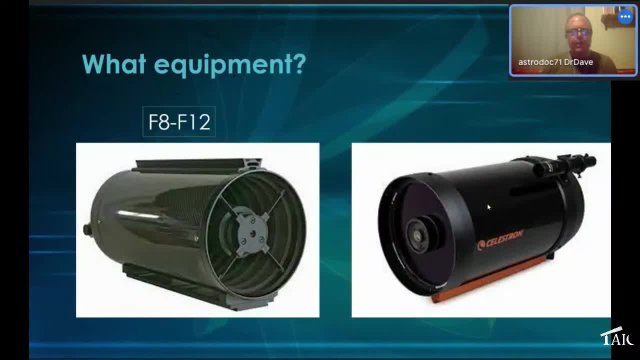 When, when you're setting this up, telescopes generally want to match your, your optics, to the, to the focal length of your, of your spectrograph, which is about F10.. So in this range of F8 to F12,. 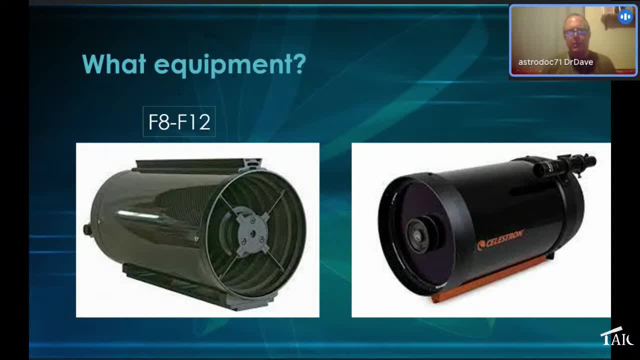 that works pretty well. Classic SCTs are great. You know your, your C8s, your C11s. I have a C14.. You can use RC scopes. You can pretty much use any scope, As long as you realize that if it's going to be out of this range, 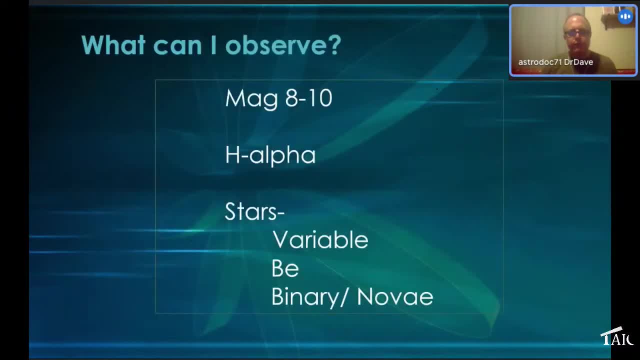 then you're going to probably need either a Barlow or a focal reducer. So what are, what are the things that you can observe? Well, you have to remember high resolution. you're going to have a lot more dispersion, So it's going to dim things up a bit. 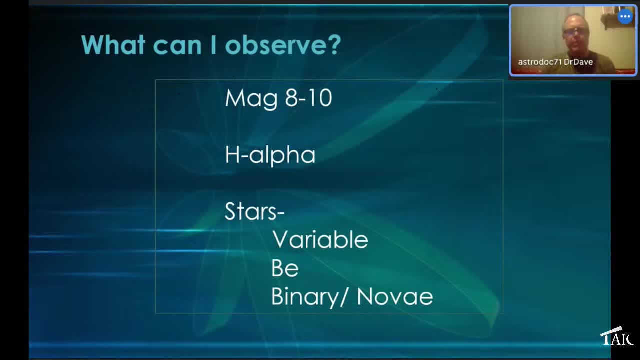 and that's going to limit your magnitude to probably in the eight range. So you're really going to probably be looking at stars mostly, And that's really where most of the research is at Variable stars, the so-called BE or B emission stars and binary stars. 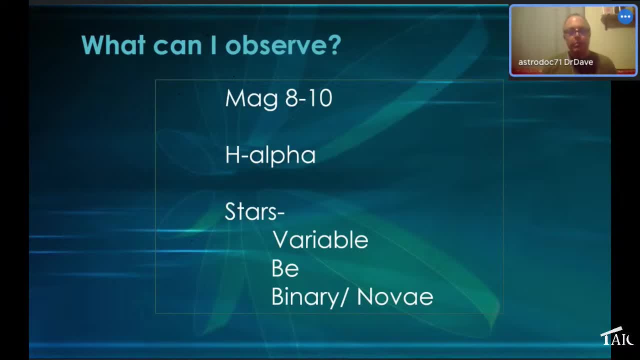 and occasionally NOVI are, are good targets. You're going to be probably doing H alpha for the most part, because that's where the strongest signal is in most cases. But if you're not, you're not. there's nothing written in stone on that. 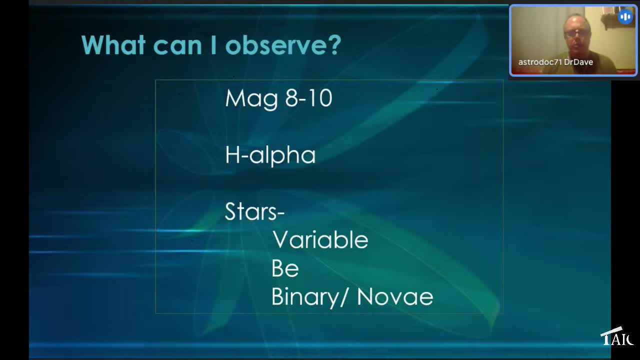 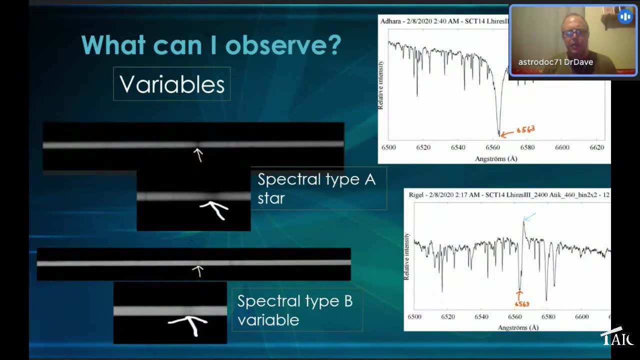 You can certainly go to other regions of the spectrum that we'll get into in in a little bit. So variable stars. So those are stars that have intrinsic variability from pulsation in a in a unstable atmosphere, changing in brightness at varying periods. 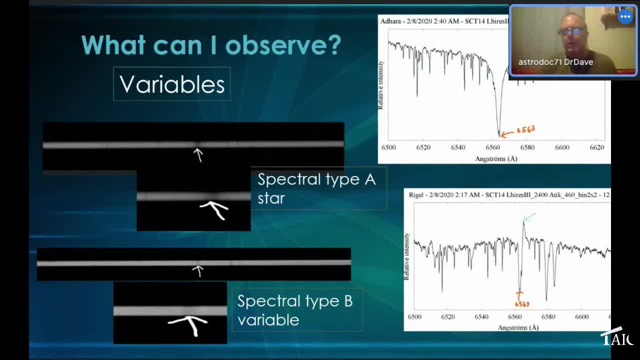 So I just have an example of a typical spectrum of a spectral type A star. This is Adara, which is in Gemini. It's like you know, it's a very, very low magnitude- two or so- And this is a fairly typical absorption line profile that you see. 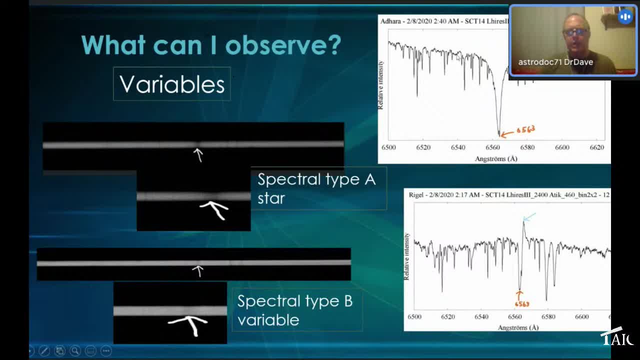 Here's your 65, 63 point there. These lines here are mostly a water vapor. nothing really really special there, but just to give you an idea. And then, excuse me, on the left here you see the the Ross spectrum and here's your. 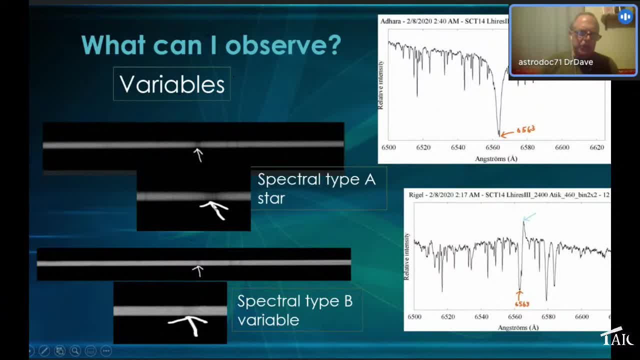 your absorption line where the white arrow is, And I blew it up a little bit too so you could see it a little, a little easier, And that's definitely different than what you see on the bottom. So this is Rigel, which is a variable star. 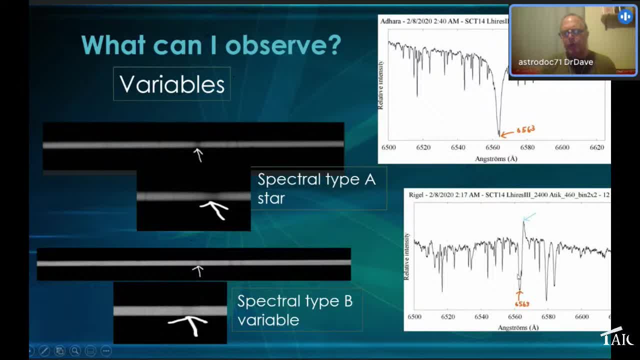 And what you notice is this line profile has what you call an emission wing here. This is a region of emission and that's caused by stellar wind That's close to the star And this is actually moving away from us because it's toward the red. 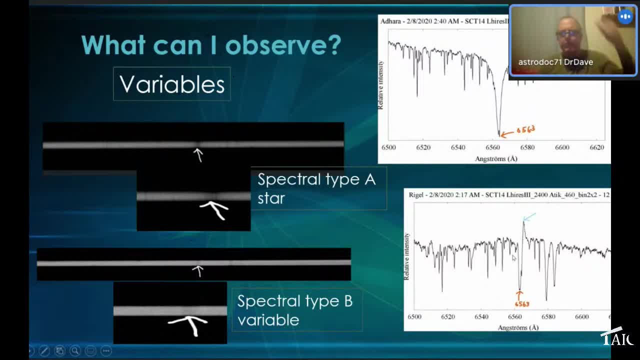 And you have this material that is showing absorption and that is moving toward us. So this sometimes is flipped. It changes pretty frequently. So it's a pretty dynamic system And if you take spectra on a weekly basis, you see the changes that are pretty dramatic. 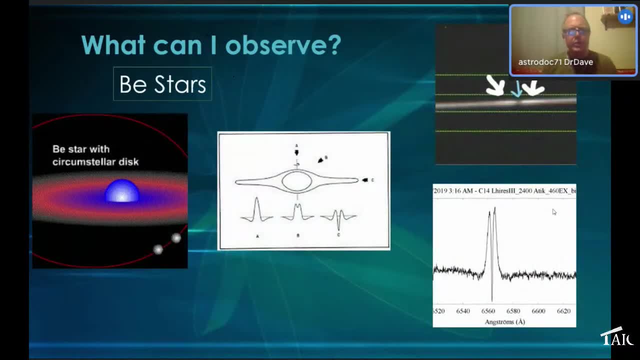 This is. this is a subset of stars. You're going to probably be spending a lot of time here. These are a B, so-called B admission stars. They're a spectral type B that have that have a rapid rate of rotation, about 200 kilometers per second or greater. 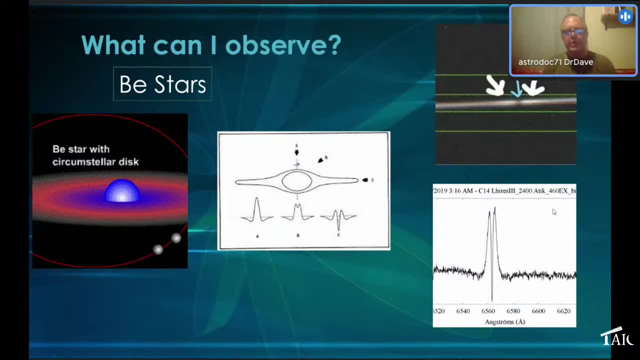 They form a large circumstellar disc, And so this on the upper right- this is, this is my bad here, because this is not. this should be horizontal. This is one of the earlier ones that I took, But in any event, you see, here's the absorption portion. 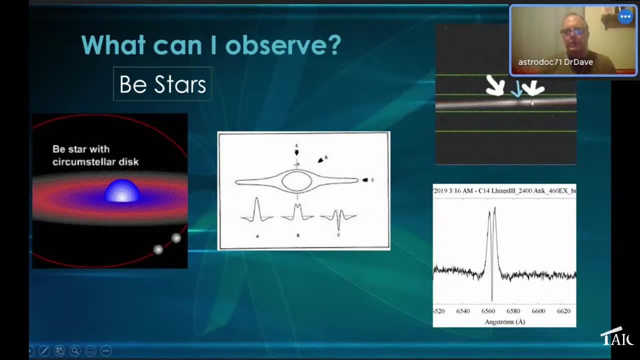 And on either side of that you see what's what's called an emission globe. So on the bottom here you get this kind of bi-lobed line profile, which is pretty interesting. And if you look at this schematic here, 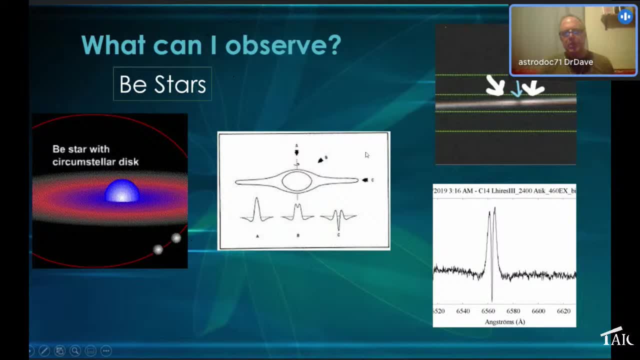 this kind of shows you what you can expect to see, depending on the observer's location around it. So if you're looking directly down onto the star and you see mostly the circumstellar disc, you're going to get mostly the emission component, because the disc is going. 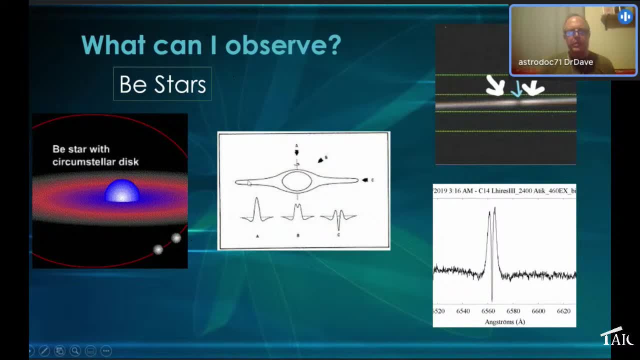 to dominate, But as you shift over and start looking at it from the edge, you're going to get more of an absorption component from the actual star itself. So this was really cool. This was the. this was the. this was the. 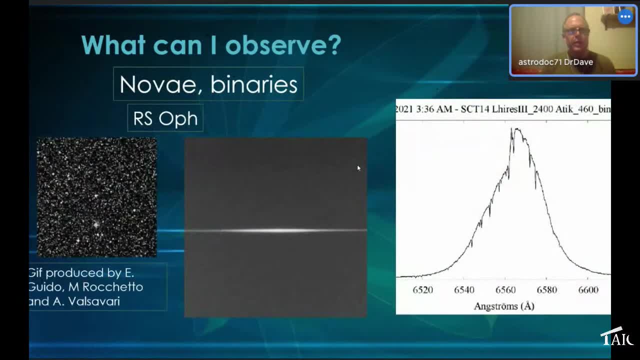 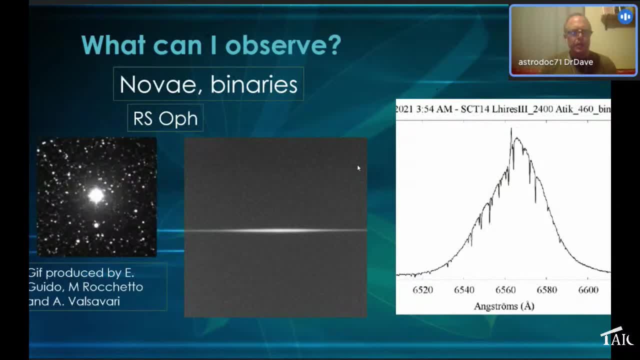 I know some of you looked at it visually. This is a visual gift produced by the imaging team of Guido Roquetto and Valsavari- Hopefully I'm pronouncing that right, But this shows a dramatic change that you can see there. 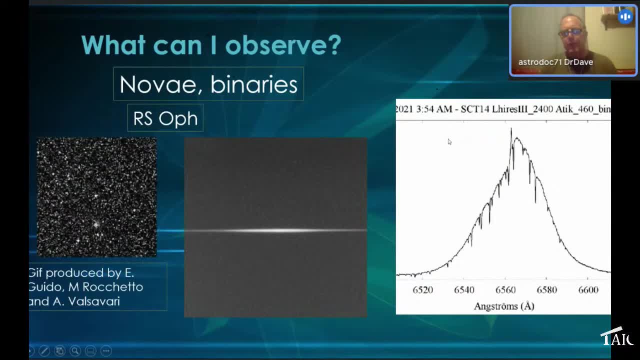 And on the right is the spectral version. But the thing is with this on the right- Valsavari- I was about a week and a half late. So this is just two observations, two or three days apart, And this was already a week, about a week and a half after the peak. So what you see here is a very large emission zone from this is the ejecta from the explosion. 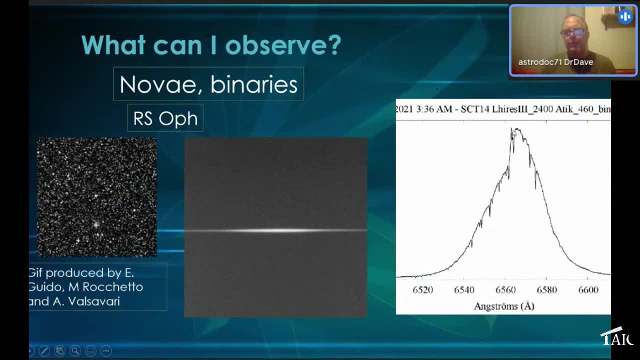 And this is the hydrogen peak, the hydrogen emission peak, And by now it's kind of lost in this continuum here. But you can see that this is a very dynamic system And if you image this, if we were to image this every night, there'd be some significant changes there. 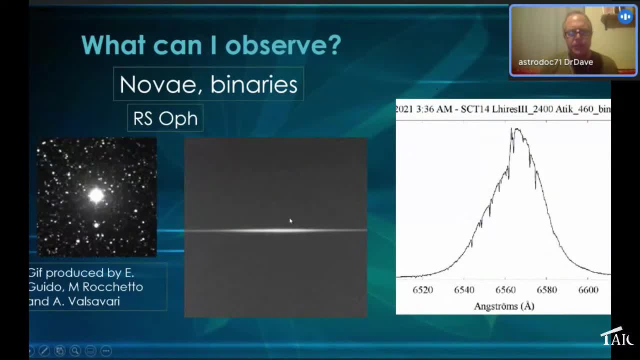 The middle portion here is: this is a. This is a raw spectrum showing the emission, the raw emission spectrum, And then you can see this broad brightening here. But this NOVA is a binary. So you had your red giant and your white dwarf And what was happening is the white dwarf accretes material from the red giant. 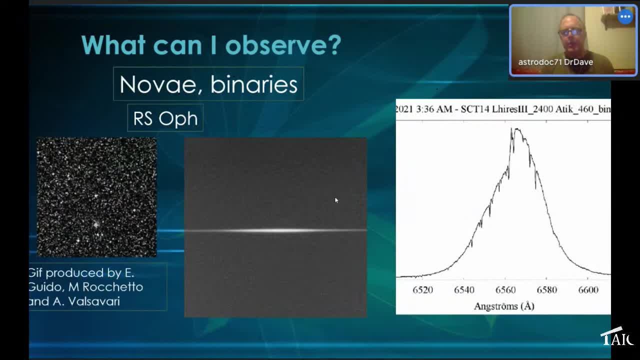 And it gets to critical mass And that triggers what they call thermonuclear runaway And that causes the explosion. So that was a pretty cool thing. Now, NOVI are not always visible with high resolution equipment because they're typically a lot dimmer than what this was. 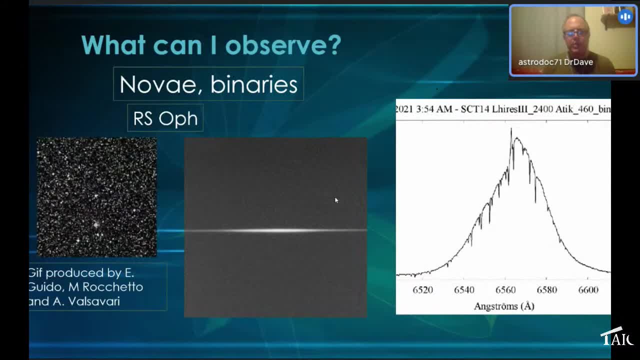 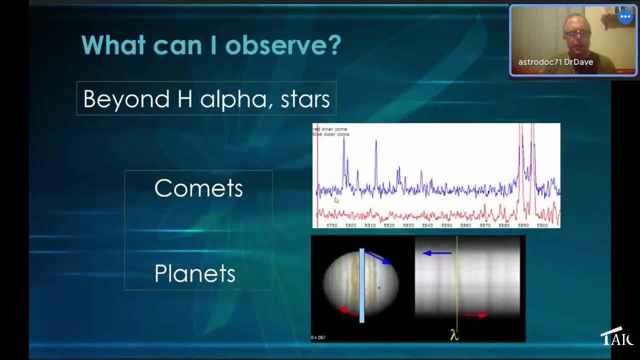 So this doesn't happen that often. They're just lucky to be able to see that. Well, what else can you observe? I mean pretty much anything that you can see, up to the limiting magnitude. The comets are very popular. This was NEOWISE, I think, and that was bright enough where you could actually get a 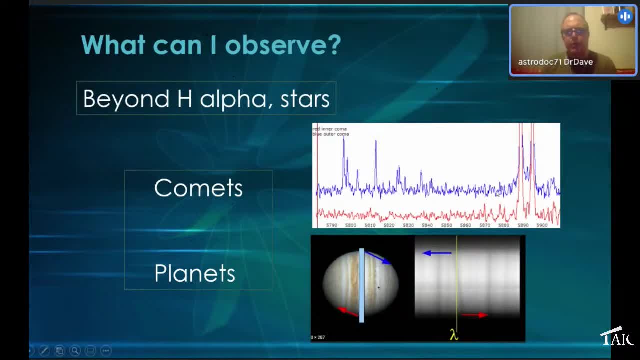 You could get a spectrum of both the inner and outer coma. You can see the sodium emission lines. There's a cool project you can do where you can calculate the rotation of Jupiter by looking at the Doppler shift of the spectral line, where you have the blue shifted on one limb and the red shift on the other limb. 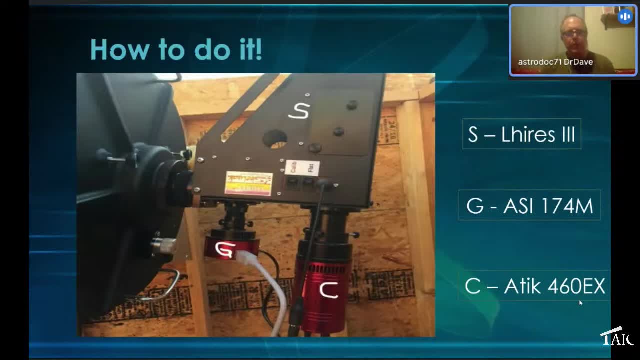 So now, with that, we want to know, well, how do you do it? If you were to decide to do it, this is my setup here: spectrograph camera and guider, And I have the C14 there on the left. 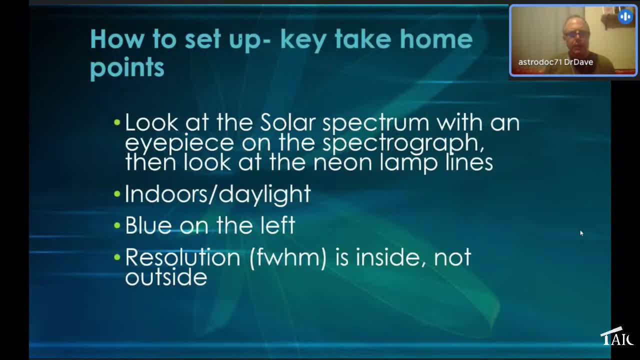 So the key take-home points is: if you're going to go with the L-hi-res and you get your spectrograph, you want to look at the solar spectrum with an eyepiece. It is safe to do that, by the way. 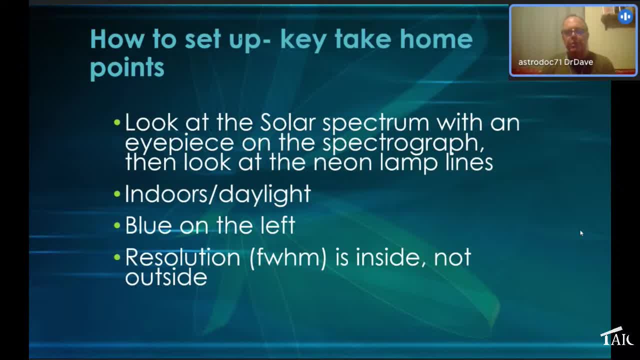 There's not nearly enough light coming in, Even at the zero order. there's no problem with that, And it's really cool to look at the. You just kind of scroll through. You start from the blue end and you go to the red end. 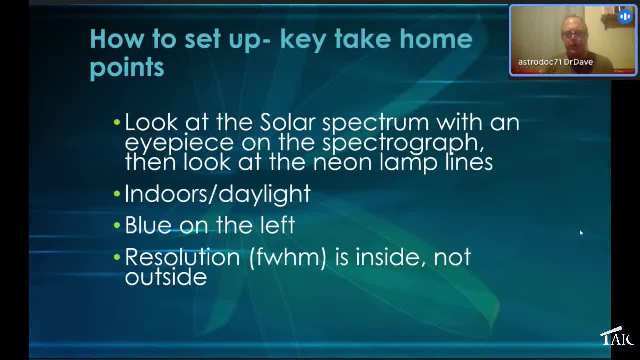 You see all the Fraunhofer lines And you get to the red end and the H-alpha just kind of becomes It's like three-dimensional. It's pretty crazy, But that tells you where H-alpha is on your, On your micrometer. 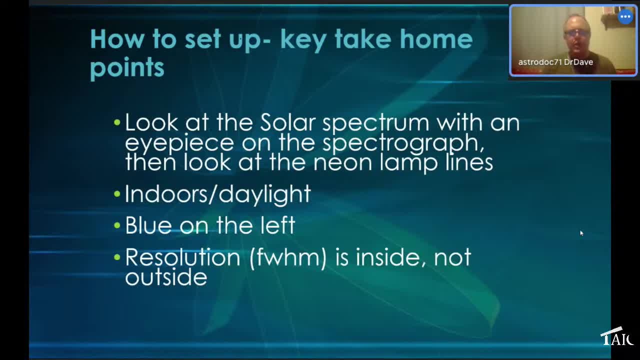 And then you can write down the numbers so you know exactly where it is. So once you do that, you cover the telescope. You can look at the neon lamp lines, which are thin red lines that you're going to see in your field. 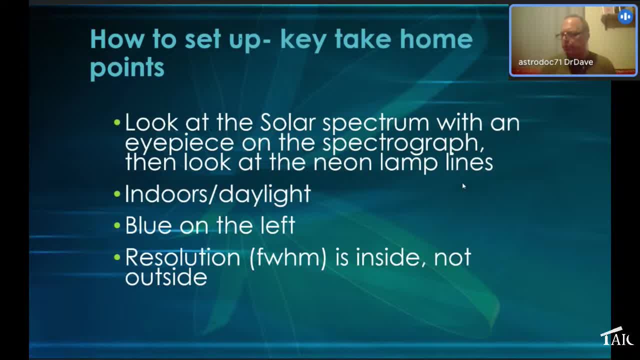 There's usually three, sometimes four of them. Most of your setup you're going to do indoors during the day And the convention in spectroscopy is that in your image you want to have blue design on the left side of your image. Red is on the right. 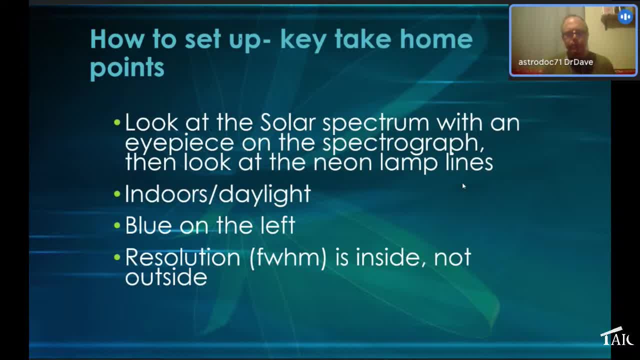 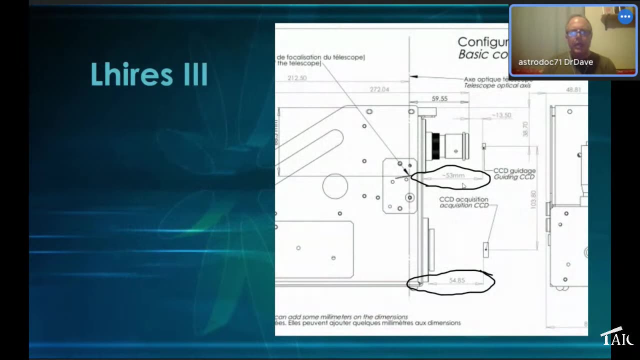 The other thing to remember because, as we pointed out before, your camera doesn't know anything about what's outside in the sky. It's just seeing the slit image and light coming through that. So that's where you're going to work on your resolution: by focusing that lens in the spectrum, in the spectrograph. 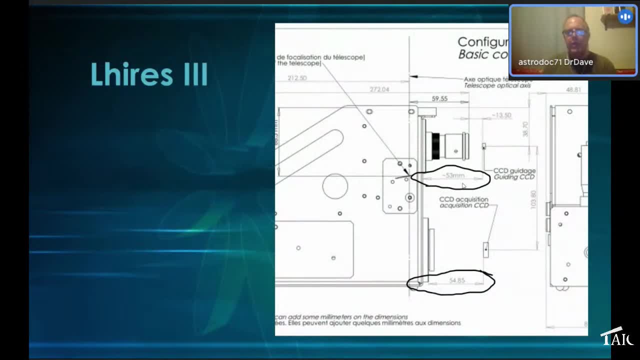 Sorry, This is a spec diagram of the Alhairas And these numbers are really important. Once you get these right, Once you adjust your camera spacing, you're going to be fine. So we all know about things like metal back distance and back focus and stuff. 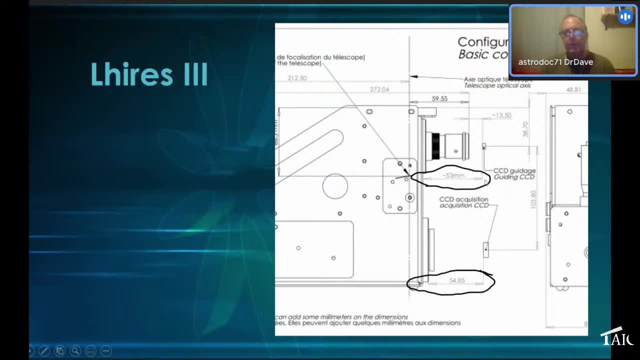 This really has to be accurate to. I would say really within a millimeter. If you do go with this spectrograph, the folks at Shell Yak are great. They'll help you set your camera equipment up and get you the right adapters so you get the spacing right. 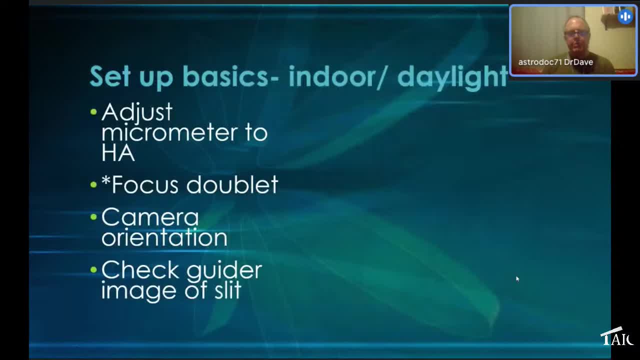 But that's really critical. So the basics are: you're going to adjust your micrometer like we discussed. Find your HA, Find your HA line. Your focus is a doublet. You've got to get your camera orientation right. So blue is on the left. 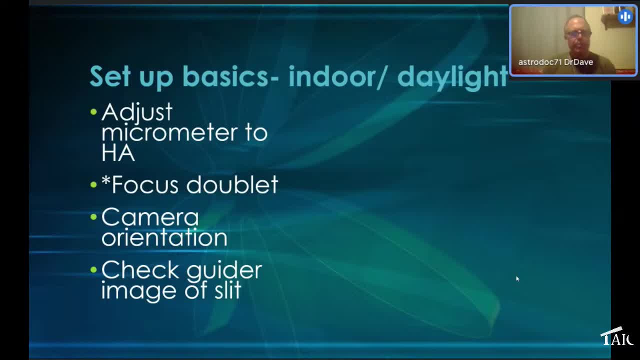 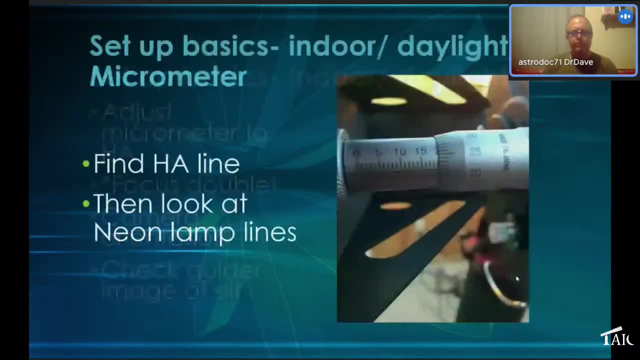 Red is on the right. I screwed that up when I first started and had it backwards, So it's easy to do. Then you want to check your guider image and make sure the image of the slit is correct. So, like we said, find your HA line. 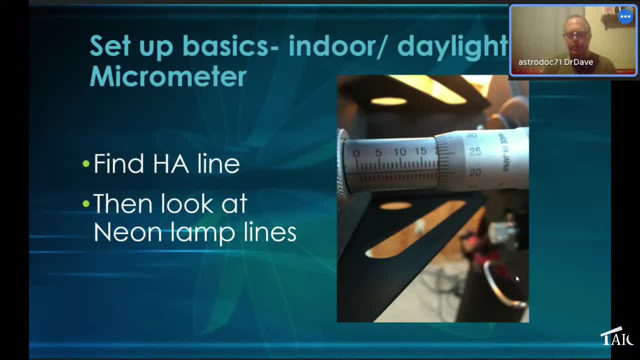 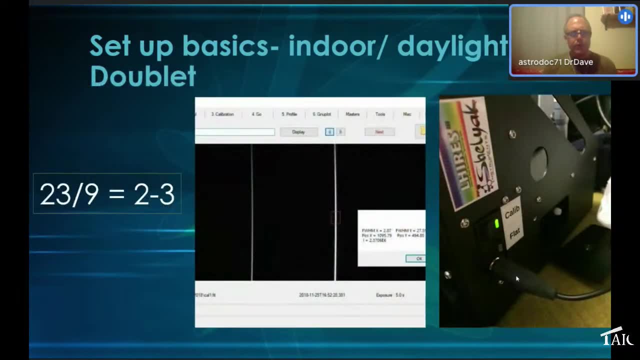 Look at your neon lamp lines, Make sure you see them. So that tells you that, yes, you are in the HA region. This is our old friend Nyquist, who's coming back to haunt us here. But it's actually a lot different, because we don't really care about the sky scene. 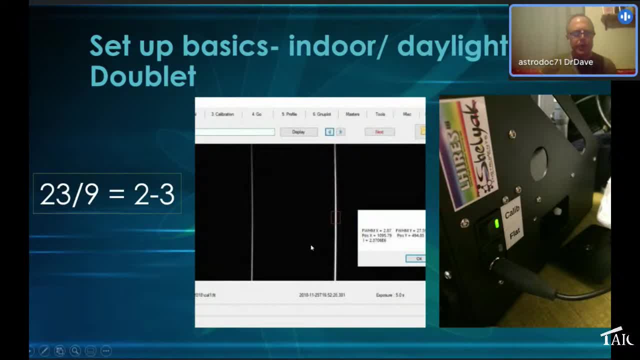 What we're interested in is that light coming through the slit. So that's 23 microns through that slit. And for myself, I'm using an attic camera. The pixels are Okay, Okay, Okay, So I'm using a camera that's like four microns, four and a half microns. 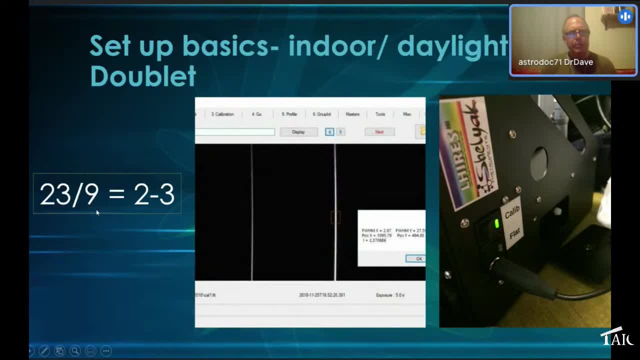 So I'm going to bin, And so the light coming through the slit is going to fall on two to three pixels with this relationship. So the nice thing is you have control over that every night And all you have to do is focus the lens inside the spectrograph. 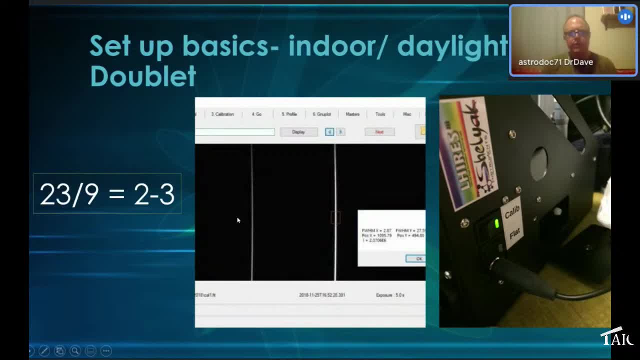 And what you do is you take an image of your lamp- And we'll talk about the ISIS program, which is really great- And what you do is you draw a little rectangle around your line here and you click on. there's a full width, half max button in the program and it tells you: okay, your X is well. in this case, we're good because we're 2.87.. 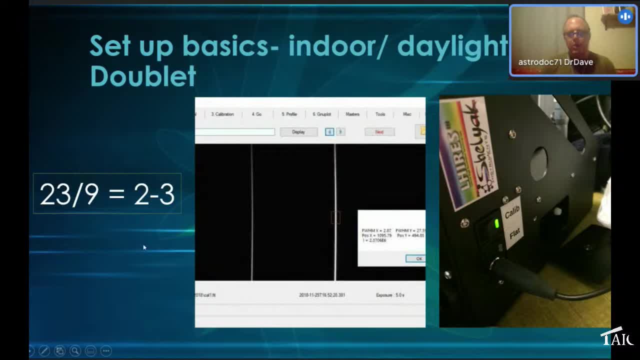 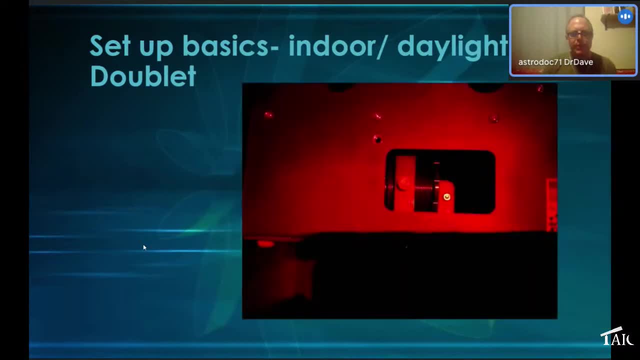 But let's say it's four or five or something like that, you're going to need to go back and just refocus it until you get that number right, And that might take about 15 minutes or so. This is an example of doing that. 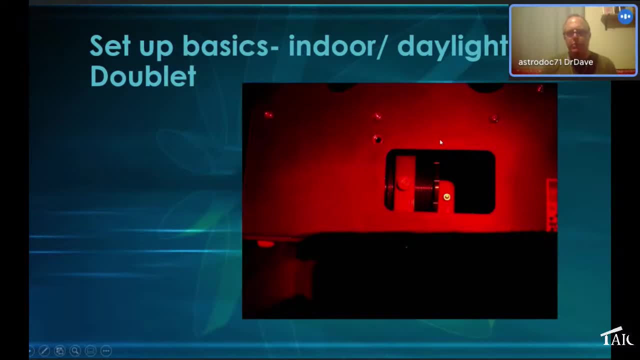 And you can see here, if you look out at the telescope, the doors of the side doors of the spectrograph are removed. here's your doublet ring. there's a little nylon ring you have to unscrew that. you got to undo, you got to take off both doors to get it, to get it right so you can turn the ring easily. 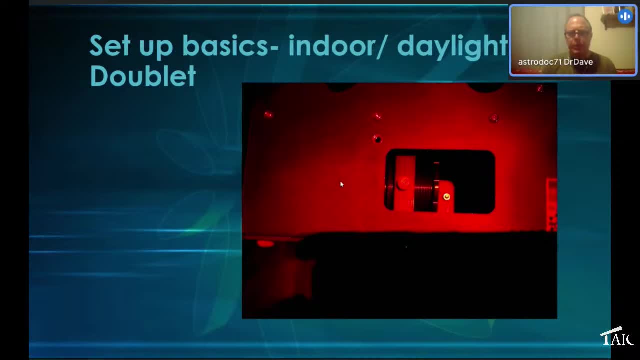 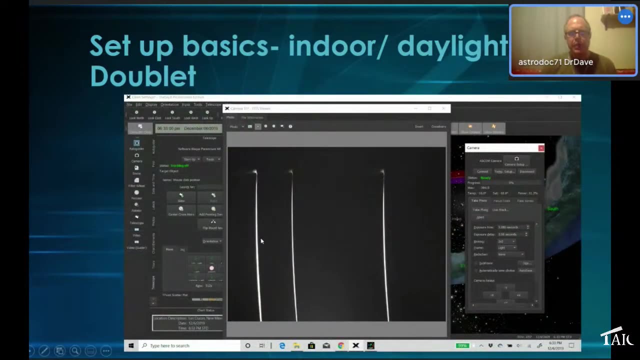 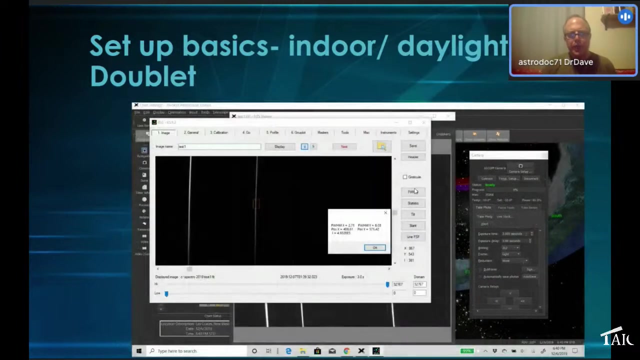 And then, when you're done, you just tighten everything up. this is a image of your calibration lamp. here's your three lines that you need to be able to see And notice that they're a little tight, Okay, And notice that they're a little curved. that's because you got that 10-degree tilt in the spectrographs, with the light coming back toward the camera. but the good news is, your software is going to cure all that. you don't even have to worry about it. 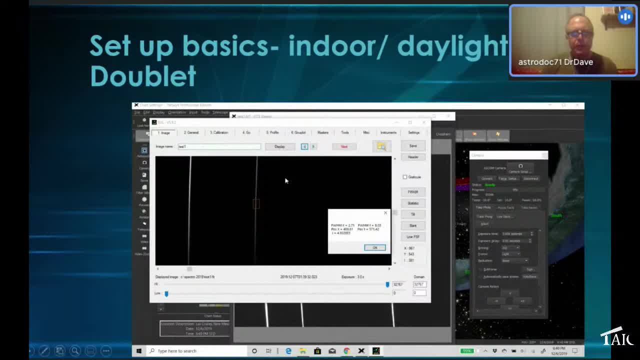 So this is what I mean with the lamp image. so you go in your ICES program and you here's your image tab and you just draw a little box around. this is the center line of the three, or not center, but it's the middle one. 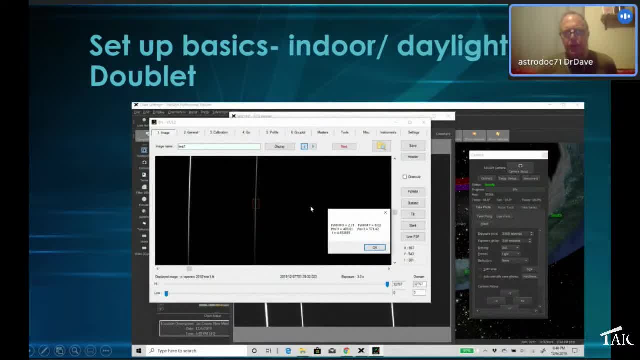 Okay, Because that's the one that's closest to the center of your sensor. So then you come over to this full width, half max button, click on that and, okay, we're good here. so that's what you're going to do to get that focus. 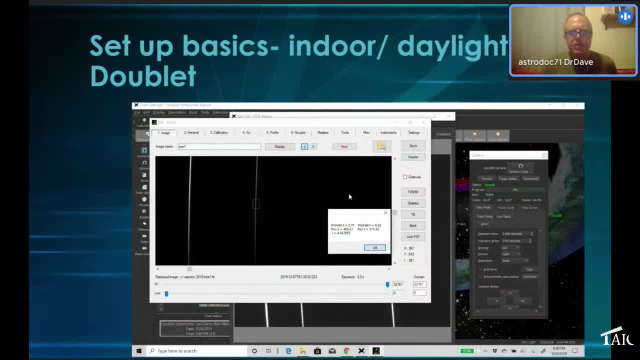 You only have to do it once and it's good to practice it indoors, but, like with our regular cameras, we have to refocus because the temperature changes. so you're going to want to do that at the telescope. This is another way you can check your camera orientation. 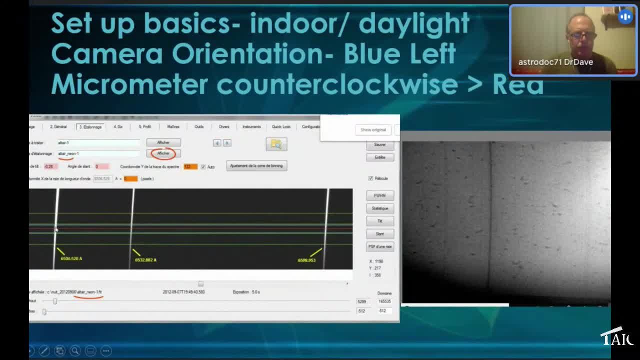 So again, you got your three lines. you got to do that. So you have three lamp lines here: 6506 on the blue end and 6598 on the red end. so that is correct. When I first did this, these were flipped. I had the two on the right and the one single one was on the left. so that was not correct and that was easy to recognize and I fixed that. 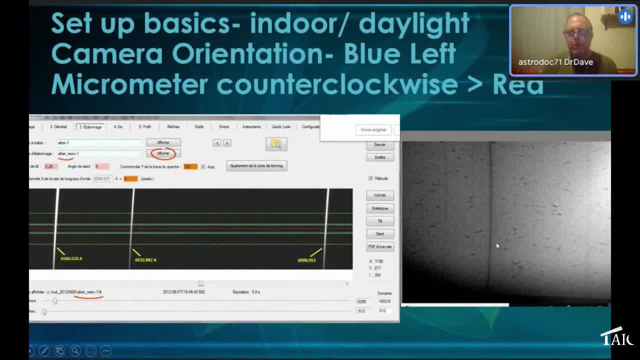 Here is the HA line. so what you do is you go out during the day, point your scope at a random part of the sky and you get the reflected spectrum of the sun. So here's the HA line. So here's your HA line, and you turn your micrometer counterclockwise and that will move you into the red portion of the spectrum. 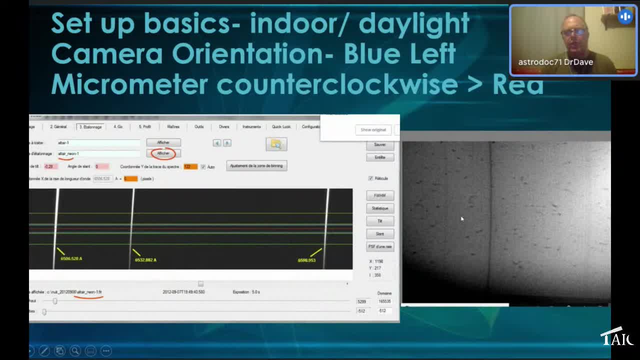 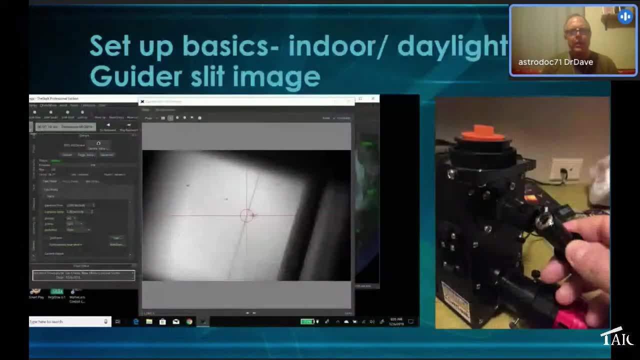 So you're going to want to see this line move to the left, so it goes the other way. your camera is upside down, So that's another clue that you can use. This is your guide, or slit image. Okay, so this is pretty ugly, and if one of my mentors is watching this right now, he's probably cringing. 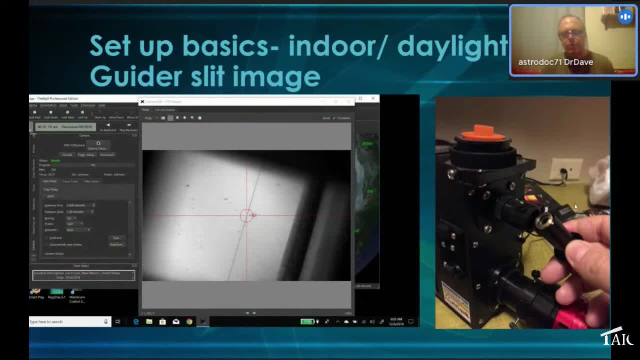 So this is pretty ugly, and if one of my mentors is watching this right now, he's probably cringing. But this was about two weeks before the conference, so I was not about to go into the spectrograph and monkey around with it. 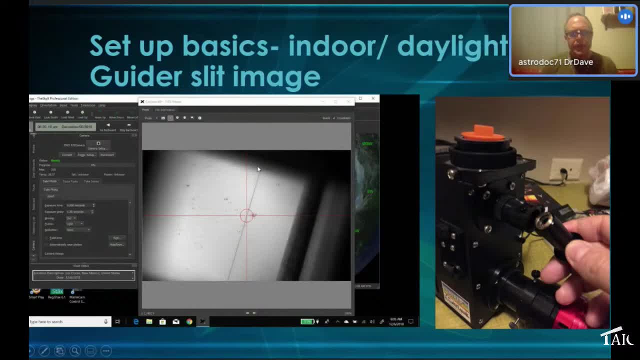 I was able to confirm that this slit is about two pixels, which is what you want. It goes through the crosshair so I can find it at night, but I left this the way it is. I promised that I'd fix this and this is not the way it looks now, but I left it for this talk, because here you can see the edge of the …. 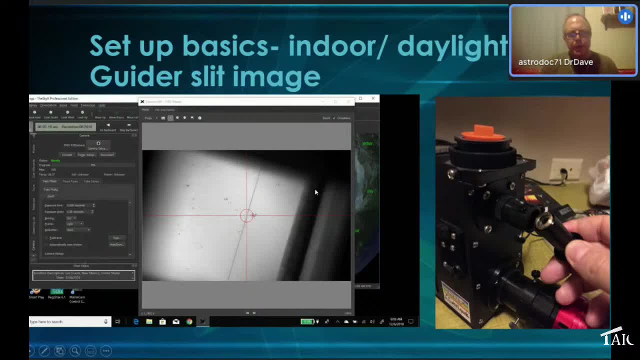 of the of the slit mirror. okay, so this totally worked for my setup, doing it manually. but to be fair, if you are going to do a little more automation, you're going to do plate solving and kind of the same routine that we do for imaging. you know this is going to have to be. 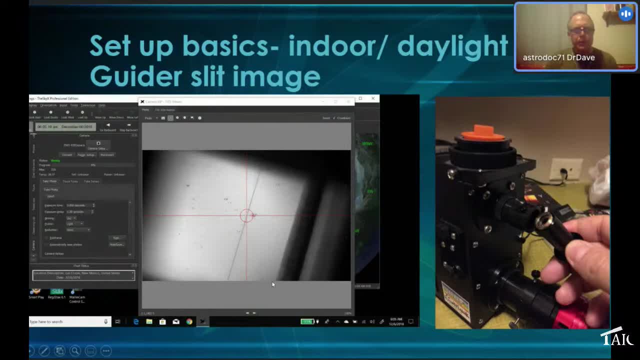 improved where it lines up with your, with your, your guide or better, but the main thing is you want this slit image to be about two pixels, and the way that happens is your distance between the spectrograph and the guider is, in that, one millimeter, not more than one millimeter off. 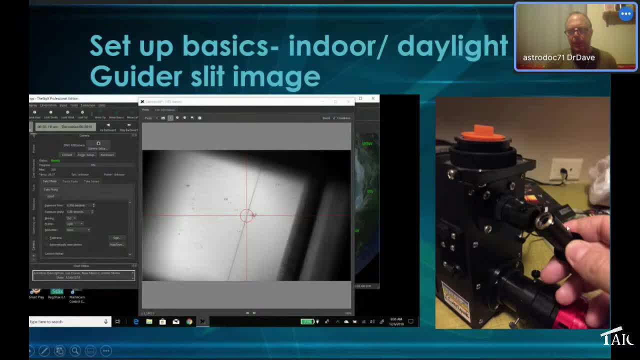 of that back back a distance that you need to get right. this is a. this is the guide port here. it's pretty small, it's as weird, it's like a seamount, but you can find adapters for that. no, without too much, too much trouble. so at the telescope you're going to refocus. 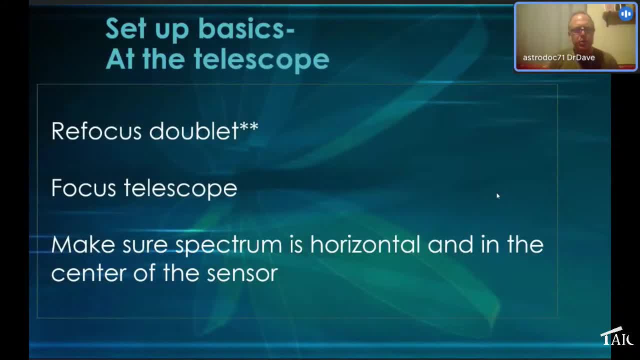 the doublet because the temperature is going to change. you want to do that one time. you're going to focus the telescope. now I just focus with the knob on the primary mirror. that's all I do. um and uh. that that works great. and you want to make sure the spectrum is horizontal and in the 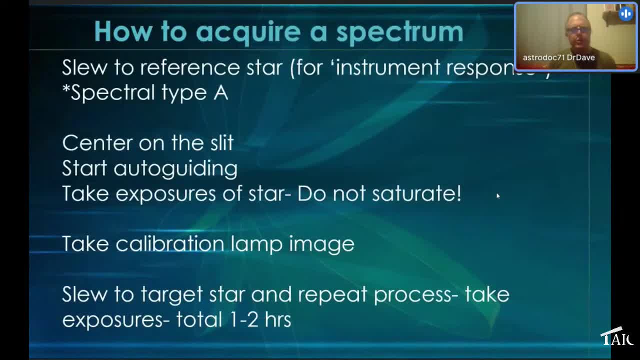 center your workflow. what you're going to do is: first you got to slew to a ref, what's called a reference star. so what happens is your, your equipment has a certain spectral sensitivity. it's going to be different for every Observer- and you want to correct that and your final spectrum. 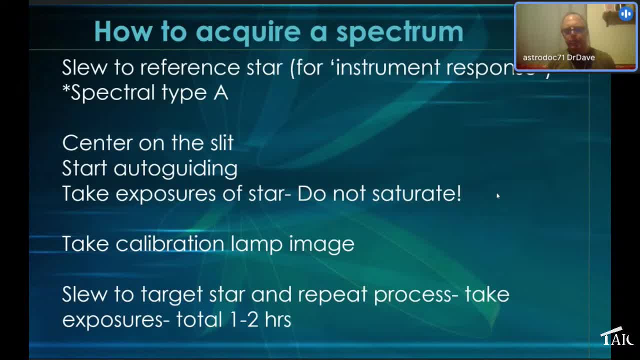 or account for that. so you're going to take your, your reference star spectrum, you're going to compare that to a database of professional spectra and that's going to be used to calculate what's known as your instrument response, which gets figured into the final to the final target spectrum. 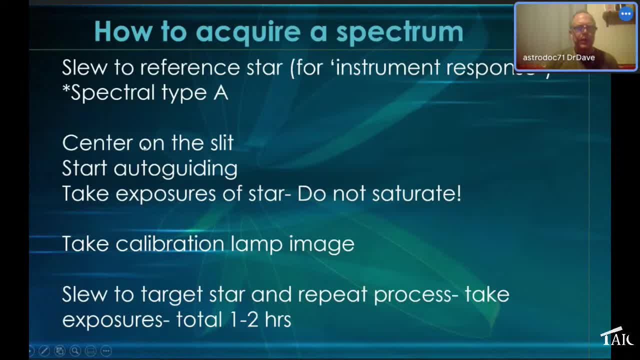 um, things we're used to. obviously you want to Center your target. you Center the star on the slit. you start auto guiding. you don't want to oversaturate, uh. then you take your calibration lamp image. then you go to your target star, uh. repeat the process and at the end you take your 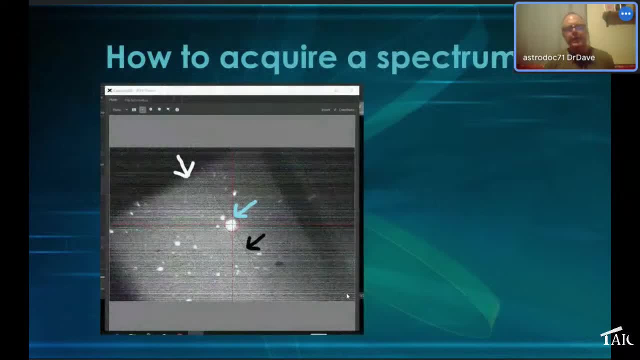 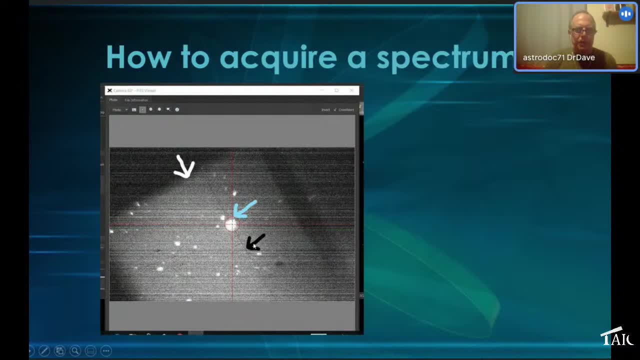 black arrow is actually the center of the sensor. that I that I figured out initially. now it's more like here because I adjusted the mirror. but um, but this worked. I mean, as long as I knew where this was, I would just jog the, the uh, move the star down to about this location and just take a test. 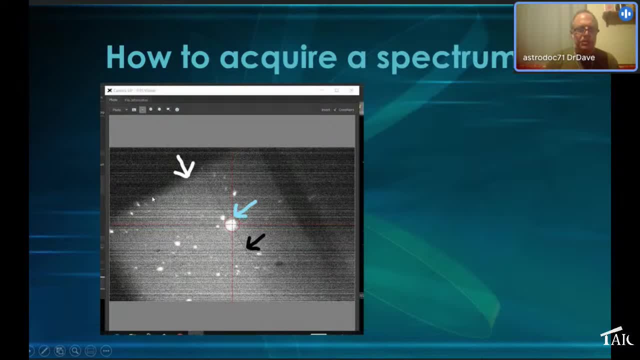 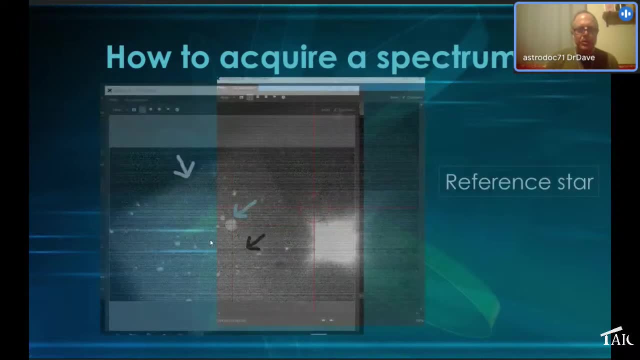 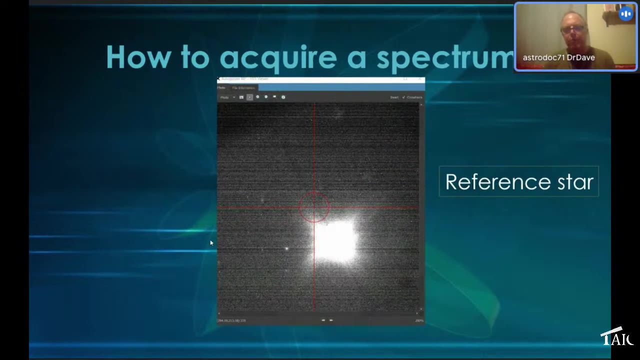 image and make sure that it was centered. and you can see this is a pretty big uh guider field and you have a bunch of guide stars that you could use, so you gotta. so that really does help if you have a large guide field that you can take advantage of. this is an example of a reference star. this is a super bright. this is 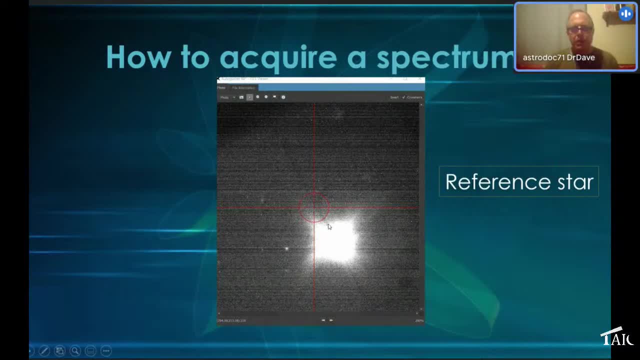 probably Vega or out there or one of those. and the thing is, here the eye is an is an excellent judge of when and, in my opinion, when this is centered, because when you do that, when it's you're going to see this line is going to darken, the the slit line is going to darken, or you could. 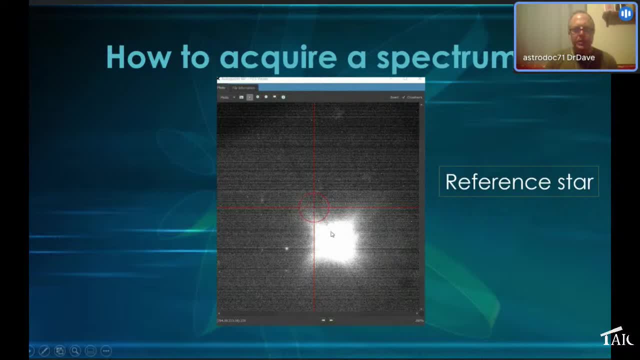 say that the star dims, but what your eye sees is that this all of a sudden gets dark because the flux of the star is fine, is uh, is is dropping as the light is the maximum light that can get through the slit, is is going through it. so then you know, you're good, you got a nice little guide star here. 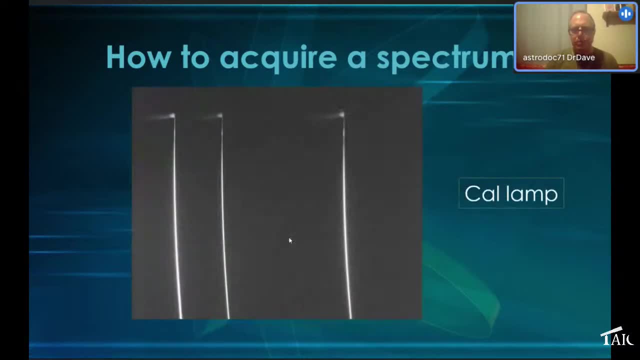 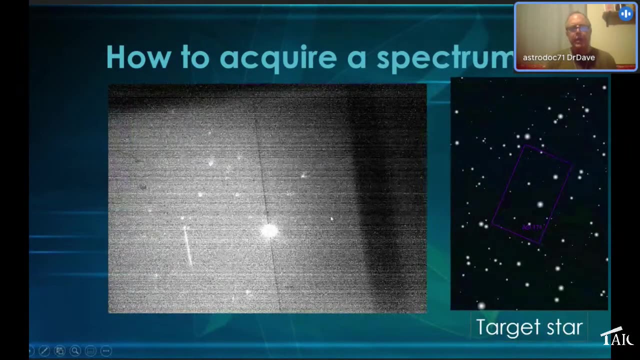 that you can use and you're all set. this is your lamp image that we talked about before. um, this is your target star and since I do this manually, um, uh, you know, sometimes your, your pointing may not be that perfect, and I find that, if you use your your uh field of view, uh, if you. 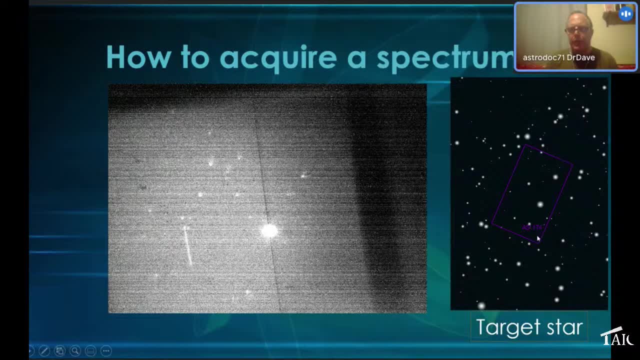 have a field of view indicator that shows what you're, what you should be looking at. you can see the pattern of stars that you should be seeing. this is not related to what you're seeing here now, which is just an example of something that can help you. now you're going to be looking at mainly. 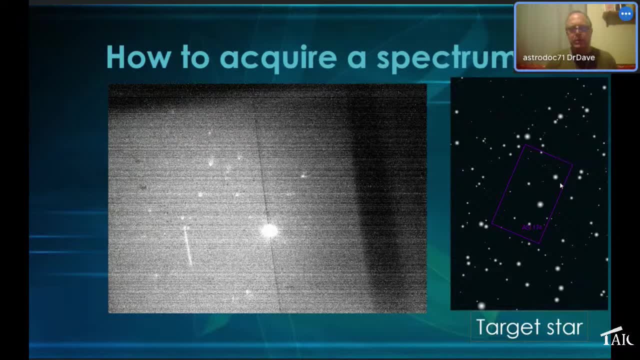 stars that are. you know, they're pretty bright. I mean, they're going to be like, uh, six magnitude or so, and they're going to be the brightest star in the field by far, so you're going to be able to find it pretty easily. um so, how do you process a spectrum? this is the Isis program. it's written by: 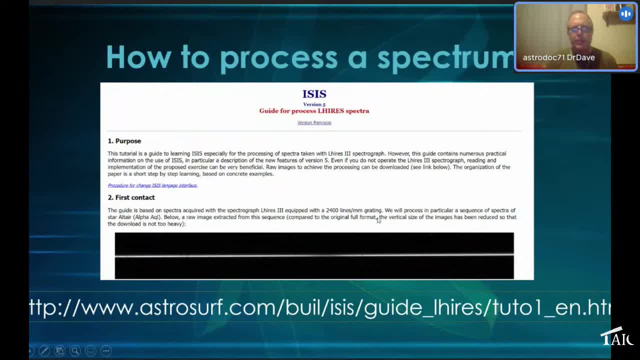 uh, Christian wheel and uh, it's a. it's an excellent program because it takes all uh it. it automates just about everything, um, and it's it's very simple to use. this is a one-page tutorial. that's all you need. it explains everything, um, so you can go to this uh web page and and get all that information. 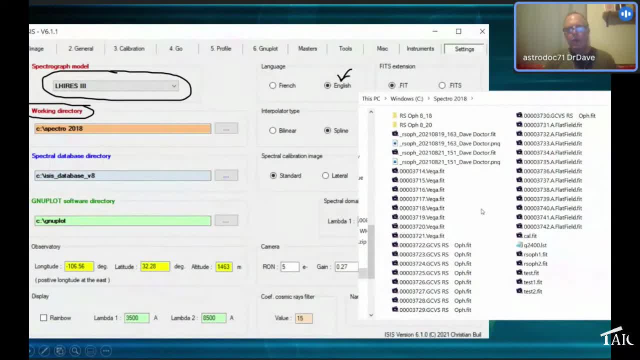 uh, the key thing is: uh, you got it. you you want to put a or set up a folder. let the program knows where to find everything. and really it's just one folder, anywhere, um, um, and you put everything in there. you put your flats, your lights, your, your, your, your darks. you don't have to organize them. 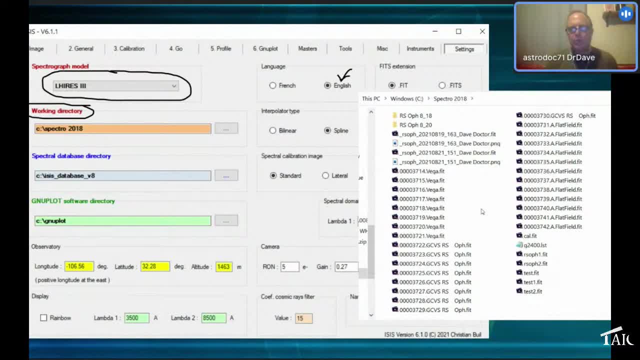 in any way. if you don't want to, it can be, you know, like a closet. you just throw all your clothes in there. they don't have to be folded, they don't have to be organized in any in any way, shape or form. they just have to know that they're there. so you set. 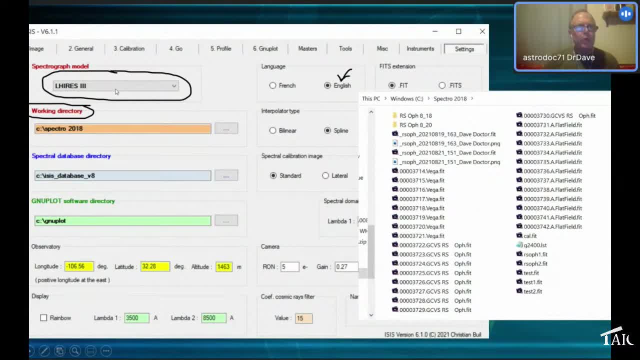 that up here in this working directory. uh, when you go to the spectrograph model, this is really cool because, uh, if you click on a high res, it already it tells the program: okay, I'm using the neon lamp lines, you know 6506, you know the other two, and and it already tells the program. that's how you're. 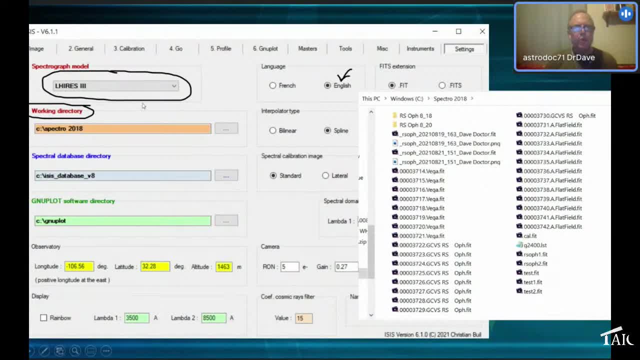 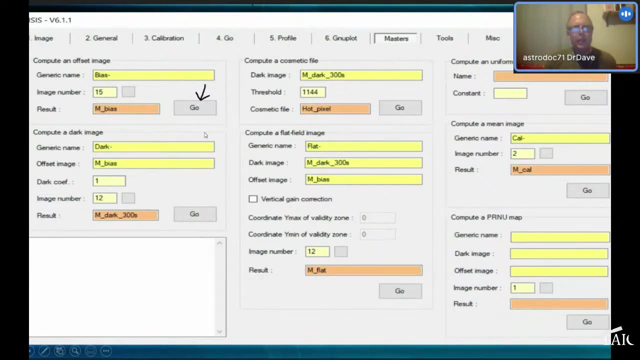 going to calibrate your spectrum, so you don't really have to do much more than that. and, of course, if you need the program in English, you click on that. you reboot it, uh, and, and you should be good there. so, uh, you go to your master's tab, you um, uh, everything you're doing here is clicking on a. 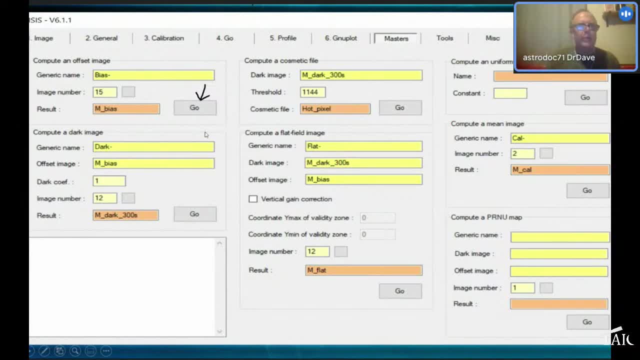 go button. that's that's how you uh. uh, that's how you get through this, uh. so you uh call, you, name your, your master files, uh, however you want to, um, and you click on go go and it produces a master file, um with this name and you get all your uh, your files, uh, in the same 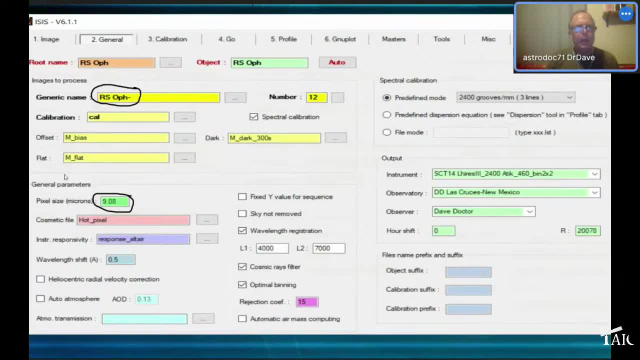 spot, um, and it knows where to find them. uh, then you go to your general tab and, and the really the key thing is you. you got to name your object, uh, uh, and put a little dat, a little hyphen next to it, otherwise it won't recognize it. but that's all you need to to know. there it tells you all. 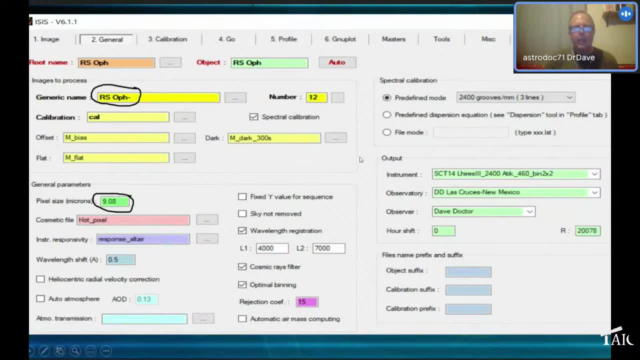 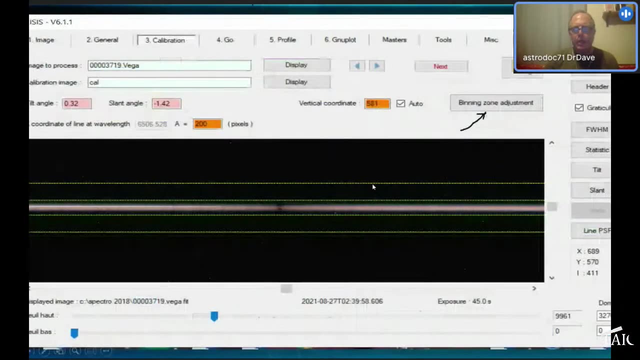 these things. you know your location. how to set that up in the tutorial takes maybe about uh, you know, once you set it up, which is about maybe 15, 20 minutes, um, you, you can run through this uh in a few minutes every time. you, you, you do a spectrum, uh, you go to your calibration uh page and, um, what you're going to do is uh, 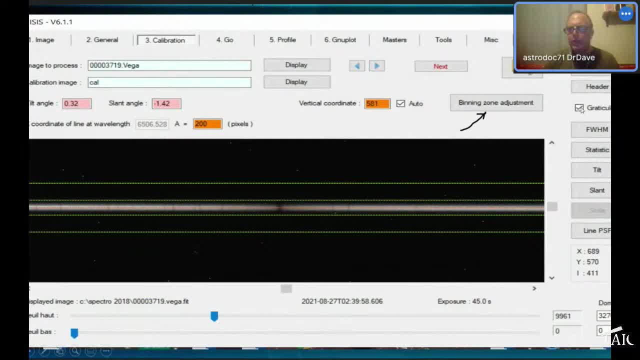 you're going to use this grid here. this is uh called the graticule, and and you can click on and off of that. so, uh, you want to get this, uh, these inner lines, as close to your uh spectrum as you can to eliminate the background noise. that's why, as you can see, you're going to need to make this pretty. 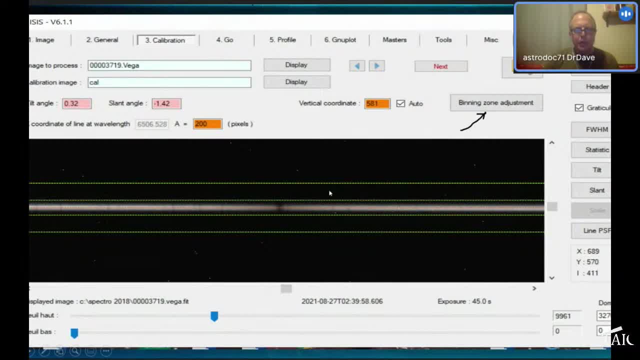 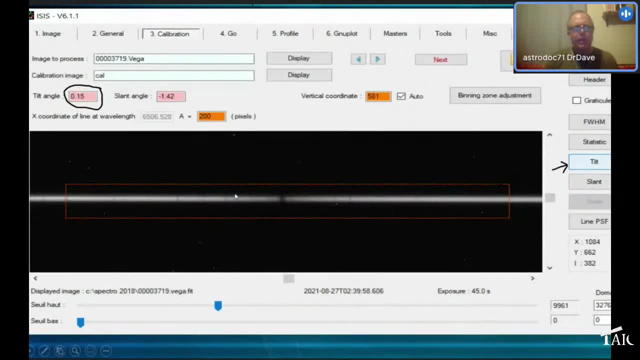 horizontal, because if you have a more of a diagonal one, you're going to need to spread these out, and that's going to include a lot more noise there. next, you're going to figure out the, the tilt of your spectrum, how far off of horizontal it is. that's pretty simple too. you draw this box. 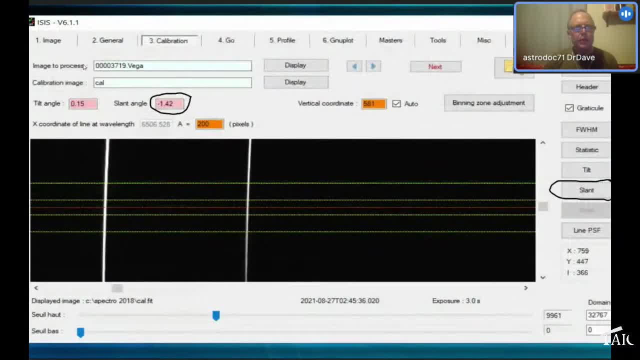 it. you're done with that. next you go to your calibration image and you're going to calculate the slant, as we mentioned. that has that curved. it's a curve, a little bit of a curve to it and you want to correct that. so you draw a little box around here, click on slant, calculates that. 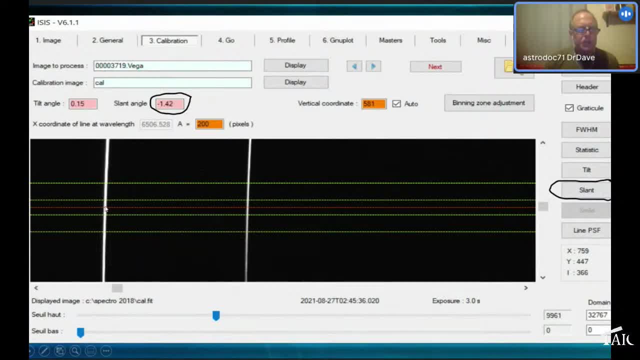 and then the key step here is: you're going to, on this line, which is the 6506 line, that's the furthest away, furthest in the blue, you're going to double click here and that's going to tell: uh, the, the software. okay, this wavelength is at pixel 200, so you're going to do that. 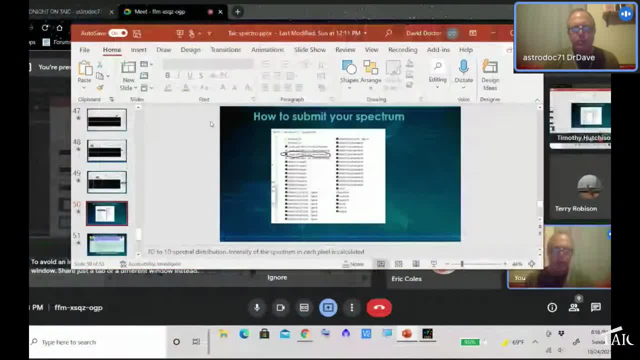 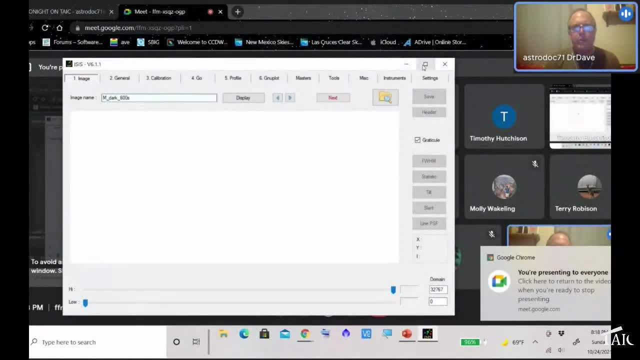 what i want to do is just: we're almost done. i'm just going to run through this processing here for for two minutes, just to kind of give you a sense of that. so we are going to process. so we are going to process- uh. spectrum of vega. 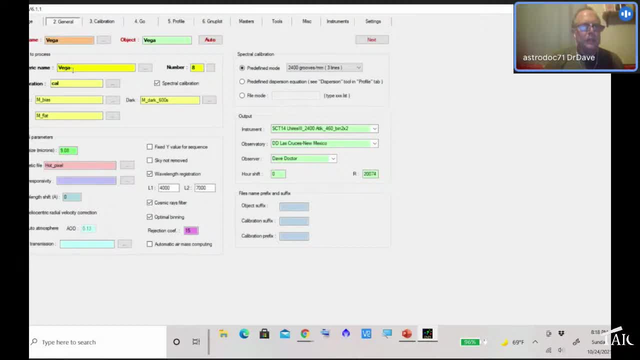 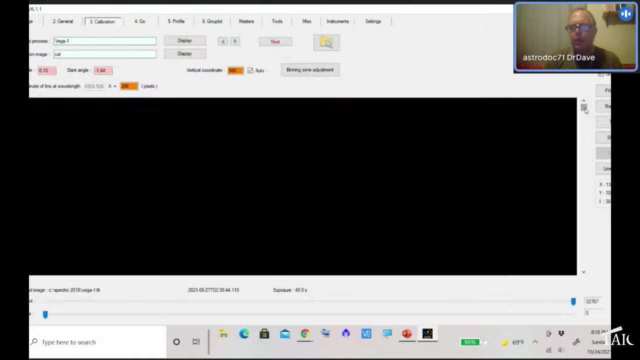 and uh, notice, i have the uh star has the dash line in it and it knows exactly. okay, you've got eight light frames and if you click on this box, it confirms that it's eight. um, so next you go to your calibration page. so i'm gonna move this down to the center here. here's your, your grid, and oh, i don't. 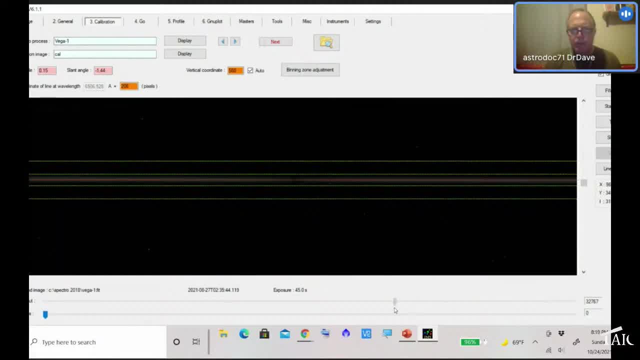 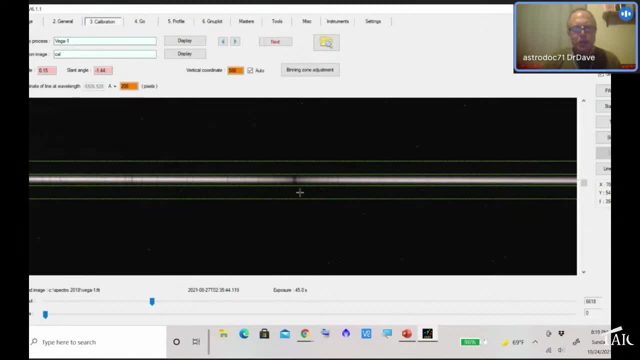 see any spectrum. well, that's because you've got to take this slider and you move it here and presto, there's your, your spectrum. so the next thing you do is you're going to center it. you just double click in the center there. the next thing you do is you take the grid off and you 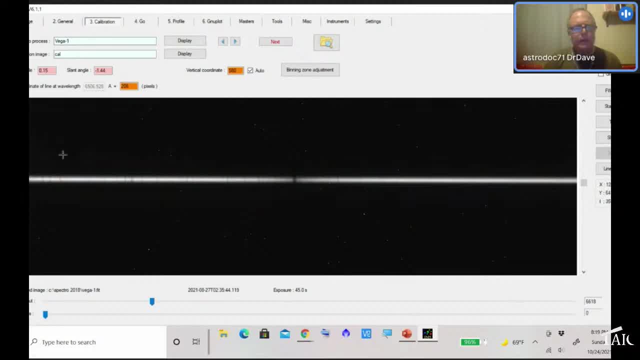 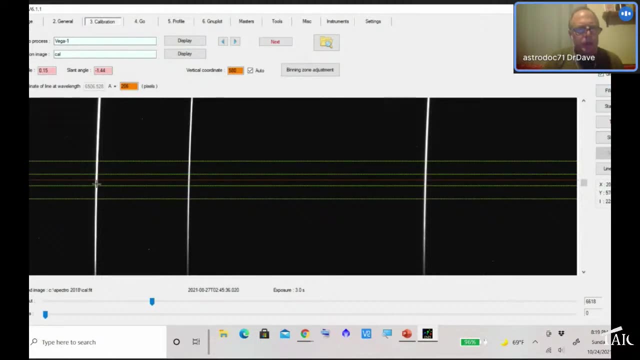 draw your box and you, you uh, calculate your tilt. and the next thing you do is go to your calibration uh file and you're going to set your. your wavelength here on the edge tells you're at 204. you're going to draw your box around the middle line, calculate your slant. puts that in here. okay. 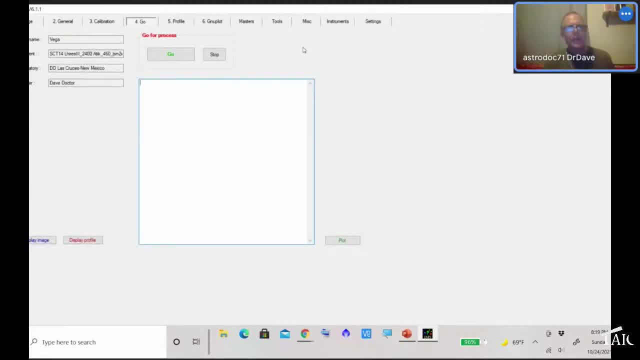 now you set everything up. so what do you do when you want to process your spectrum? well, you click on go and in a few, about 10 seconds, your spectrum is processed, and that's it. well, of course, now okay, it's a. what it does is it takes a. 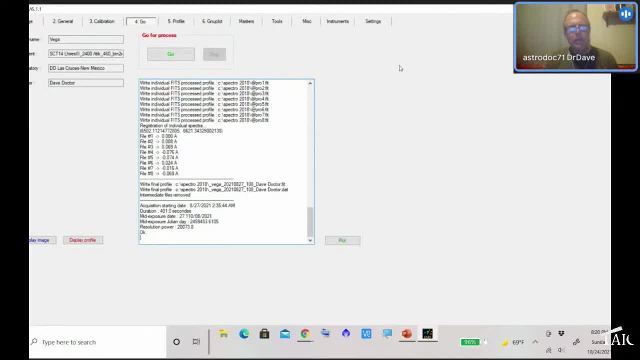 two-dimensional uh spectrum, okay, and it converts it to a a one-dimensional uh uh. it's almost like a data file, because it's what it's doing is it's assigning intensities to the spectrum, to each pixel, but there is a profile that you can see, because what you do is you just 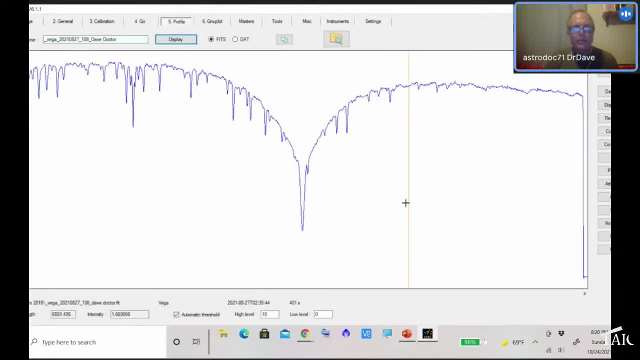 click on this profile and display, and there it is. so um, and here's your, that is 65, 62.5. so that's how you process the spectrum. now, this was your reference star and you're going to go through that again after you figure out your instrument response. but that's another. let's say: 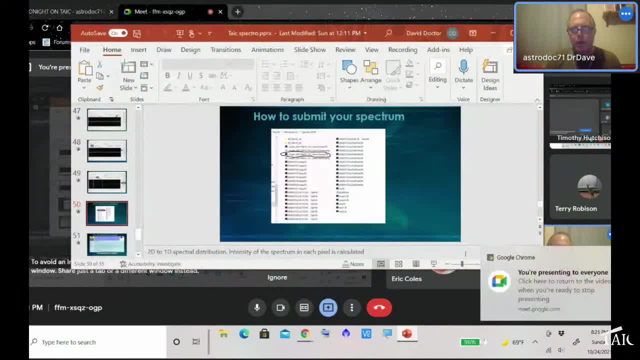 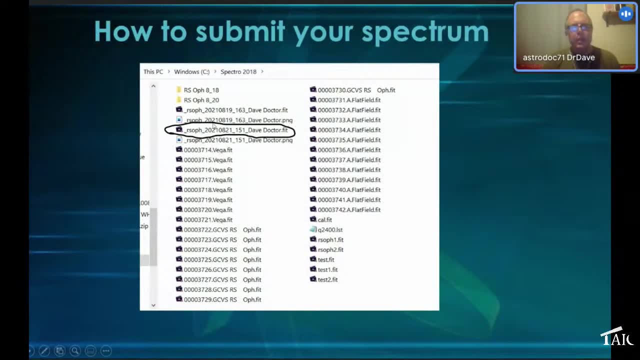 10 minutes of that. so, um, uh, now that you've done that, how do you submit it? you're going to look for this 14 kilobyte fit file- okay, that it's not the two-dimensional line profile. you're going to send this to your, to your sources, and. 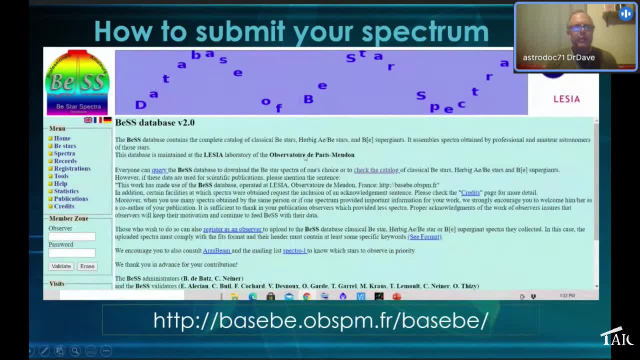 you're probably going to start with this. this is the best, best database- uh, it's a bit probably the biggest one in the world for be stars, and this is great because when you submit your spectrum, you'll get you get somebody to tell you: okay, it looks fine. 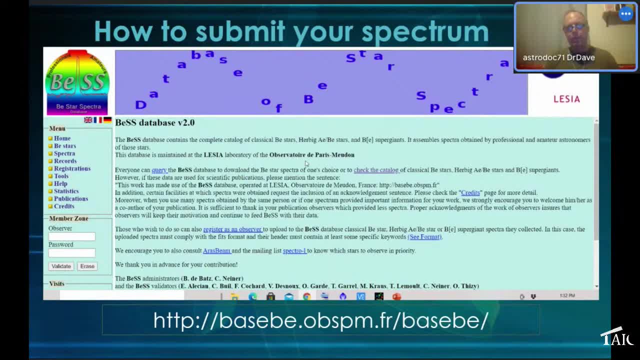 it's accepted. but if it's not accepted, we'll tell you what's wrong with it, you know. they'll give you hints on how to correct it and what to do. and that's a great learning experience and uh, and, and it's a, it's great um, uh, to help you, uh. 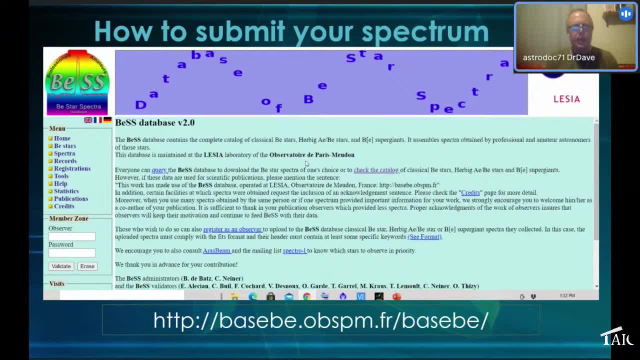 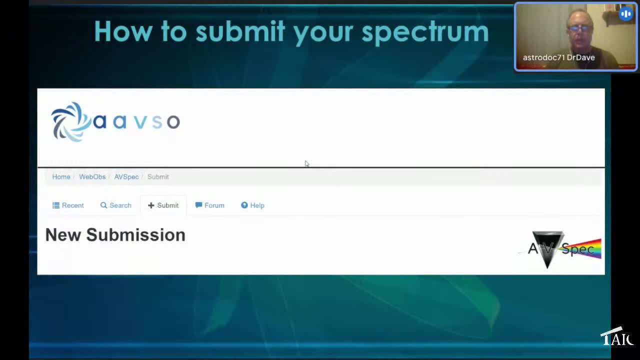 are at the at the spectrum acquisition side, the aavsos we talked about. this is a great resource and you can do the same thing. they have a spectral database. you can submit any spectrum you want there. it's also great because they have a, a forum there, the great people. they answer all. 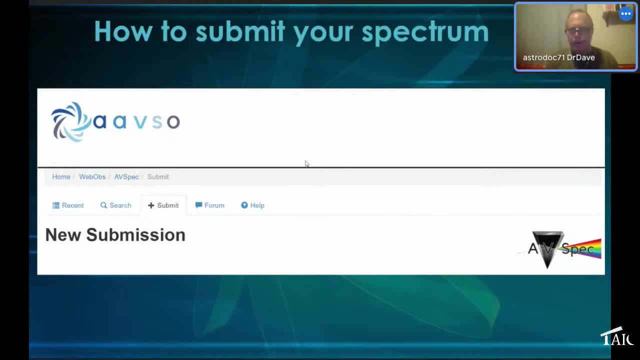 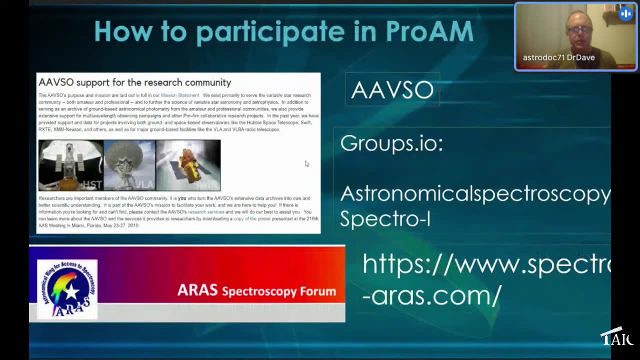 your questions, regardless of how simple they might be. so you definitely will want to do that. so pro-am collaboration, that's a big thing with the high-res spectroscopy, but really what happens is not you seek them, it's they're. they're going to, they're going to seek you out. the aavso is the. 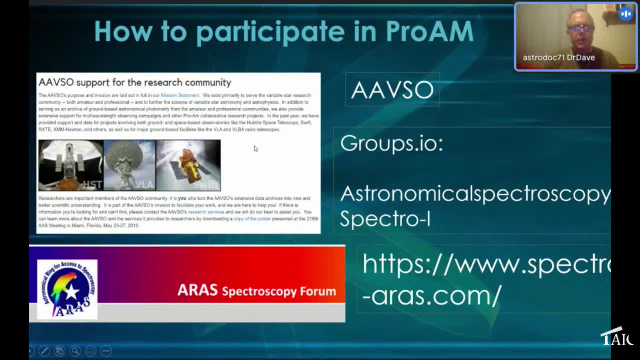 resource for even the nasa telescopes. they really need people to support. they need ground-based support on their research all the time, so there's there's never a shortage of of projects to do. you can also join these groups here. astronomical spectroscopy is great. spectro l. 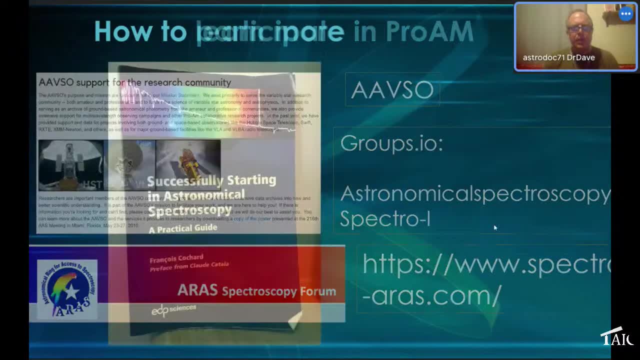 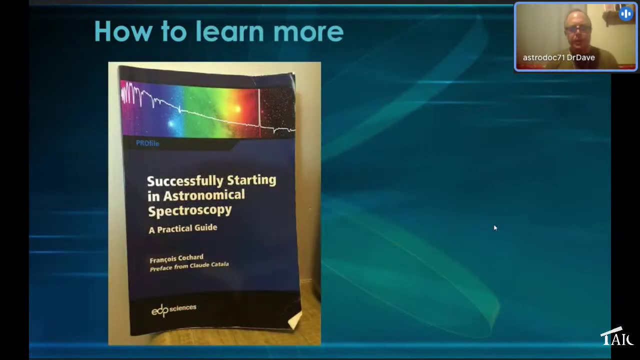 and eris is a spectroscopy group in france. if you want to learn more, this is the book to get, written by francois cochard, and it's it's indispensable kind of goes through some of the stuff that i presented in much more detail, so you definitely want to want to do that. 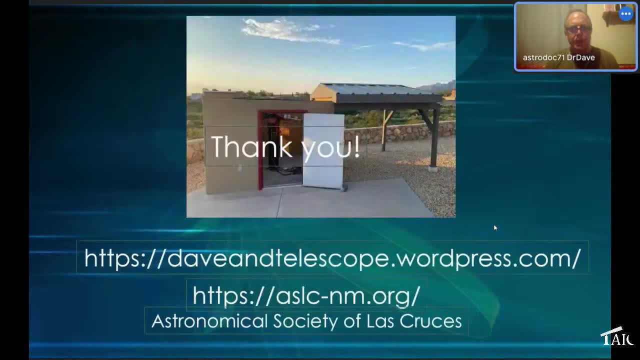 and uh, that's pretty much. uh, that's pretty much all i got. um, if if you want to find me, you can uh find me on dave and telescope at wordpress dot wordpress. that's my blog. i'm also an active member of the astronomical society of las cruces, which one of you mentioned was founded by clyde. 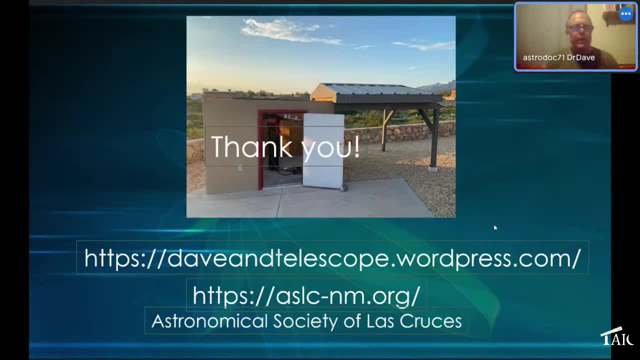 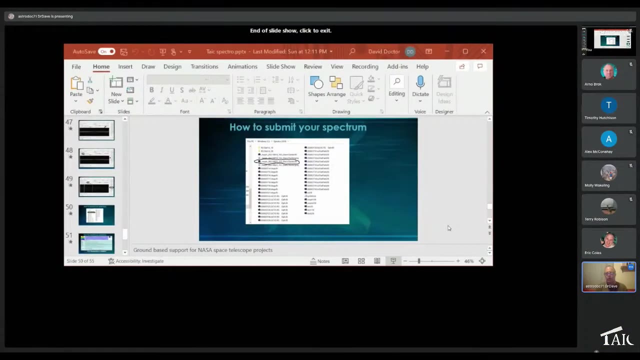 tombaugh and has a rich history of uh education and public outreach. if you're in southern new mexico, uh, you need to check us out. we do a lot of cool things there. um, thanks a lot and, uh, i'll take any questions you have. i don't see any questions in the chat, but i have a couple of questions. 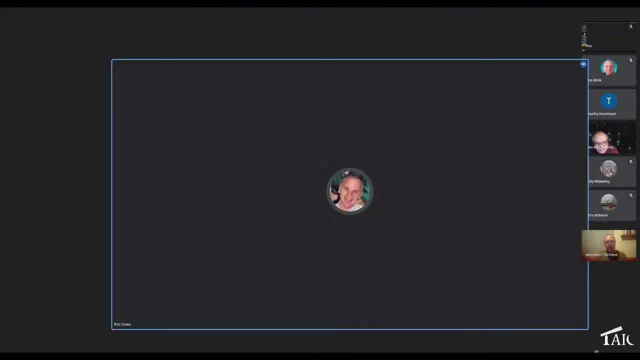 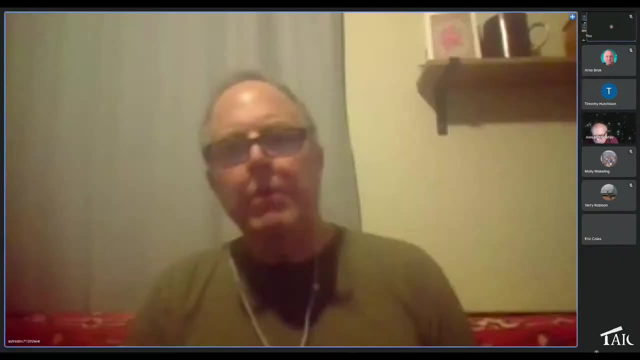 so the reason that your data is so valuable is that the professional astronomers just have difficulty getting telescope pain. uh, yeah, well, that's certainly uh, that that's got to be a a part of it. i mean, uh, you know, they have to apply for telescope time- what a year or so in advance. 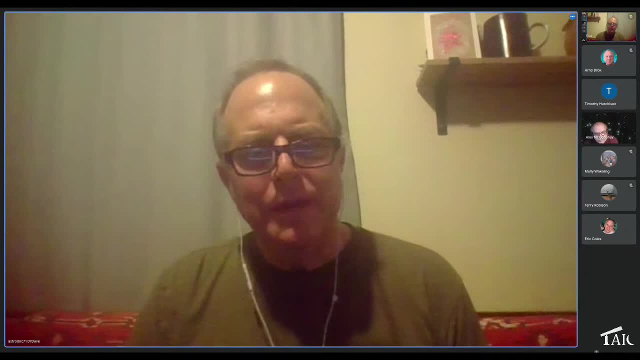 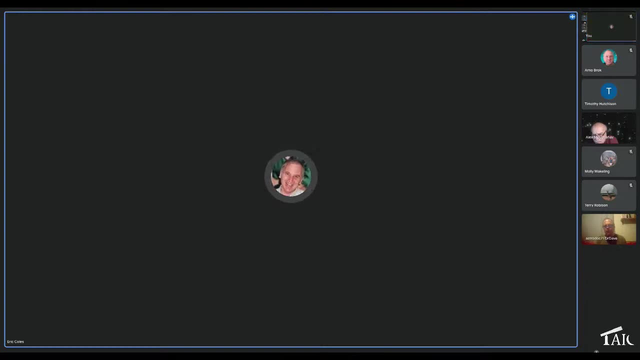 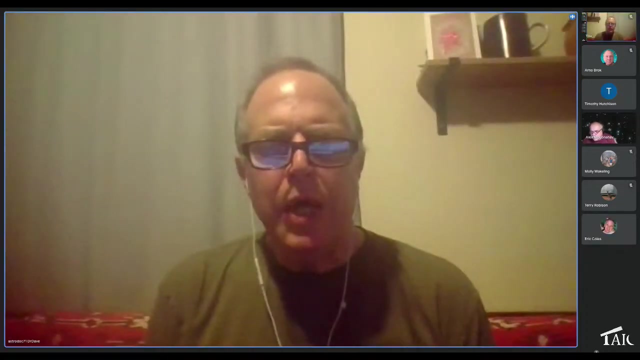 they get maybe a night or two and uh, that's it, and then it may be cloudy, who knows? so, yeah, if, if what's one, someone wanted to go into this, uh, what would be the cost of just the spectral equipment? so, uh, okay, so the ohio as the spectrograph? uh, new, um, i'm thinking, is uh, 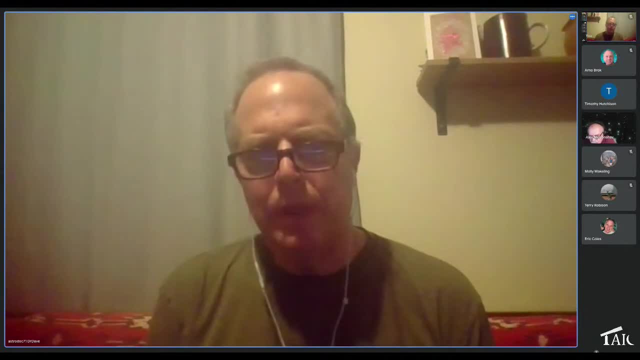 it's probably uh two, two to three thousand, but there are a lot of used ones out there now that you can get for under a thousand. and there are also, uh probably kits, because this started out- the, the eljira- started out as a kit that you could put together before they, you know, made it a compact. 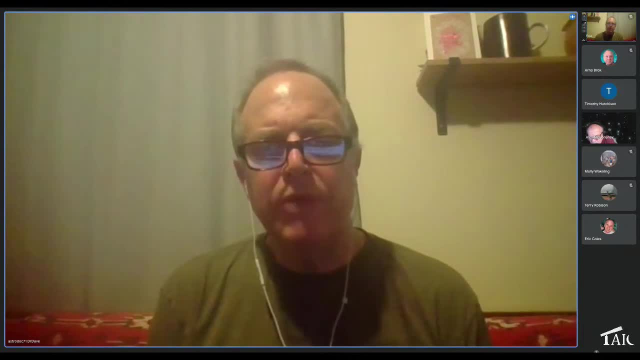 unit. so there are other less expensive options and, as i mentioned before, there are groups that are are 3d printing these things. so you know i'm sure there are uh avenues that people can take that are less costly. that's really your main, your main expense. i mean ideally you could use. 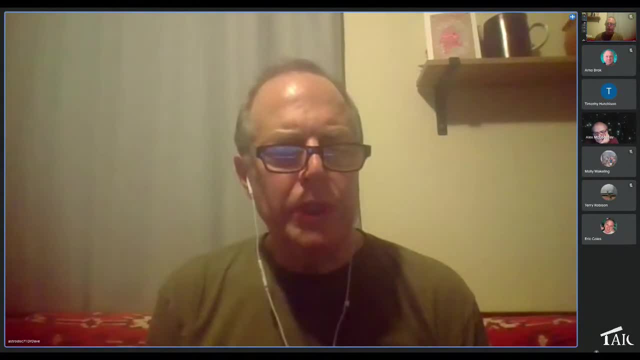 a telescope that you already have. but the telescopes that you need, um, you know, you certainly could get, uh, i think, pretty easily. so when they say you 3d print, you're not printing the gradient, uh, the grading. i'm sorry, oh, the grading. yeah, you're not printing that. no, 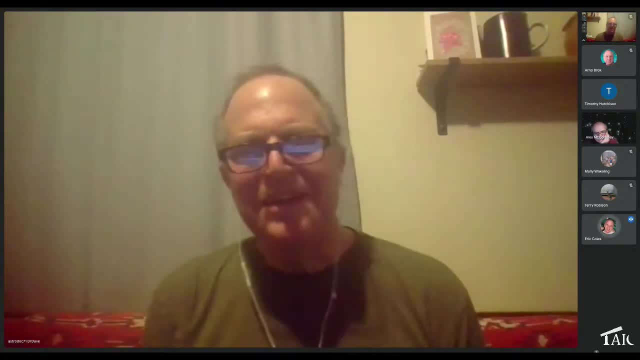 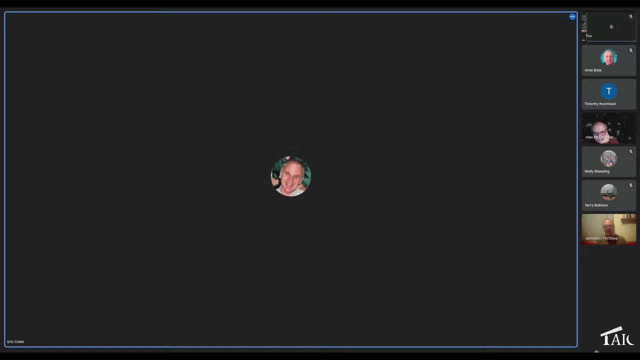 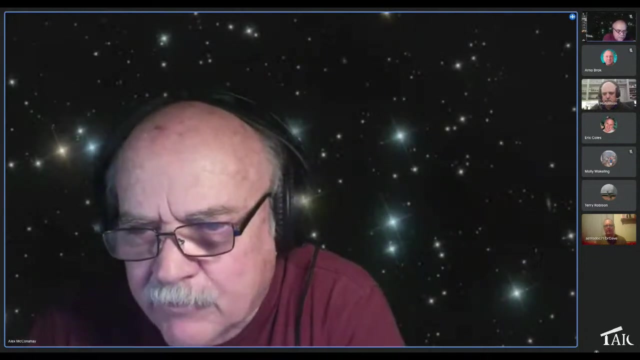 no, i, i mean, i don't imagine that you're printing that. i don't imagine you're printing a gradient. they're not not printing the grading. no, i, i don't. five thousand lines per right. right, um, eric, if you could give me a second here. uh, lance man. one says he pointed out relatively early on. 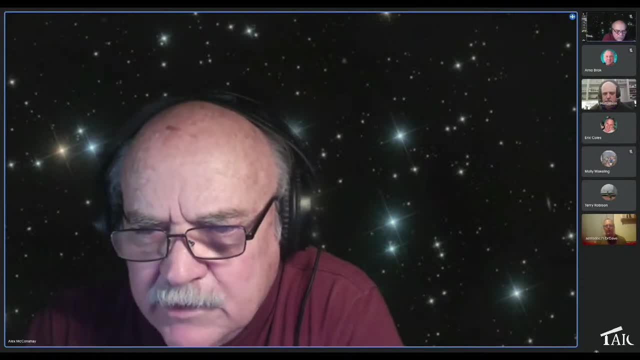 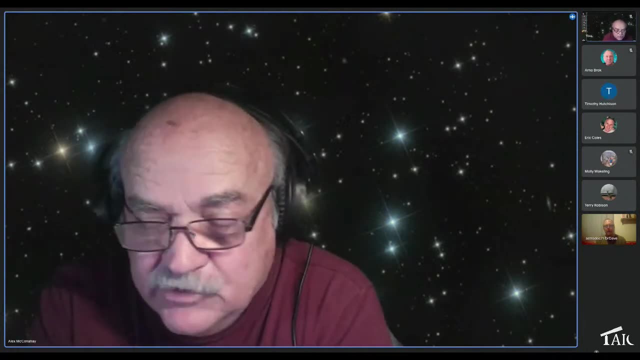 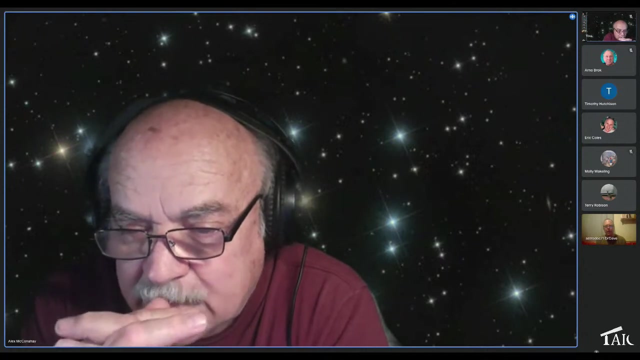 that it looks like the telescope focal length may not really be an issue when performing this type of astronomy. and then, later on, pam and jeff, who are already planning a consortium to take on the high-res spectroscopy. here pam says that, uh, she might need to wait for a bigger scope, though tell us about the you know. 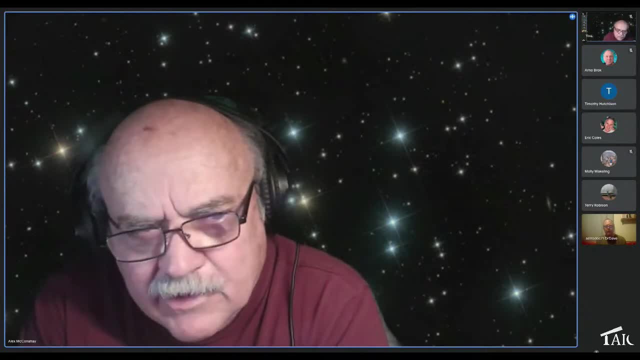 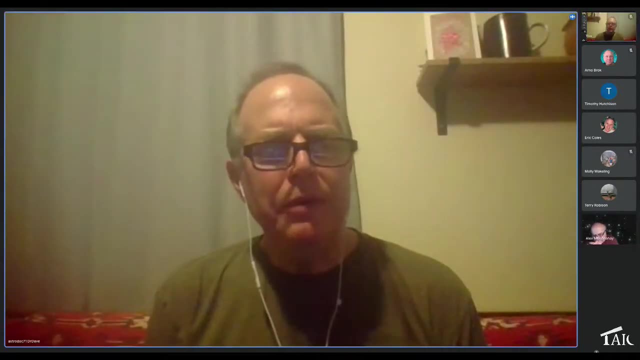 what kind of scopes we need, uh, what the implications are and that stuff. i think you touched on it, but tell us again: yeah, okay, so, uh, yeah. so you basically need to uh to match the, uh, so the, the, the spectrograph has uh as as a, uh, the folded uh focal length is f10 and uh, and you want to match that more than the other premiums. 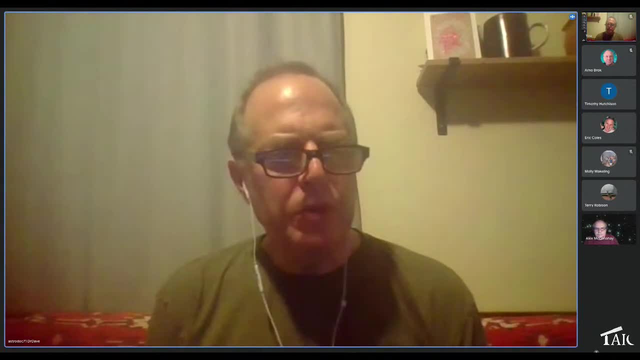 less with your, with your telescope, uh optics. so you want to be within that f8 to f12 uh region. but but but you don't, i mean you. you could like, if you have a f5 or something like that, you could technically you could use a barlow to uh. i'm not really sure how that, how that works, though, with 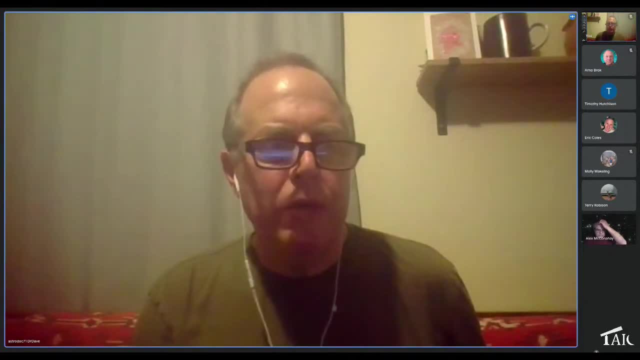 with your cameras, etc. but i know that that people do that or can do that. um, in terms of aperture, um, you know, your, your stars are, are, you know they're pretty bright, you know, uh, so, um, you're probably not going to. i mean, i think you're still going to be able to see to the, to the magnitude. 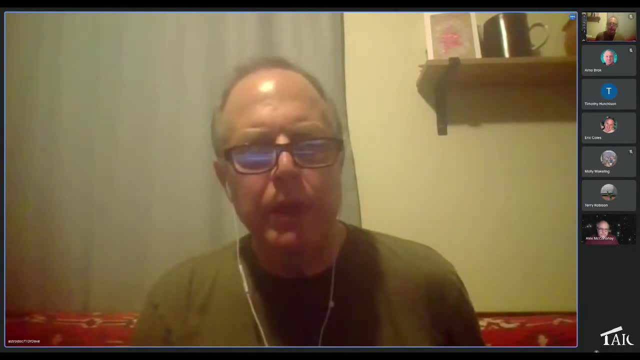 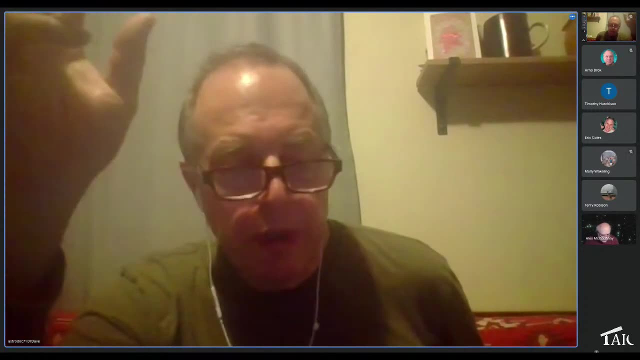 limits. your resolution might be affected though, uh, depending and that, and that depends on also the, the slit width. um, it's a little more technical because there are different size slit widths and you might have to match them. uh, you know, with the, with the uh, uh, with the telescope that you're using, typically a 23. 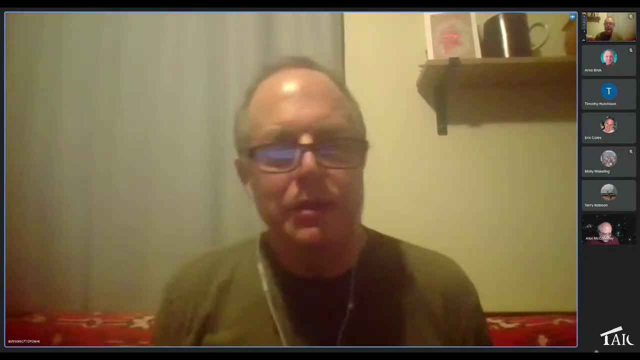 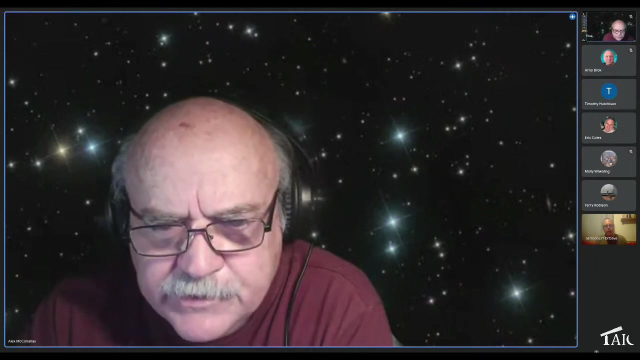 micron will work with, i think, just about anything, just about anything. so you could use a c8, you could use a, uh, a c11, you could use a, you know a refractor, even um. okay, you, you've been speaking of focal lengths or not, not focal lengths. you've been speaking of f ratios, um, and that can vary. 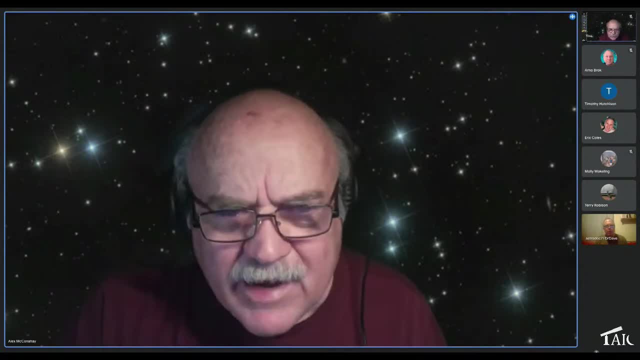 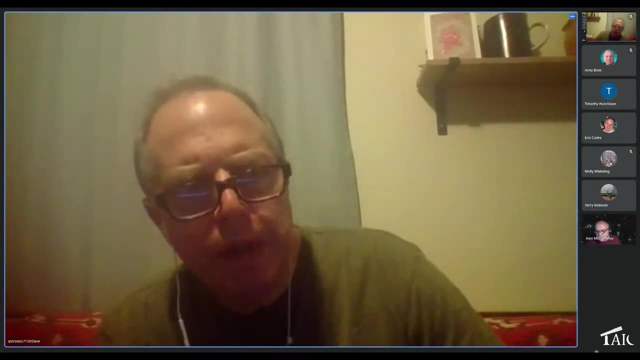 dramatically according to your aperture. what kind of aperture do you need on these things? um, i, i don't, i don't think that the aperture is uh, um, you know, is a limiting, uh, you know, for for high res. i, i think, well, i, i would say, just from what i've seen, uh, probably eight inch would be. 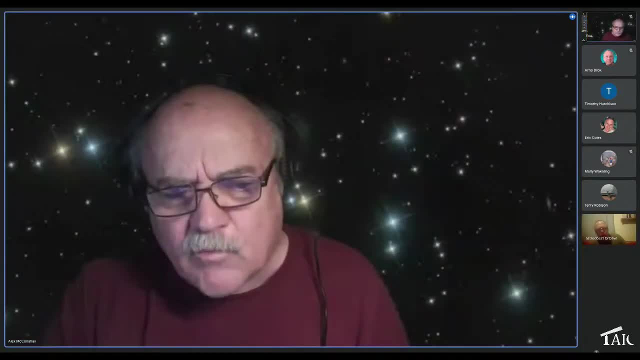 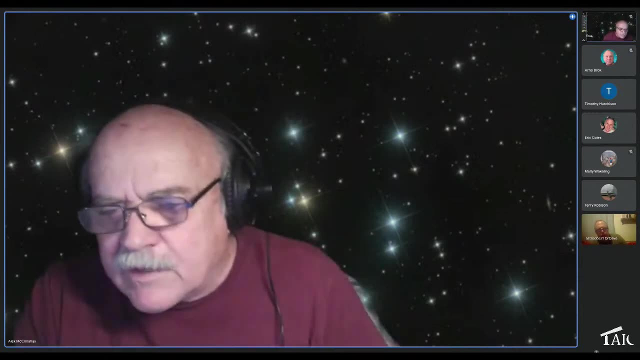 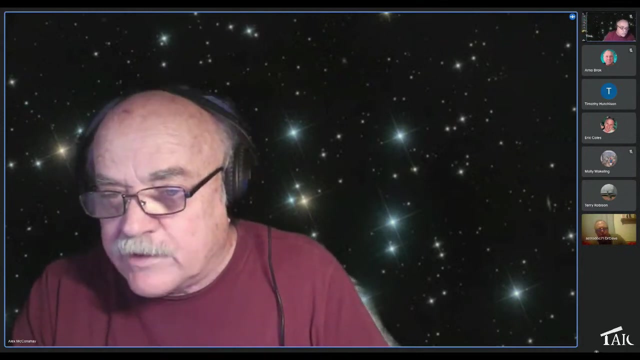 your, you'd go for one other, you'd go find somebody's used celestron c8, yeah, and, and take it to go from there, okay, okay, um, don and paul and elizabeth romero and i guess everybody else in the whole room there with them. do we need to use any? you know? non-anti-blooming camera, mono cameras- what kind? 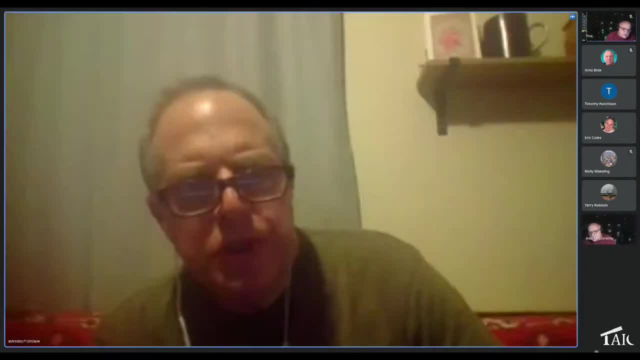 of tech cameras do you use, uh, you use c, you use uh. well, i have an attic 460 ex. so i believe that is, uh, i don't. i think there is, um, i don't think that's any- that's non-anti-blooming camera. 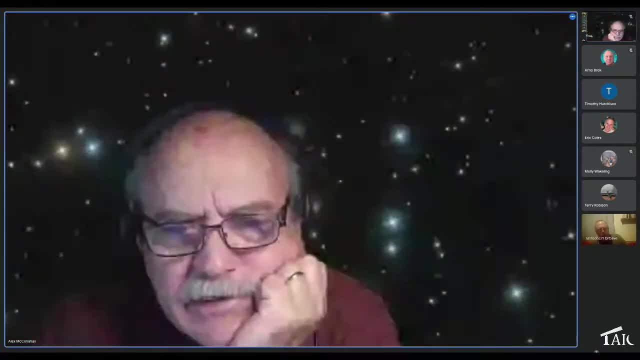 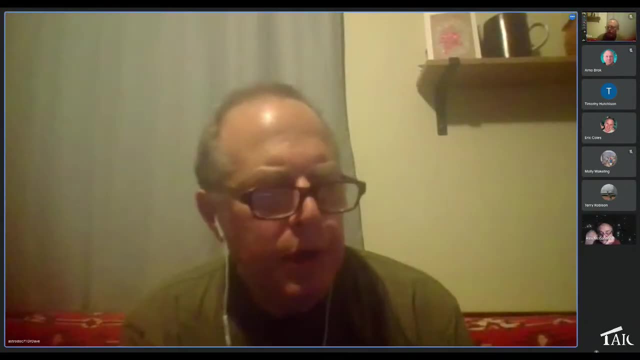 i don't think so, and i suppose it has to be somewhat linear. yes, yeah, so i don't, i don't know. uh, i think everybody that i that i've seen is still using ccd. i don't know about um, about cmos, um, i think ccd is still preferred. 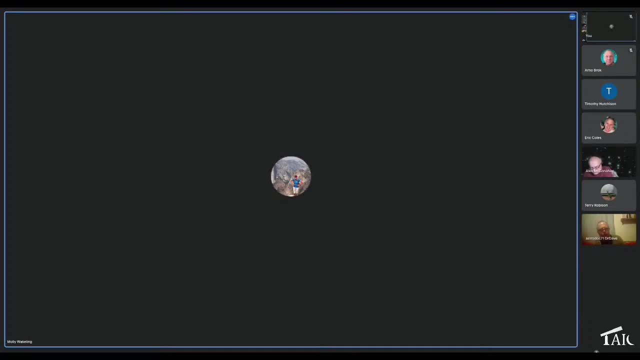 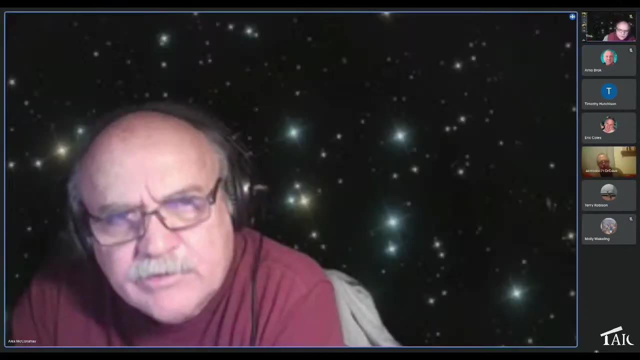 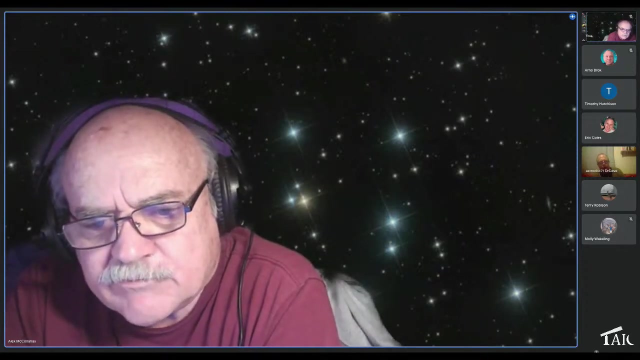 okay, probably because of the linearity, yes, but it wouldn't take a brand new, hottest off the market ccd. it just takes something big enough chip to see the to see the results. right, right, right, dave, can i ask a question? yeah, i see, you've got. 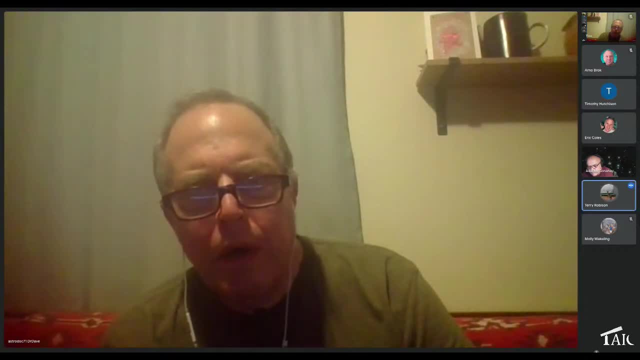 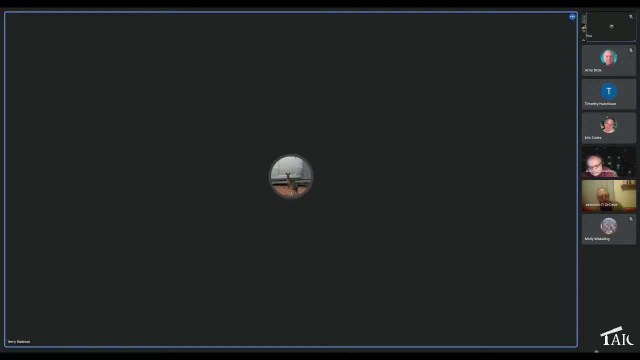 you have a reasonable amount in your photograph there. how do you find and verify the star of interest? are you looking through the slit while doing this, or is there a way to see the full background of stars and plate solve? uh, you, you can. uh, definitely plate solve. 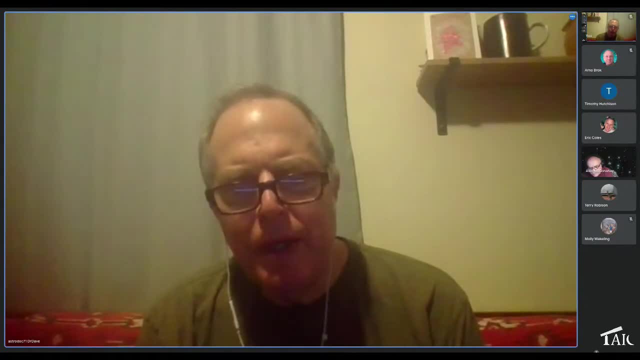 um and uh, there are a lot of people doing that, but, um, but, if you're, if you're looking at at stars, you know, i, i, i, i haven't imaged the wrong star yet and and i've been, do i, i've done this manually. i don't plate solve, um, i kind of uh, uh, i, if i have to, if i'm 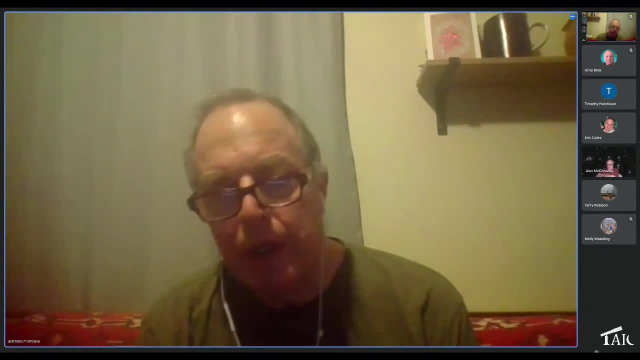 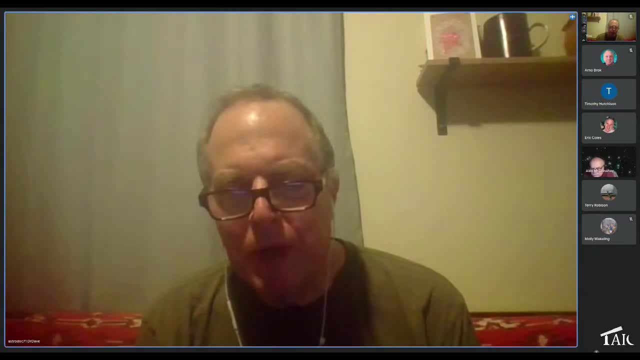 you know my fov and my planetarium program, to say, okay, that's the pattern of stars and this is the star that that, uh, that it should be. and the other thing is, if you're, let's say, you're- imaging a, a, b, emission star, well, you're going to, you're going to want to see an emission. 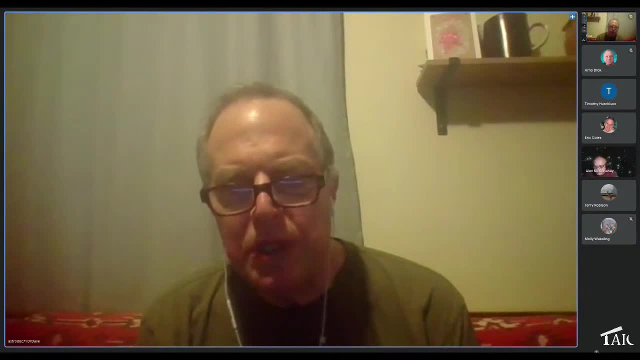 spectrum. you're going to take a test image and if you don't see a mission, uh, in the hydrogen alpha line, then you might think, gee, i wonder if, uh, maybe i don't have the right star. so there are things like that that can give you clues, uh, to avoid that mistake. but 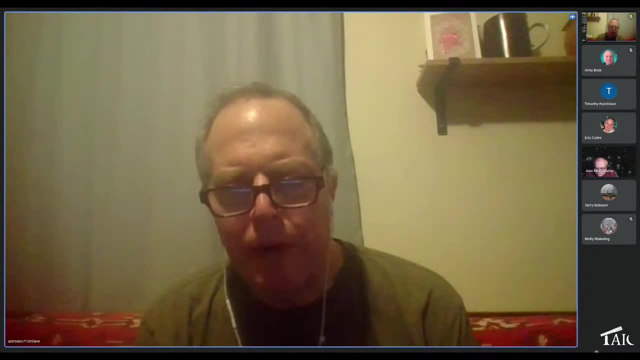 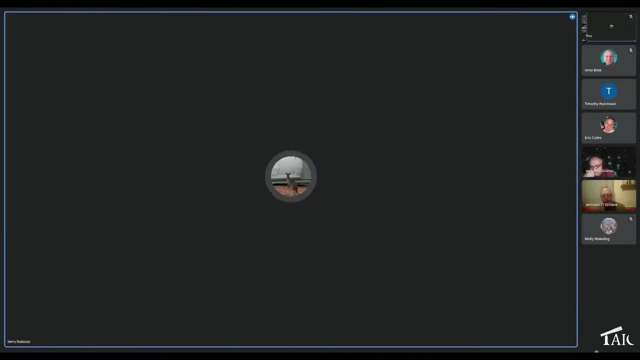 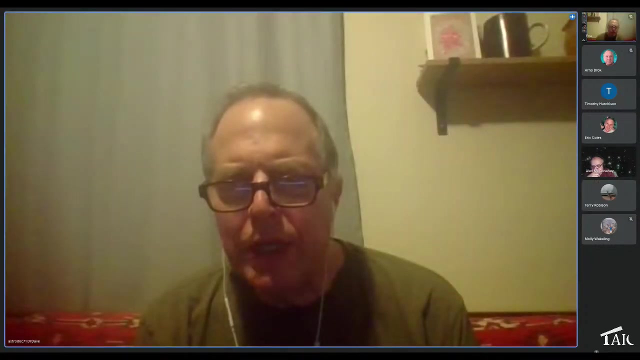 typically, the star that you're looking at is going to be a lot brighter than the surroundings in the background in your field and you do all this initial uh setting up your scope through the slit and you can use the light, of the light you're getting with your light to hit thestars as well. 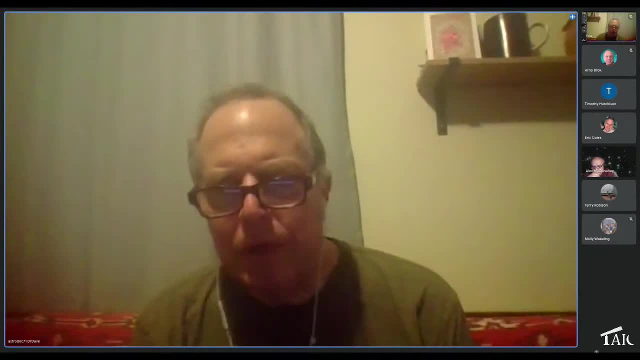 yes, did you say again. yeah, sorry, say again, uh, um, this initial, i guess finding the star here. you're doing this through the slit. no, no, your your guide camera. um, uh, because you know that the light that goes through the slit is not going to help you in any way other than i see. you know so. so the it's the, it's the light that's reflected off of the- uh, off of the slit, because the slit actually sits in the center of this mirror and the and the light is going to, is going to work out on the right side of the and the other way around. 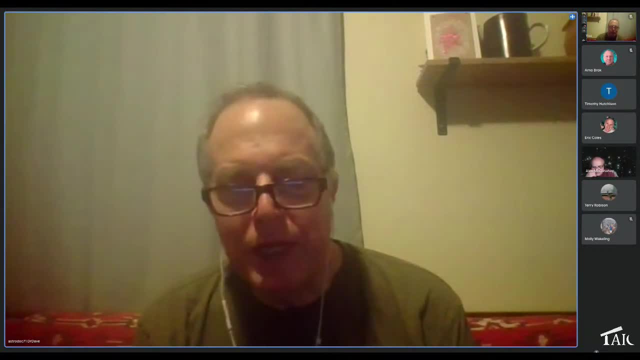 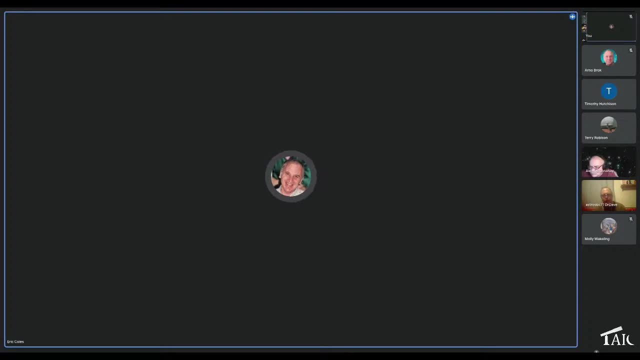 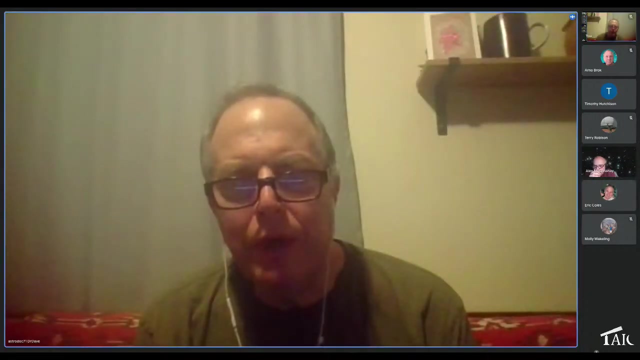 uh, go back uh into your guide camera, so that's how you're going to know where you are. okay, thank you. yeah, and actually jim said that he uses uh cmos cameras and they work just fine for this application. okay, well, yeah, that's great. i, i didn't really know, uh, anything about that to. 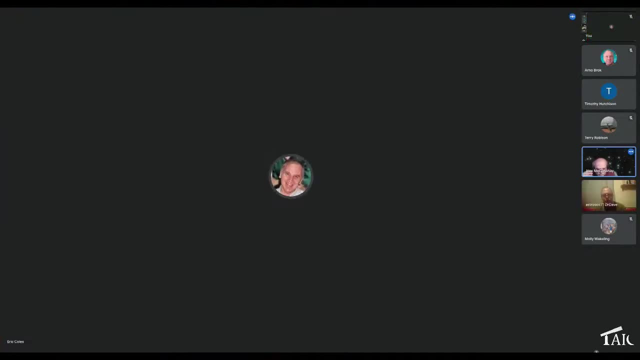 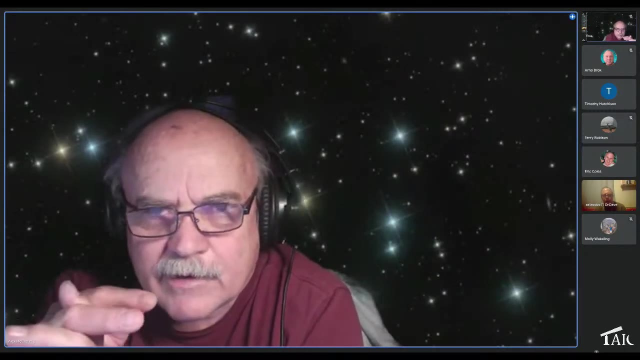 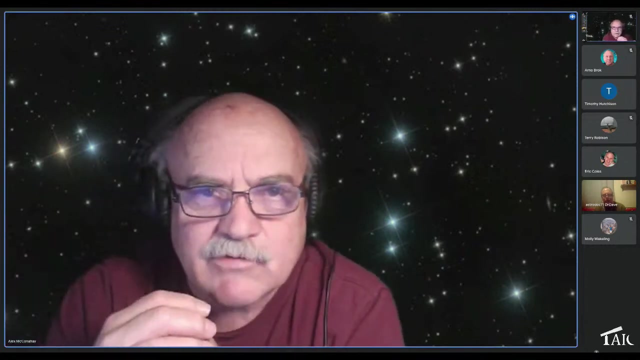 be to be honest, that would change your sensitivity probably. yeah, um, you know, i i guess i got an old story out of out of my past. um, i, in my club i was the junk dealer. whenever we got something donated to us that we needed to unload or something like that, i was often asked to do that. 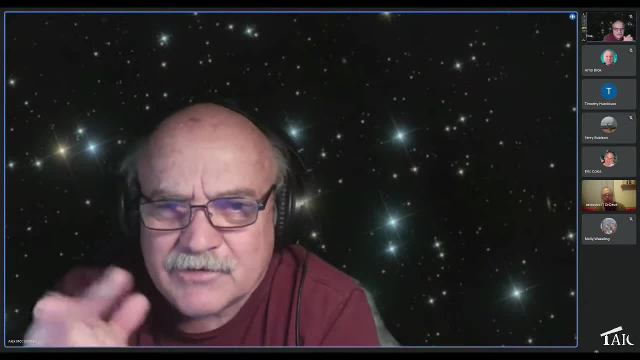 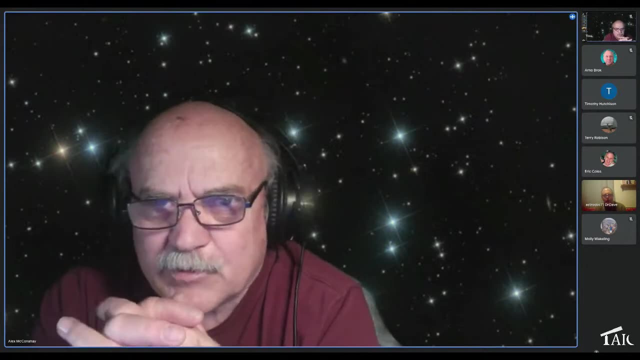 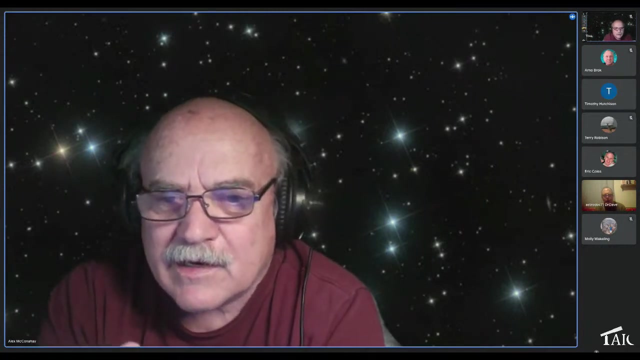 and one of the things i was asked to sell was, uh, either a c9 and a quarter or a c11 or something like that. and uh, i, when i was meeting up with the guy to sell it and i says, look, i can't guarantee any of this or that or the other thing, but i know it, it works pretty well and 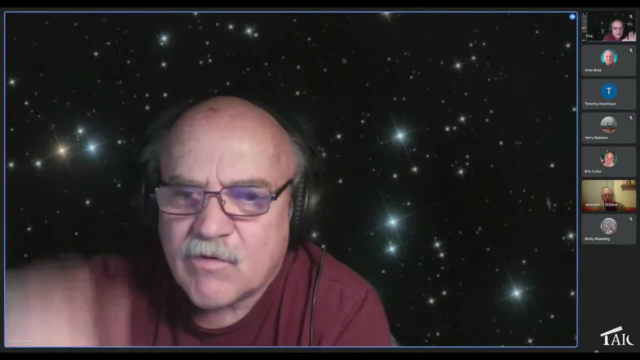 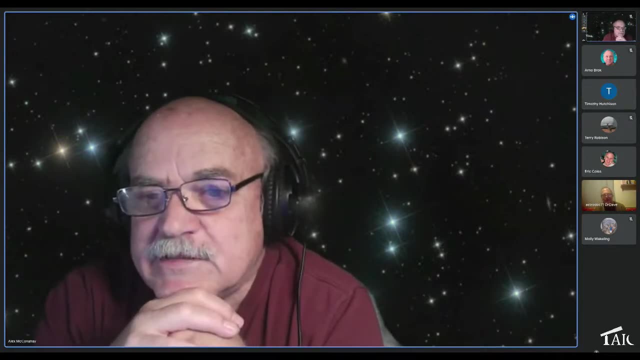 i. i don't know about pretty pictures or what it takes. he says: i don't worry about that, i'm doing scientific stuff, so i don't. i don't really have to push it, and that may be why so many people with ccds on the uh, attaching them to their, to their spectros. you know their things, their. 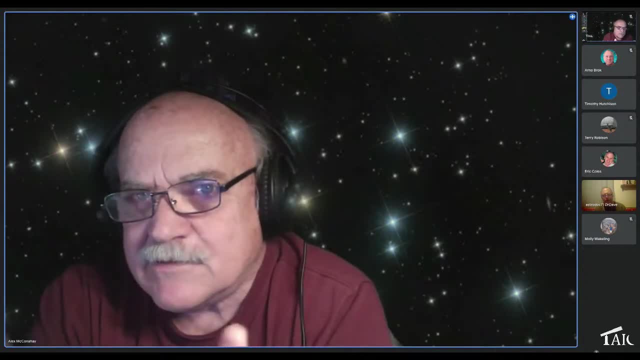 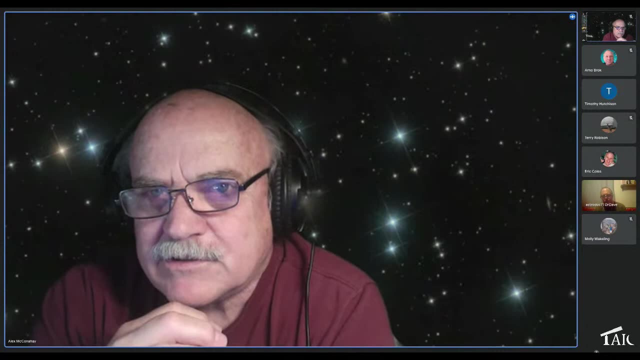 instruments there. um, that may be why it's because these do not take the highest, lowest noise. all the things that we look for when we're doing our pretty picture of astronomy is that you can get by with really decent, just good, old-fashioned pedestrian equipment. yeah, well, probably because 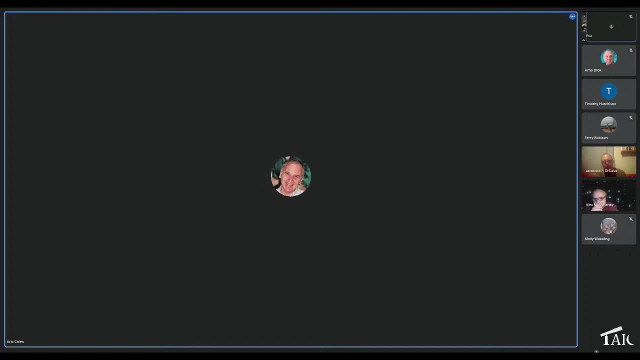 you're just looking at a single star in the center of your field, right? you're not worried about what's at the corners? yeah, it's true, i might have to put my c11 back in the service. i was gonna scts that we have in the telescope museums in our basements. 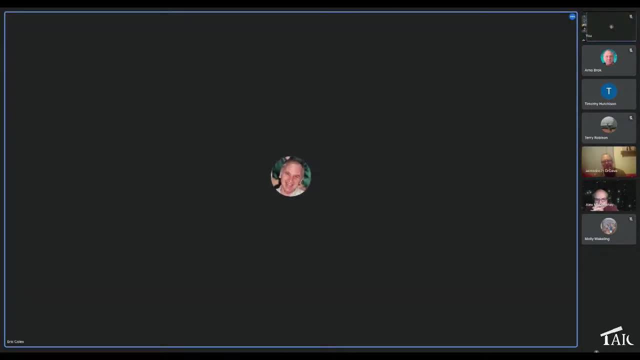 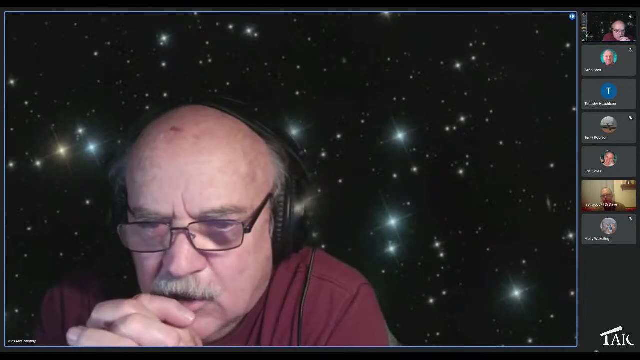 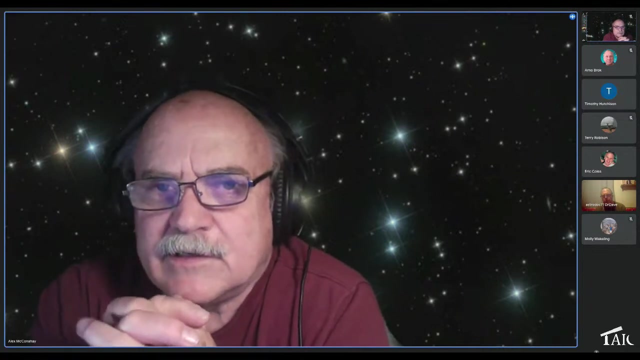 we can. we can take out for this kind of project. that's right. okay, i think we've got the questions, we've marked them all off, um, and i think we got them all in. we want to thank you very much for any introducing us to another world. uh, i think.